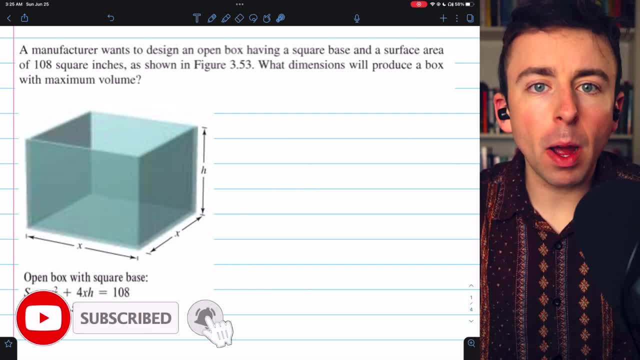 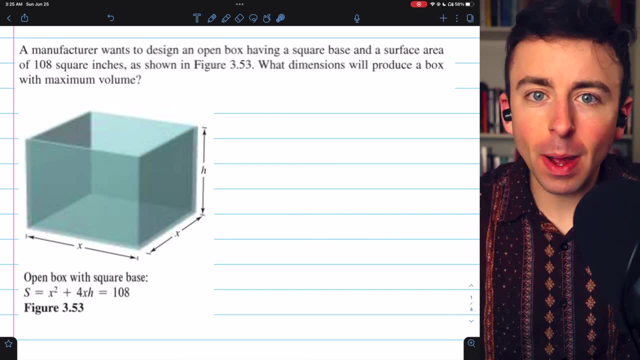 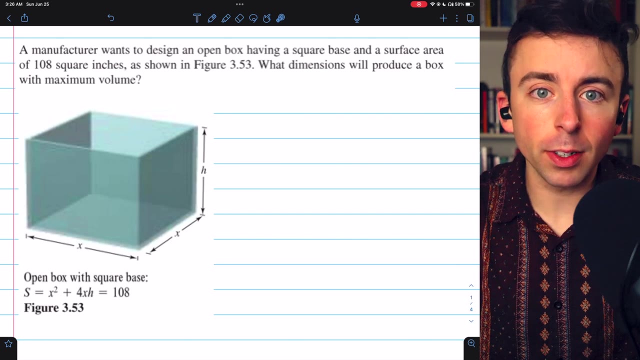 One of the major reasons we spent so much time talking about how to find maximums and minimums of functions is to solve optimization problems: Maximizing revenue, maximizing volume, minimizing surface area. this type of thing is really useful. I'm going to show you, step by step, how to solve. 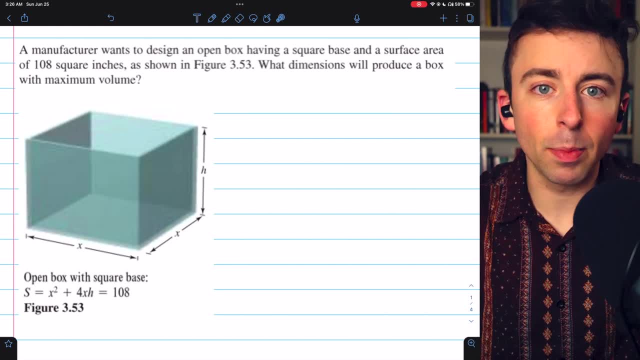 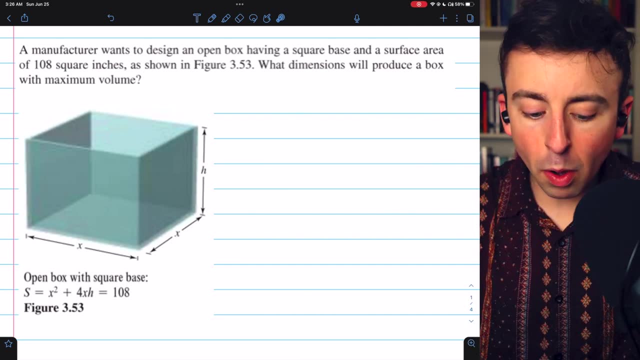 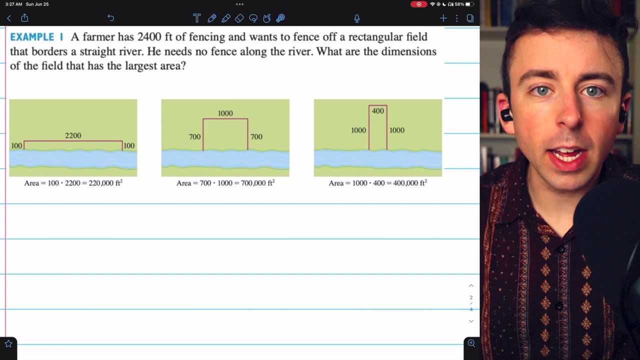 optimization problems, and today we'll do three examples. Chapters are in the description, if you want to skip around, as well as links to other practice exercises. In our first example, we will maximize the volume of an open top box. In our second example, we will maximize the area. 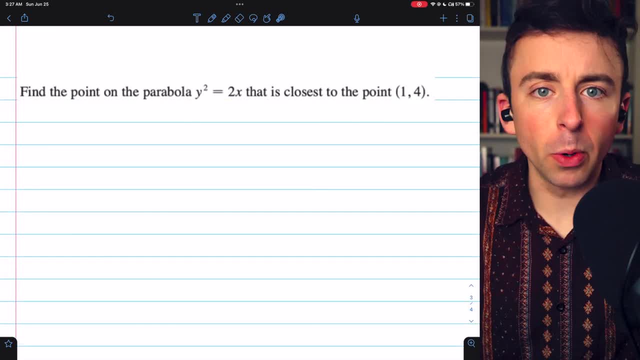 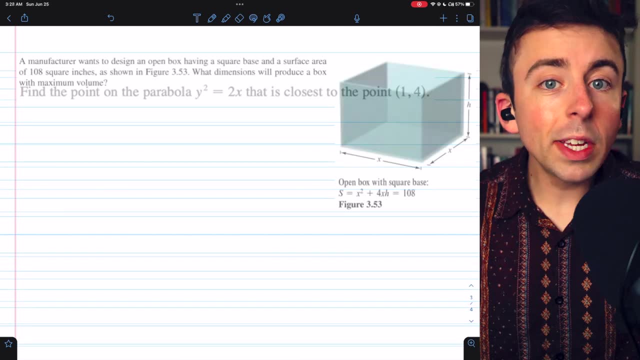 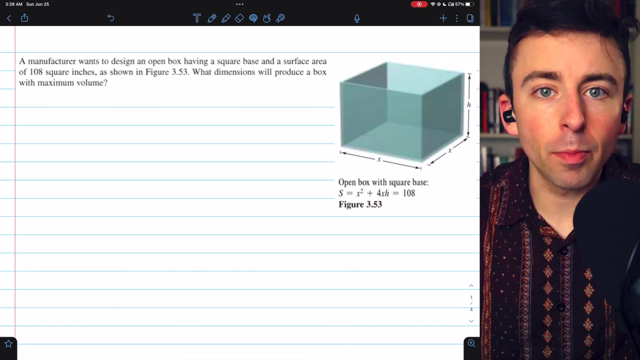 of a fenced off region. Our third example is the most difficult. We will find the point on a parabola that minimizes distance to a given point. We could do a thousand different optimization problems, but the good news is they all more or less follow the same problem. 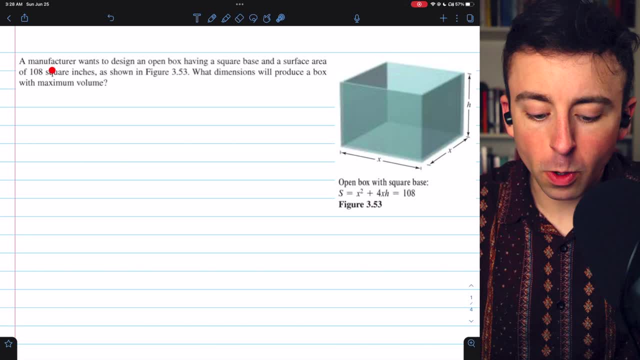 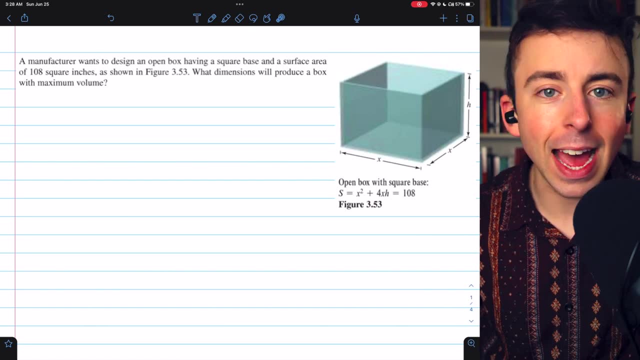 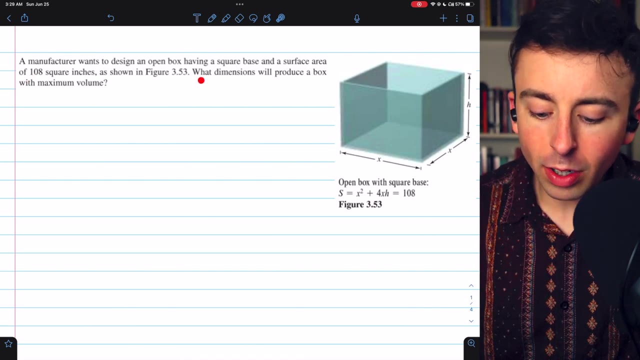 So that is the whole process. Let's begin with the first problem. A manufacturer wants to design an open box having a square base. so the dimensions of the base we could say are X by X, it's A square, and a surface area of 108 square inches, as we see in this figure What dimensions 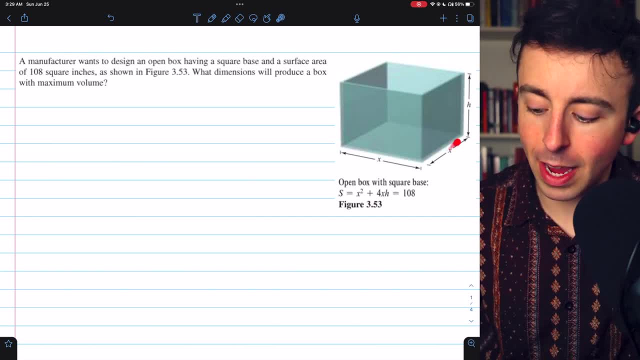 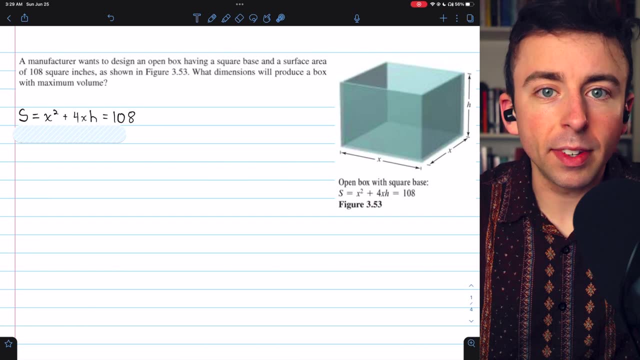 will produce a box with maximum volume. So our box is a square base that's X by X and we'll call its height H. It has no top solving. an optimization problem is to make a sketch, if we can. In this case we already have. 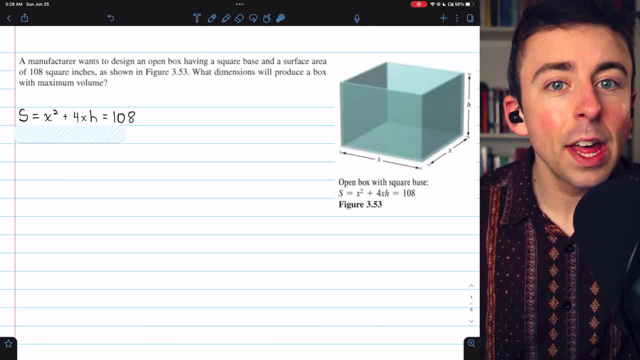 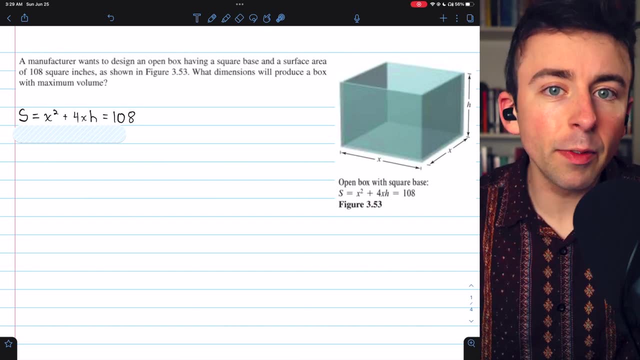 a figure to use so we don't have to do any sketching. Then we want to make sure we understand what quantities are given and what quantities we might need to figure out. In this case we're given the surface area- and this is pretty common in an optimization problem that you'll be given some. 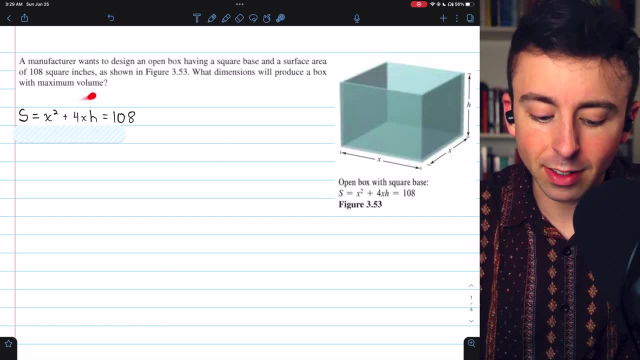 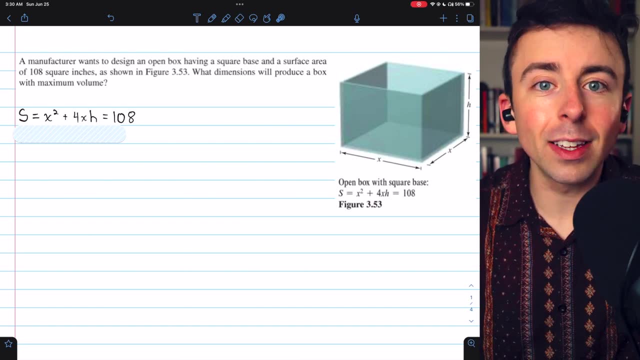 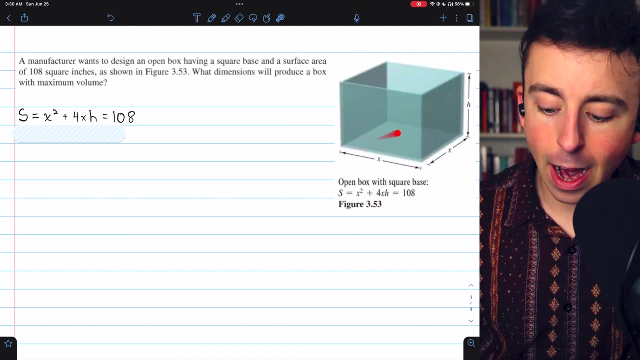 sort of restriction. In this case we're trying to maximize the volume, given the restriction that we need a surface area of 108 square inches. Since we're given the surface area, we want to write an equation for that quantity. Our surface area is x squared the area of the base plus the areas of. 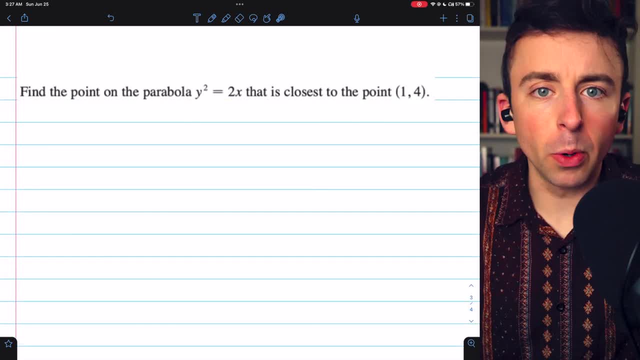 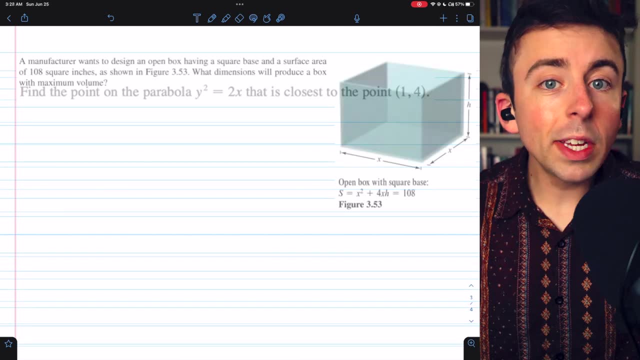 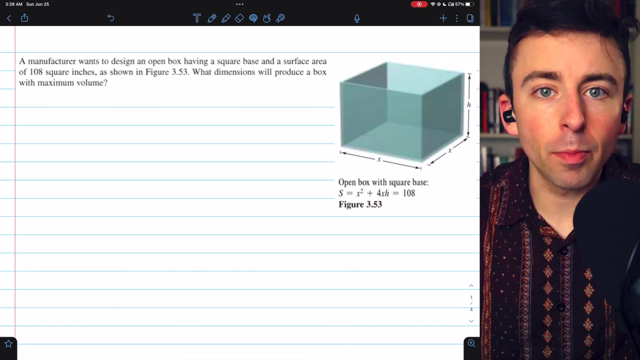 of a fenced off region. Our third example is the most difficult. We will find the point on a parabola that minimizes distance to a given point. We could do a thousand different optimization problems, but the good news is they all more or less follow the same problem. 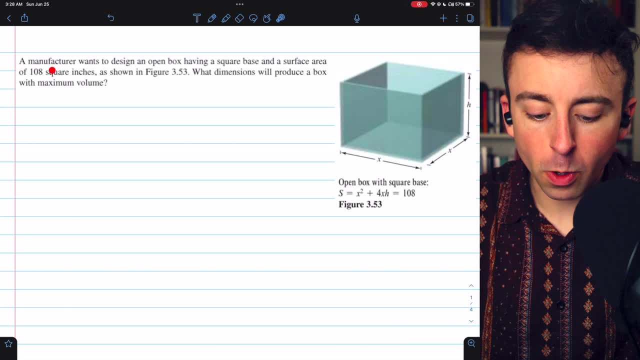 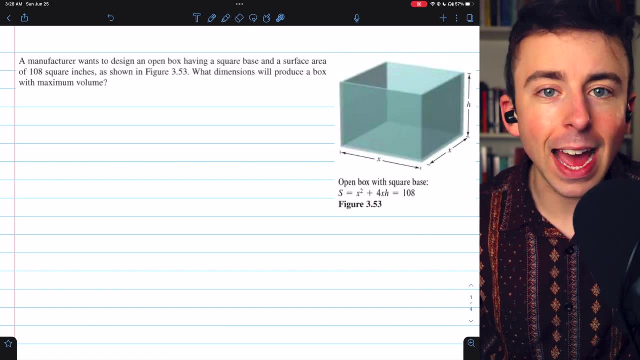 Let's see the process. Let's begin with our first problem. A manufacturer wants to design an open box having a square base. so the dimensions of the base we could say are X by X- it's a square- and a surface area of 108 square inches, as we see in this figure. 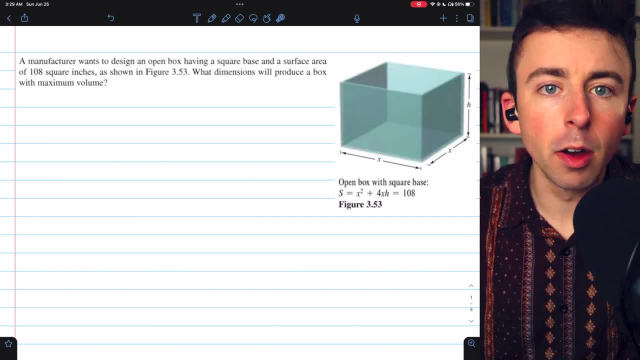 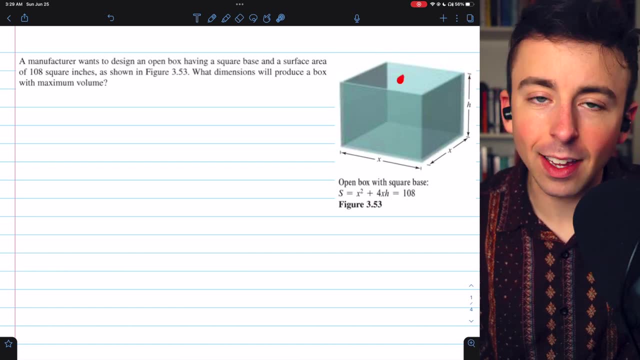 What dimensions will produce a box with maximum volume? So our box has a square base that's X by X and we'll call its height H And remember it has no top. Our first step is to zoom in on the top box and make sure that the bottom box is placed at 100.. 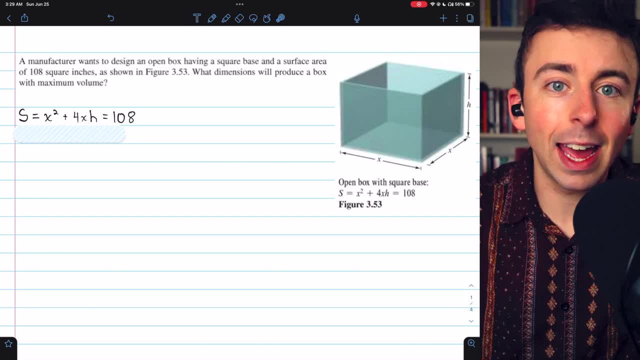 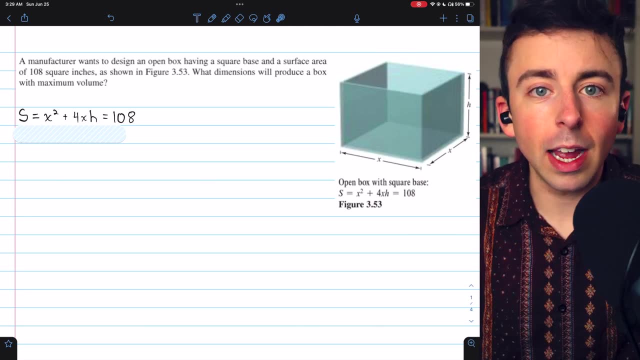 in solving an optimization problem is to make a sketch, if we can. In this case we already have a figure to use, so we don't have to do any sketching. Then we want to make sure we understand what quantities are given and what quantities we might. 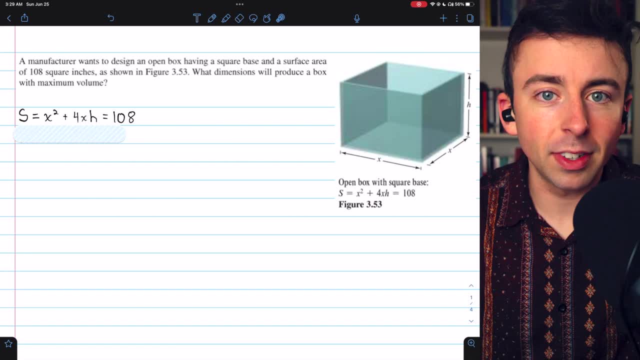 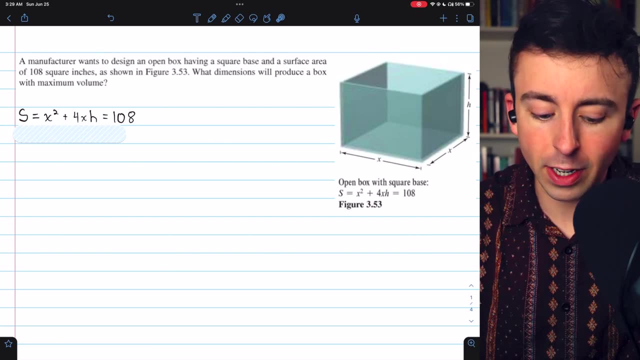 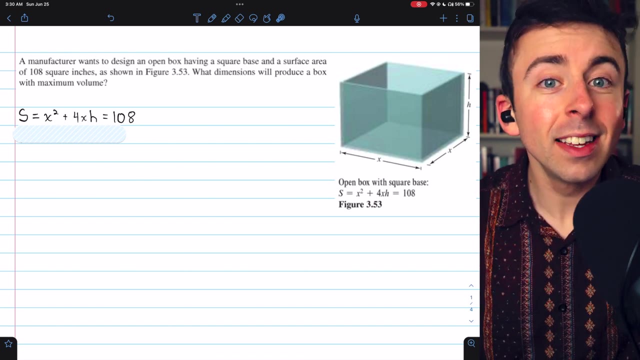 need to figure out. In this case, we're given the surface area- and this is pretty common in an optimization problem- that you'll be given some sort of restriction. In this case, we're trying to maximize the volume, given the restriction that we need a surface area of 108 square inches. Since we're given 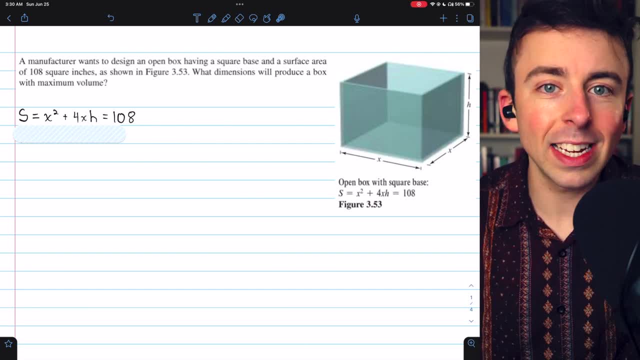 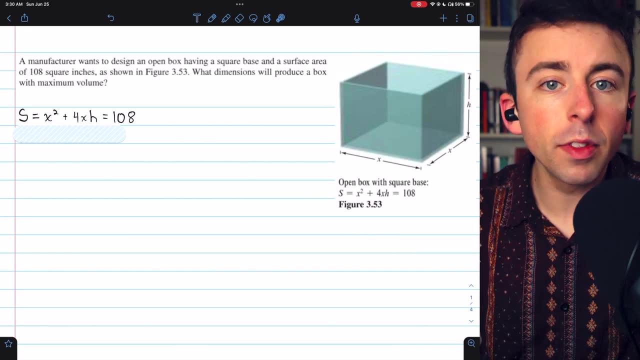 the surface area. we want to write an equation for that quantity. Our surface area is x squared the area of the base plus the areas of the four sides. Each side has an area of x by h and there's one, two, three, four sides. So x squared. 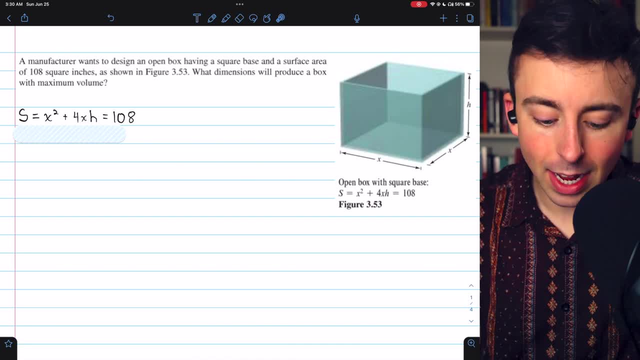 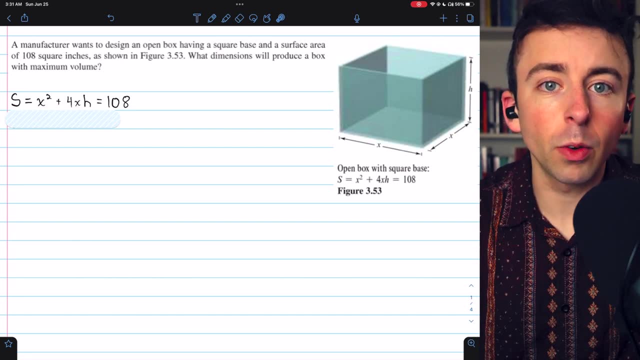 plus 4xh is the surface area, and we're given that this has to equal 1.5x. This is called a secondary equation, because it's an equation for something that we're not trying to optimize, The equation for what we're. 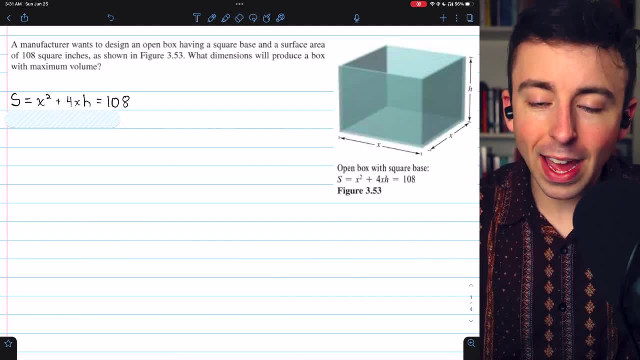 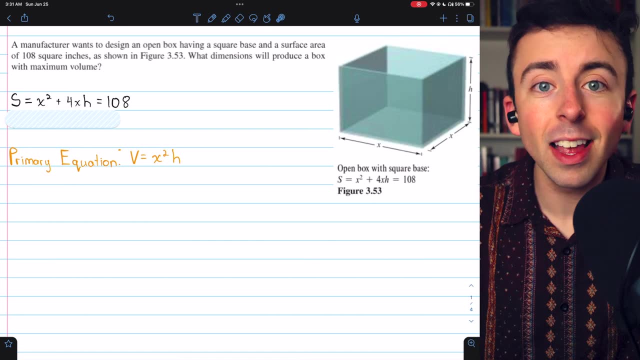 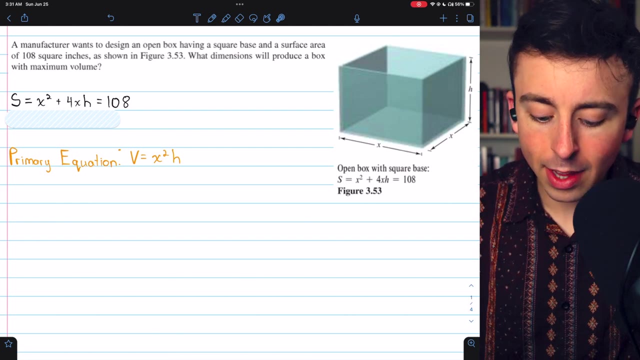 trying to optimize is called the primary equation, and that's our second step. We want to write a primary equation, the equation for the quantity we're trying to optimize. In this case we're trying to maximize volume. so our primary equation is an equation for volume. That's the area of the base x squared multiplied by 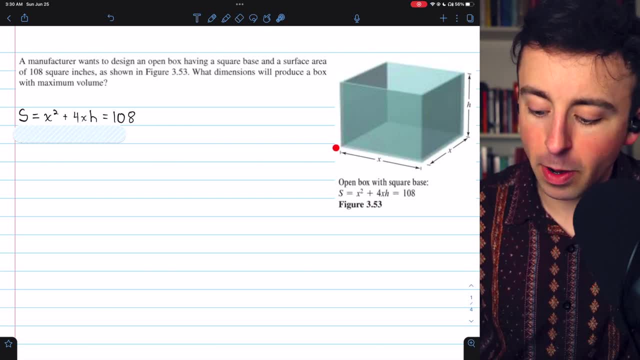 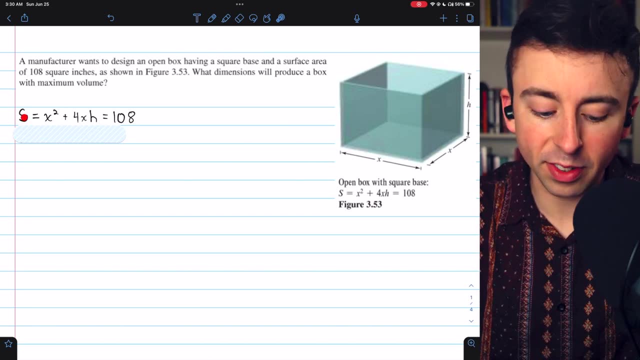 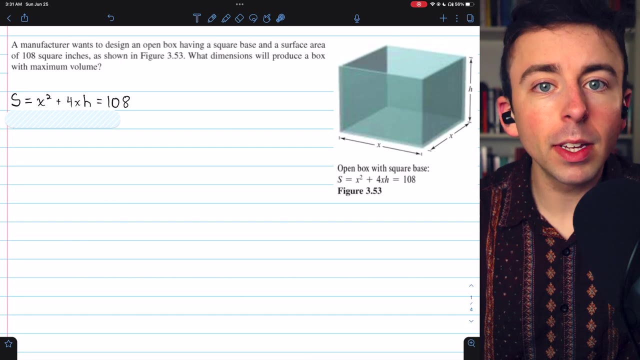 the four sides. Each side has an area of x by h and there's one, two, three, four sides. So x squared plus 4xh is the surface area, and we're given that this has to equal 108.. This is called a secondary equation, because it's an equation for something that we're not trying. 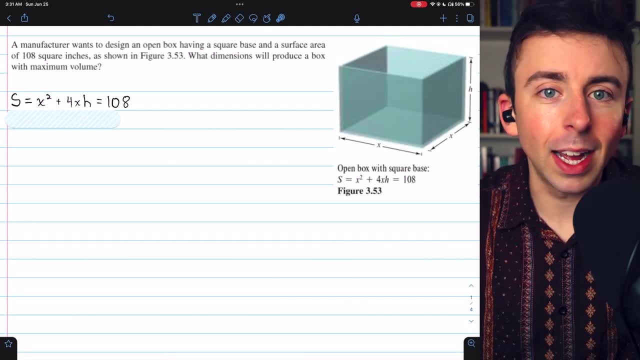 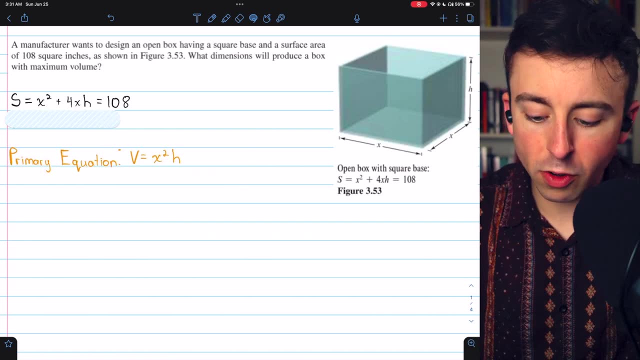 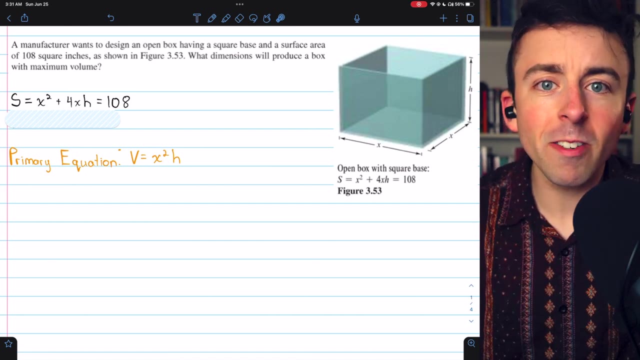 to optimize. The equation for what we're trying to optimize is called the primary equation, and that's our second step. We want to write a primary equation, the equation for the quantity we're trying to optimize. In this case, we're trying to maximize volume. So our primary equation. 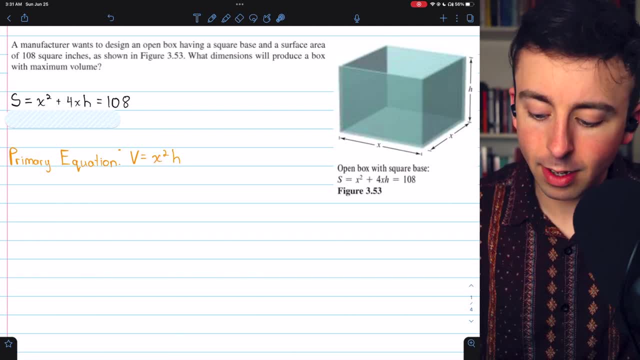 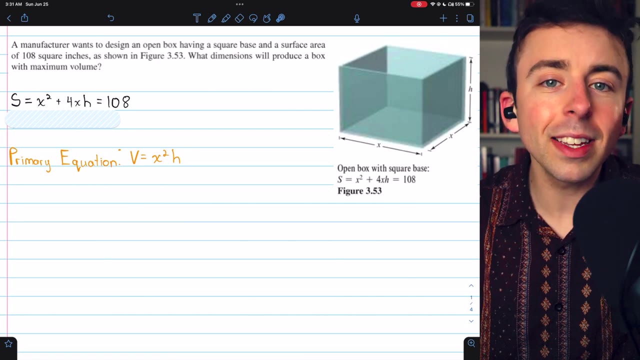 is an equation for volume, That's the area of the base x squared multiplied by the height, which is h. But we've encountered a problem because this primary equation has two variables. In order to use our calculus techniques, we need this equation to be in terms of a single independent variable. 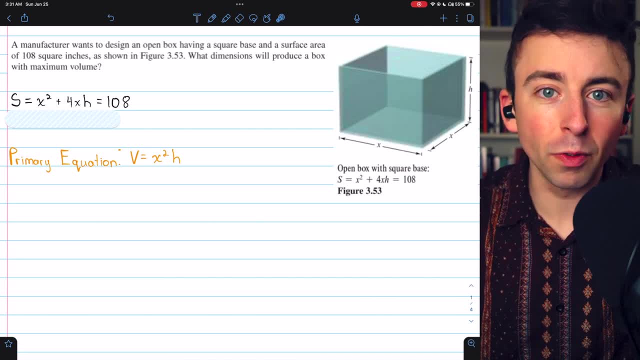 But that's where the secondary equations are often useful. This equation for surface area gives us a way that x and h relate. So if we solve this equation for either x or h- just pick whichever one is easiest- we'll be able to use the equation for the area of the base x squared. 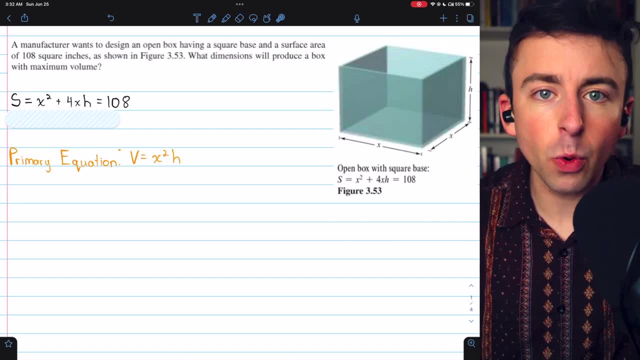 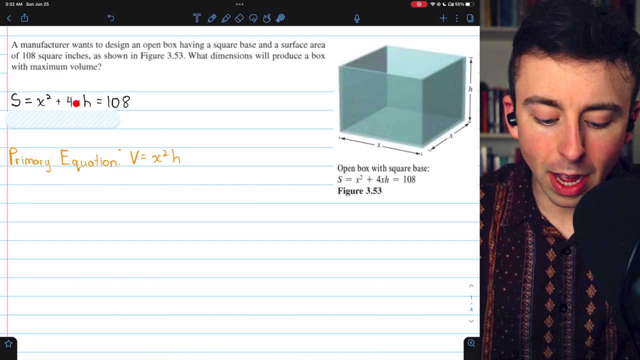 We'll be able to use that to rewrite the primary equation in terms of a single variable. And that's the next step. It will be easier to solve this equation for h than it will be for x, So let's solve for h. To do that, we just subtract x squared from both sides and then divide both. 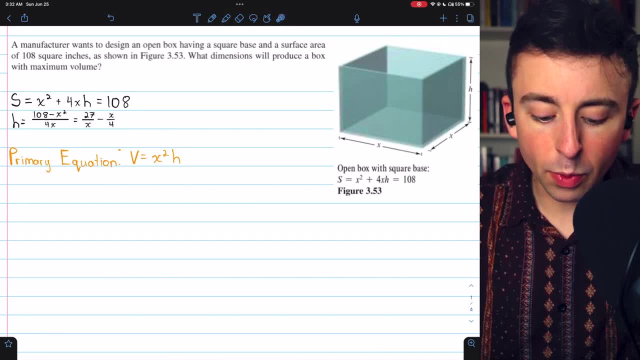 sides by 4x. And that gets us here. When we subtract x squared, we get 108 minus x squared. And then when we divide everything by 4x, it becomes 108 minus x squared divided by 4x. And then we just have h on the left side. 108 divided by 4x is 27 divided by x And x squared. 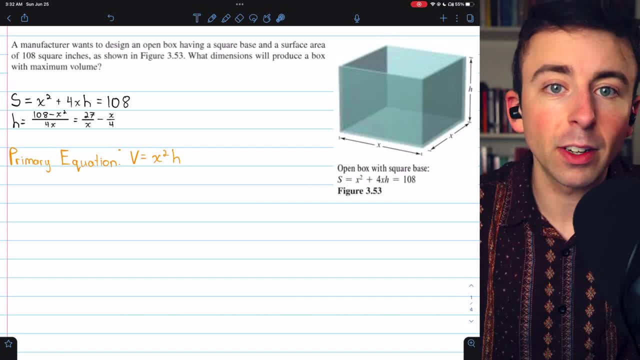 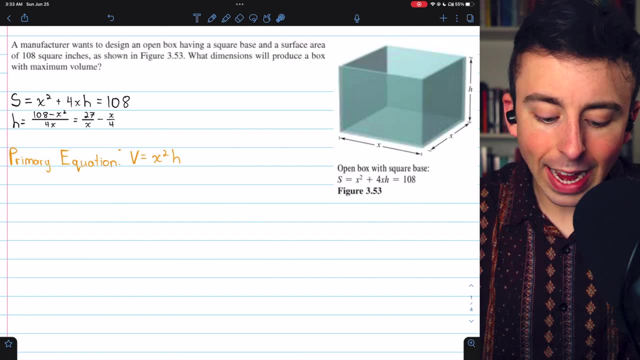 over 4x is just x over 4, because a factor of x cancels out And, don't forget, we have that negative. So by solving for h and doing a little simplifying, we find that h equals 27 over x, minus x over 4.. 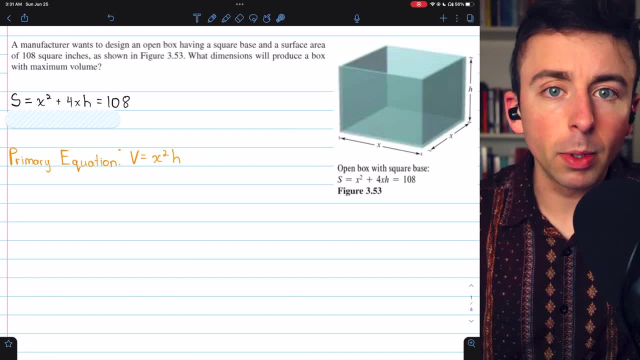 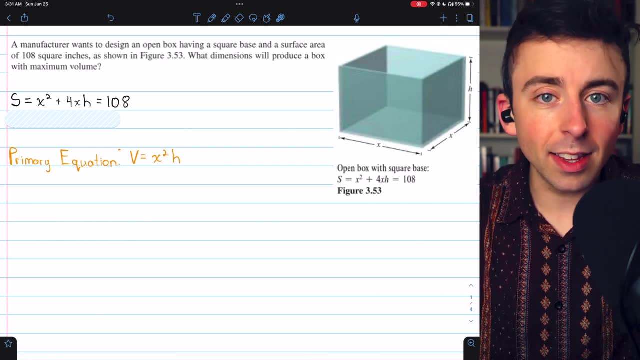 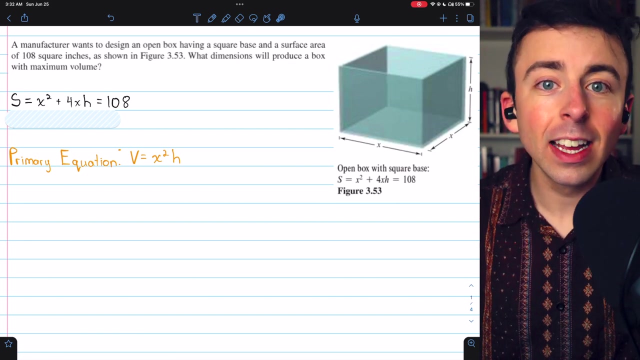 the height, which is h. But we've encountered a problem because this primary equation has two variables. In order to use our calculus techniques, we need this equation to be in terms of a single independent variable, But that's where the secondary equations are often useful. This equation for surface area gives us a way that x and h relate. So if 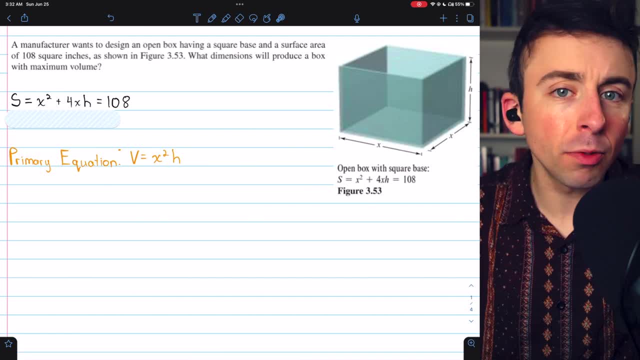 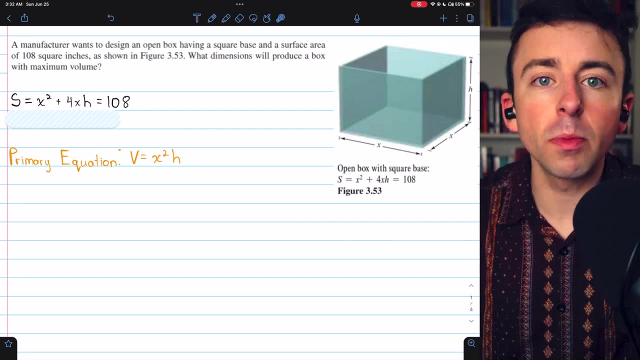 we solve this equation for either x or h. just pick whichever one is easier. we're going to be able to use the primary equation to rewrite it in terms of a single independent variable, And that's the next step. It will be easier to solve this equation for h than it will be for x, so let's solve for. 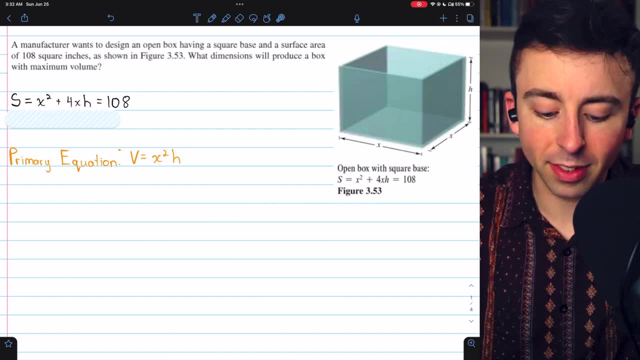 h. To do that, we just subtract x squared from both sides and then divide both sides by 4x. And that gets us here: When we subtract x squared, we get 108 minus x squared. And then, when we divide everything by 4x, it becomes 108 minus 6.. 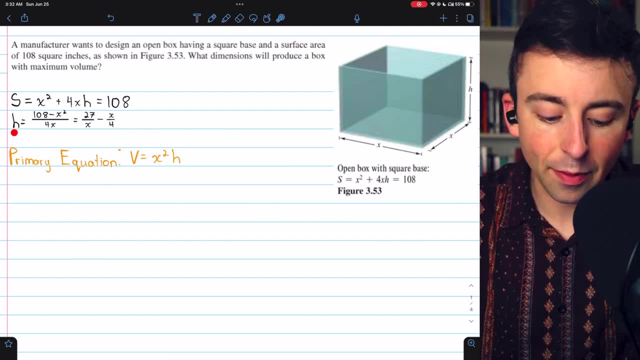 minus x squared divided by 4x. and then we just have h on the left side: 108 divided by 4x is 27 divided by x, and x squared over 4x is just x over 4, because a factor of x cancels out. and don't forget, we have that negative. 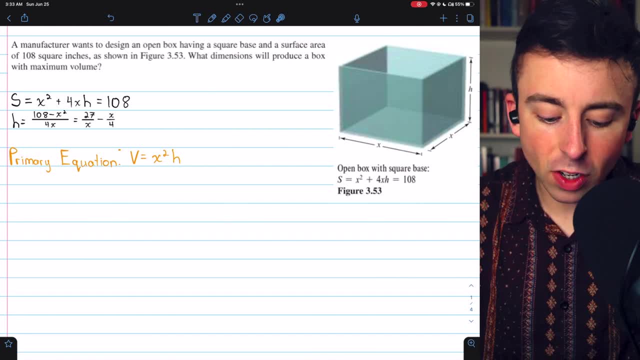 So by solving for h and doing a little simplifying, we find that h equals 27 over x minus x over 4. Plugging that in for h in our primary equation, we can rewrite it in terms of a single variable and use our calculus techniques. 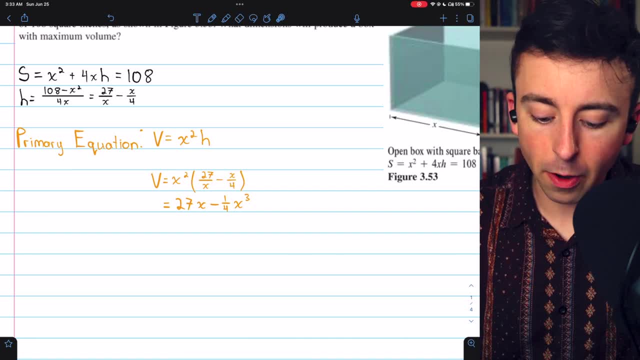 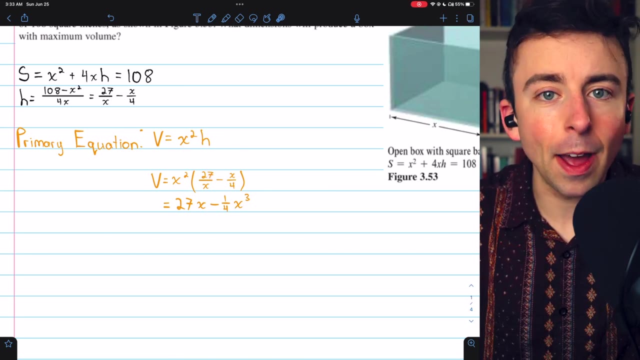 And that brings us here. The volume is equal to x squared multiplied by h, which we found is 27 over x minus x over 4.. Distributing the x squared through the parentheses, we have that the volume equals 27 times x minus 1. fourth times x cubed. 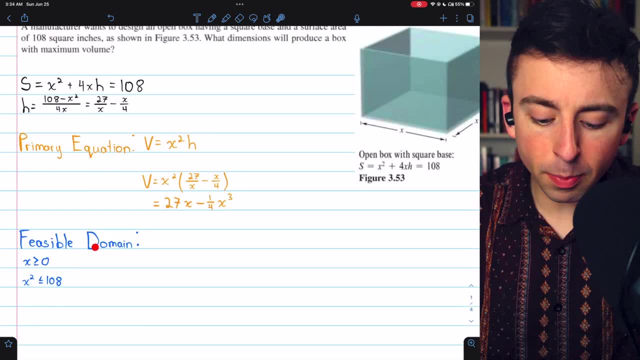 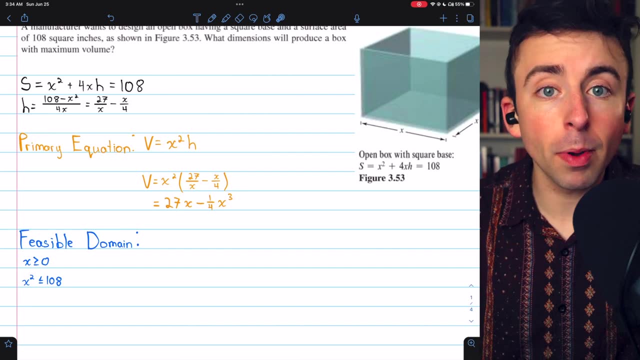 We're almost done. The fourth step is to determine The feasible domain for our primary equation that we figured out in the previous step. What values for x are possible? Well, we know that x has to be at least zero. We're not going to have negative distances for our box. 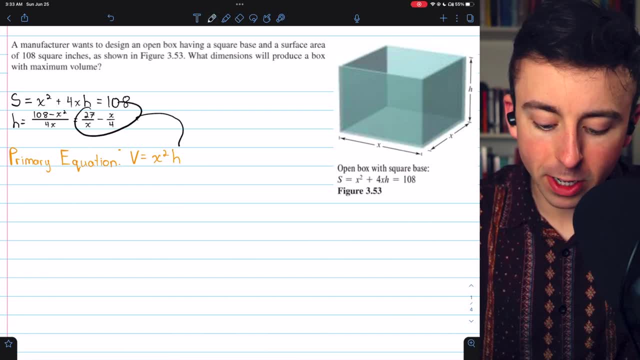 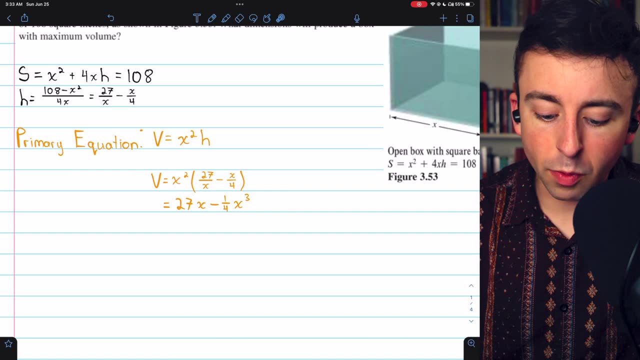 By plugging that in for h in our primary equation. we can write it in terms of a single variable and use our calculus techniques. And that brings us here. The volume is equal to x squared multiplied by h, which we found is 27 over x minus x over 4.. Distributing the x squared through the parentheses, we have that the volume. 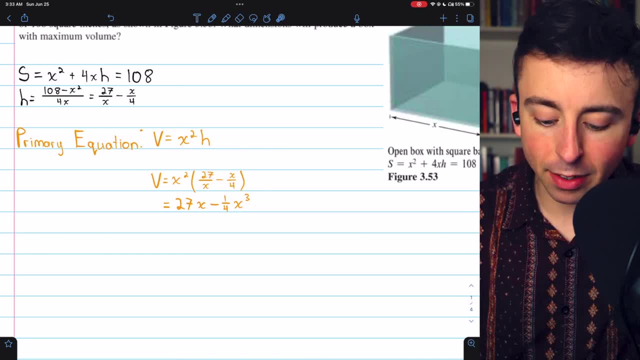 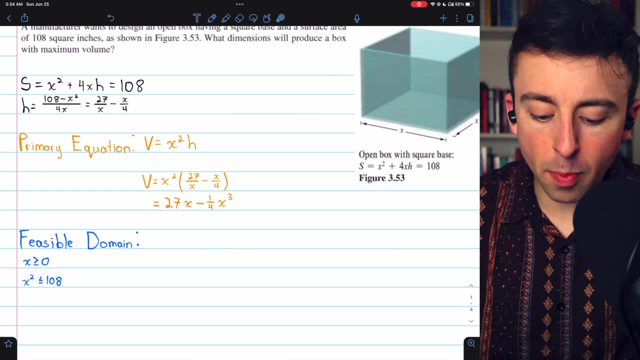 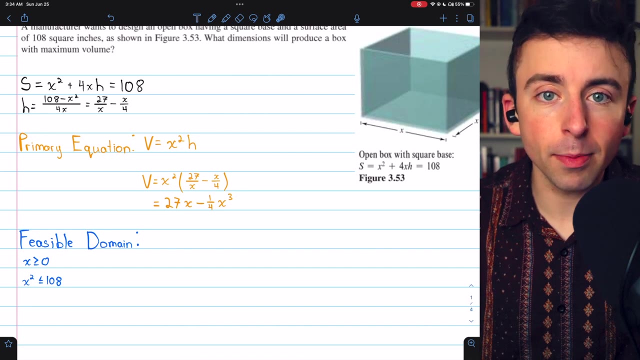 equals 27 times x minus one. fourth times x, cubed. We're almost done. The fourth step is to determine the feasible domain for our primary equation that we figured out In the previous step. What values for x are possible? Well, we know that x has to be at. 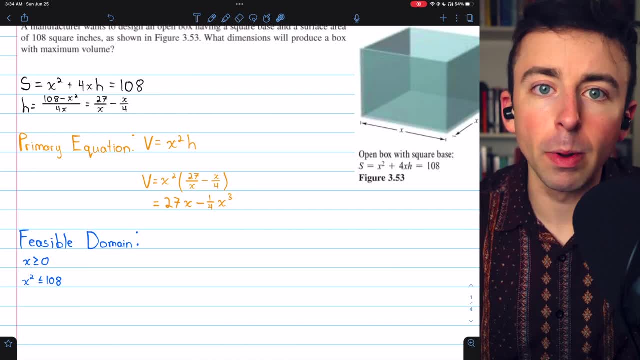 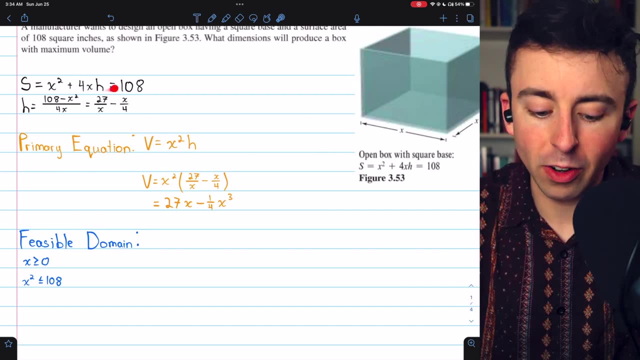 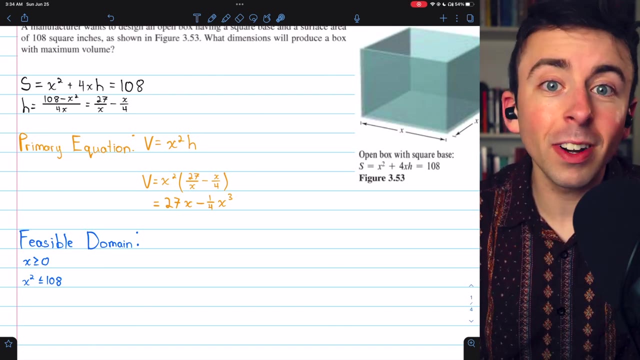 least zero. We're not gonna have negative distances for our box. We also know that x squared has to be less than or equal to 108 by the surface area equation. x squared is in this equation and the surface area equals 108.. So x squared certainly can't. 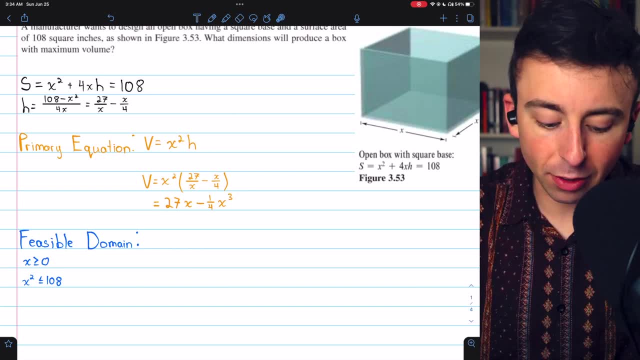 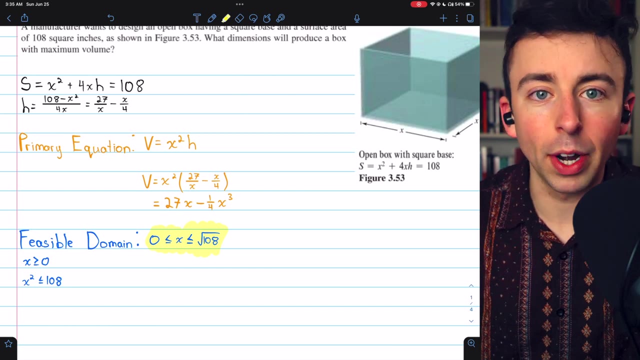 exceed that allowed surface area. x squared is less than or equal to 108.. that x is less than or equal to the square root of 108, and thus this is our feasible domain. x is greater than or equal to 0,. less than or equal to the square root of 108.. 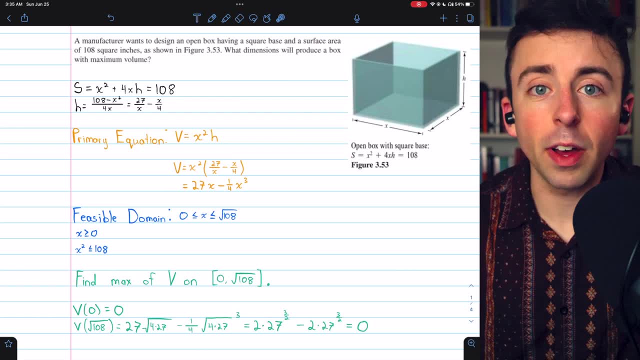 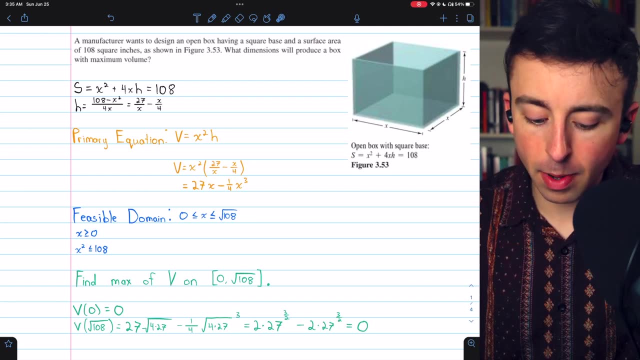 Then we're ready for the final step of using our calculus techniques to find minimums and maximums. In this case, of course, we're trying to find a maximum, and now we know that we're looking for a maximum of our volume v on this closed interval from 0 to the square root of 108,. 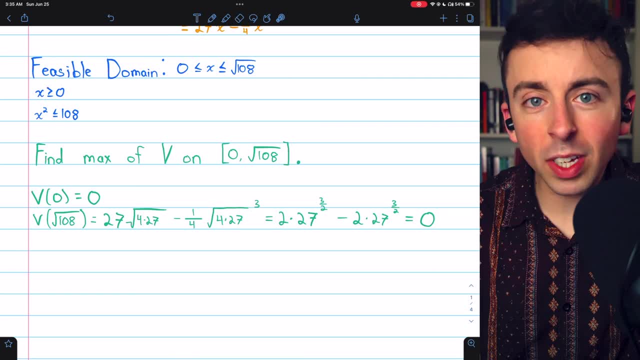 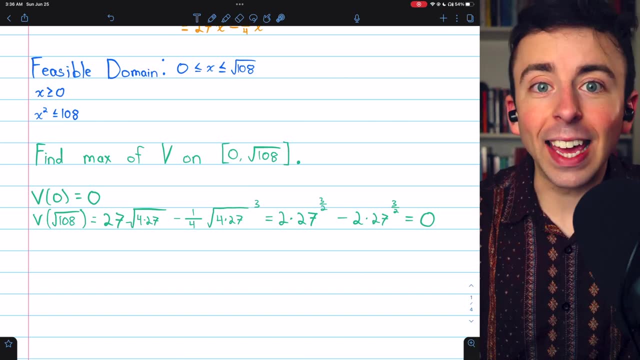 since that's the domain, Because we're on a closed interval, we're really using the extreme value theorem and the candidates test. We need to check the candidates for a maximum. The candidates are the endpoints of this domain, as well as any critical points. Let's begin by just plugging. 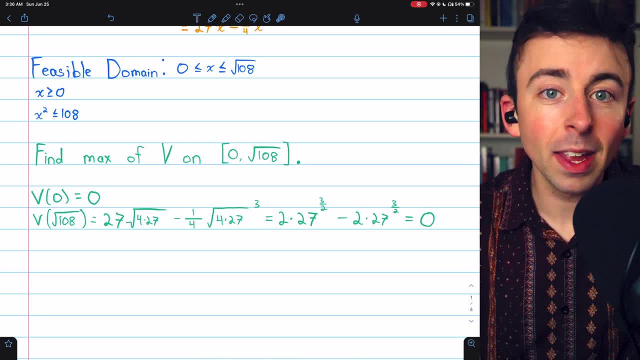 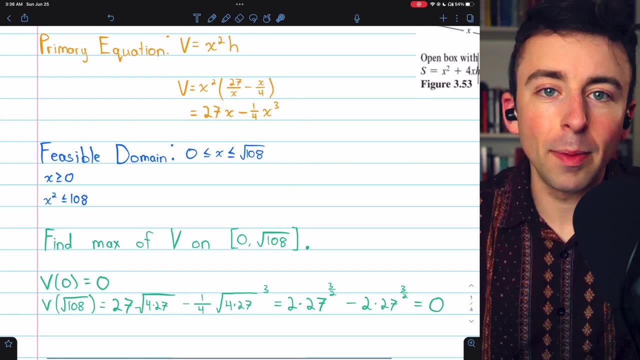 in these endpoints into the volume equation to see what we get. It's quick to see that we get 0 in both cases. If you plug 0 into the volume, well, the volume is x squared times h. so if x is 0,, 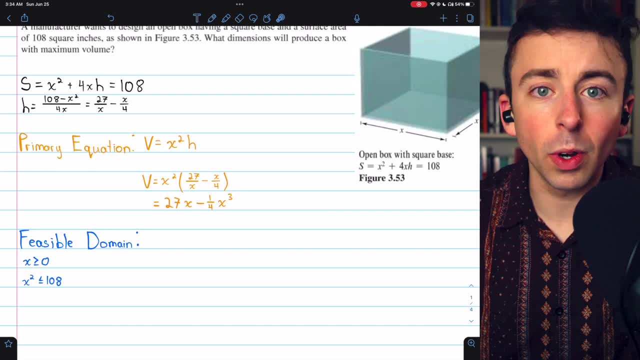 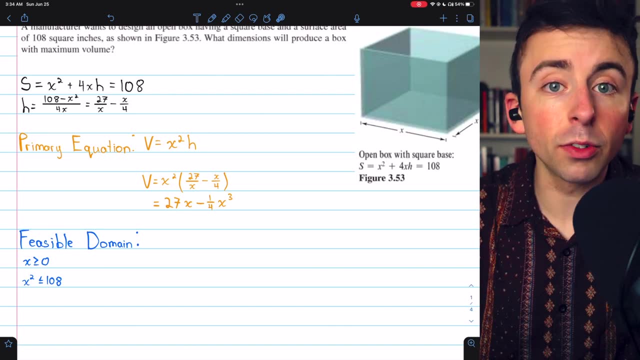 We also know that x squared has to be less than or equal to 108 by the surface area equation. X squared is in this equation and the surface area equals 108. So x squared certainly can't exceed that allowance That allowed surface area. 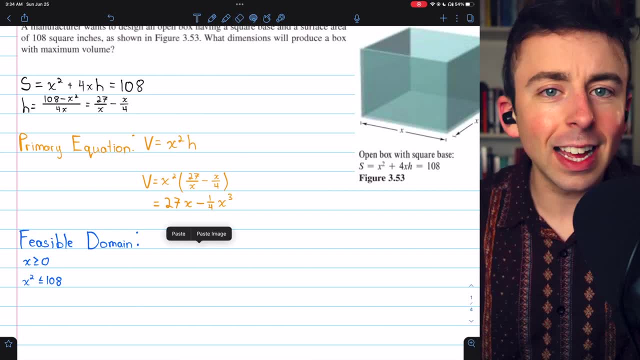 X squared is less than or equal to 108, which means that x is less than or equal to the square root of 108.. And thus this is our feasible domain: X is greater than or equal to zero, less than or equal to the square root of 108.. 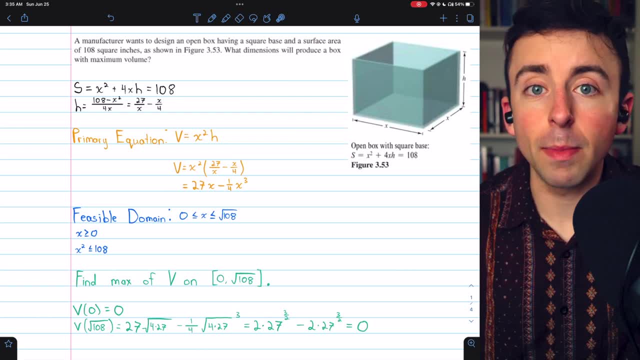 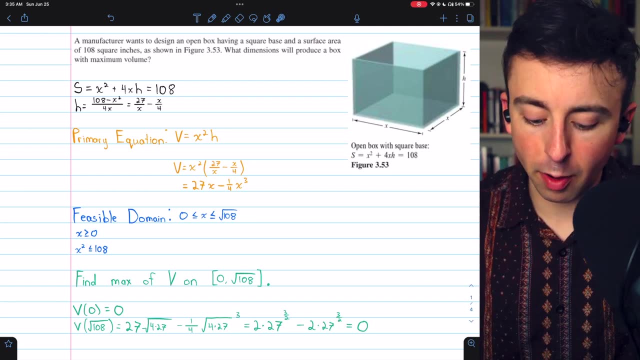 Then we're ready for the final step of using our calculus techniques to find minimums and maximums. In this case, of course, we're trying to find a maximum, and now we know that we're looking for a maximum of our volume v. 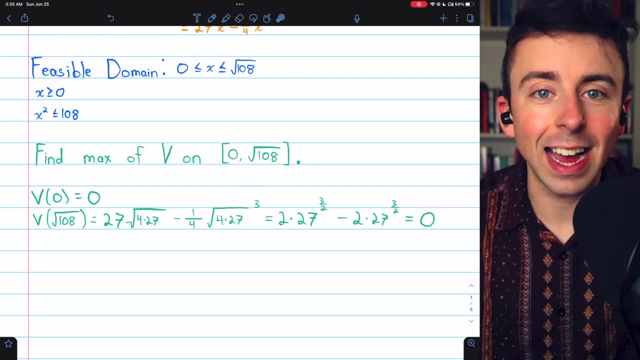 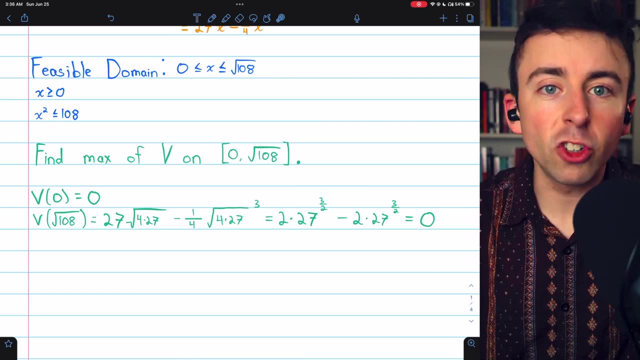 Since we're on a closed interval from zero to the square root of 108, since that's the domain, Because we're on a closed interval, we're really using the extreme value theorem and the candidates test. We need to check the candidates for a maximum. 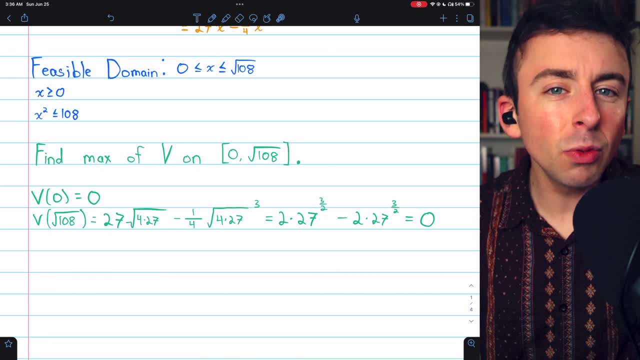 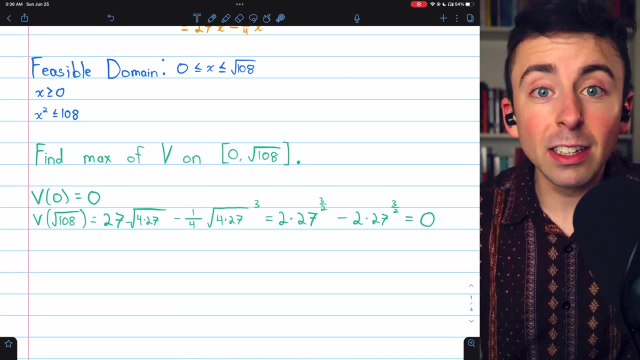 The candidates are the endpoints of this domain, as well as any critical points. Let's begin by just plugging in these endpoints into the volume equation to see what we get. It's quick to see that we get zero in both cases If you plug zero into the volume. 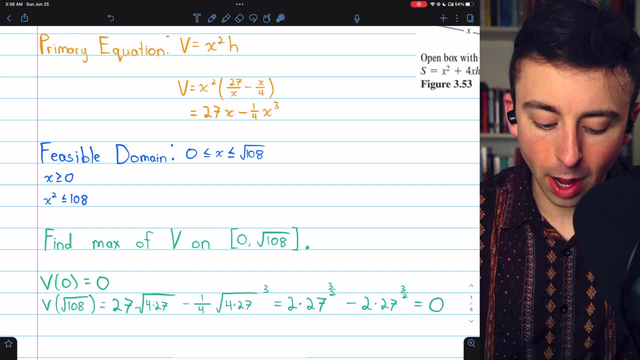 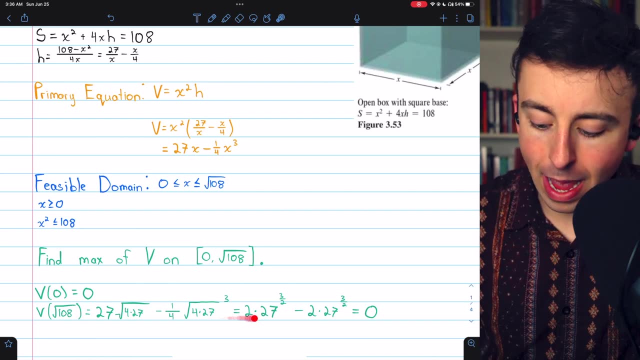 Well, X squared times H. So if X is zero, obviously the volume is zero. If we plug the square root of 108 into the volume equation, you can do the math and find that it equals zero. Or, alternatively, just look at the surface area equation. 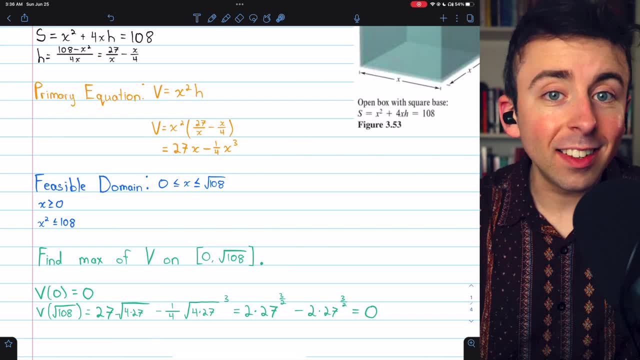 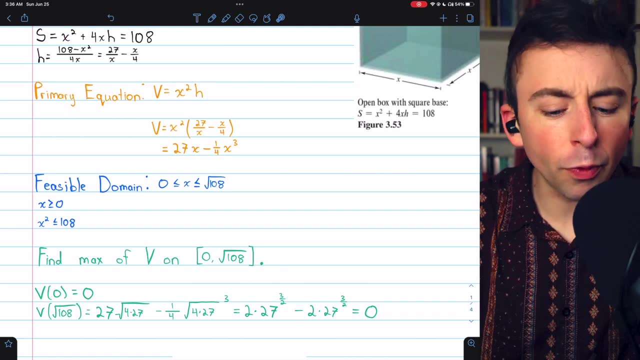 The surface area has to equal 108.. If X is the square root of 108,, then the entirety of the surface area is taken up by X squared, which forces H to be zero. If the height is zero, Then the volume is zero. 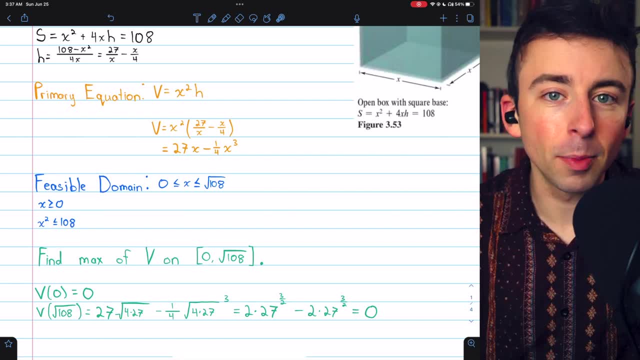 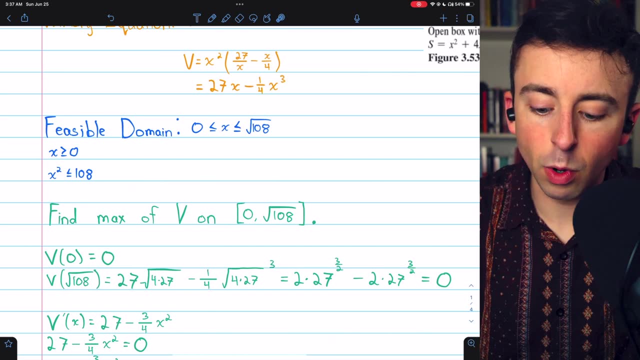 Obviously, our volume is zero, So these are certainly not going to be our maximums. Let's move on to finding critical points by taking the derivative. Remember our volume equation is 27X minus one fourth X cubed. That's what we're taking the derivative of to find our critical points. 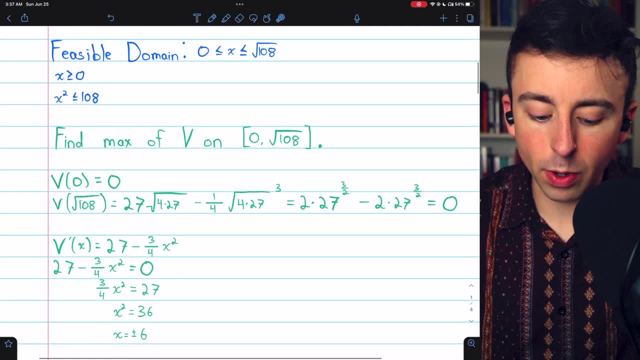 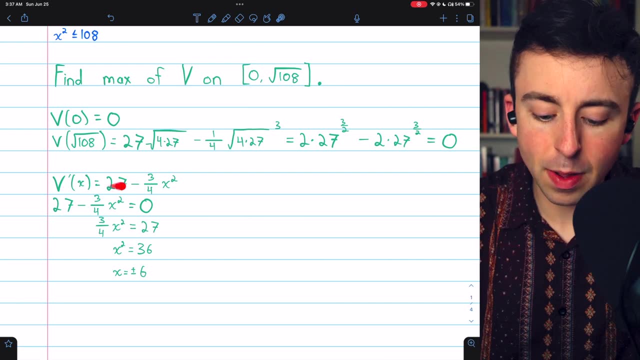 This is just going to require us to use the power rule. The derivative of 27X is 27.. And the derivative of negative one fourth X cubed is negative. three fourths X squared. So that's V prime, The derivative of our function here. 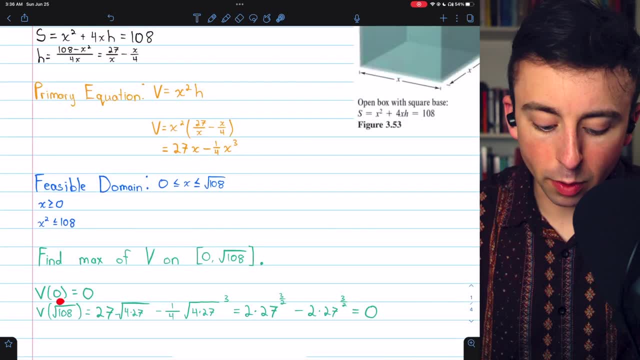 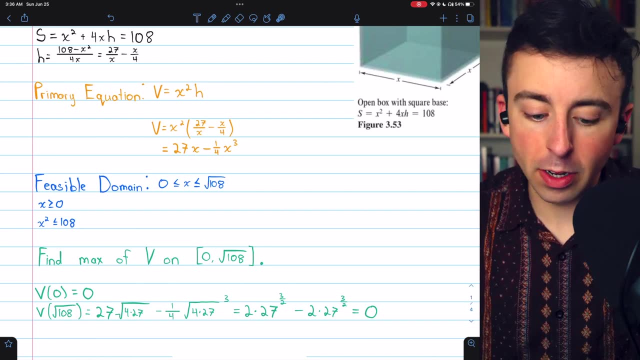 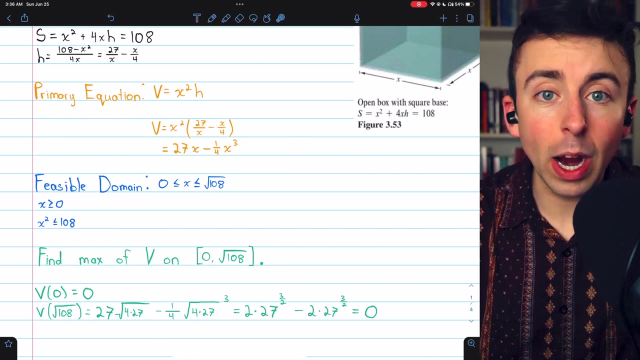 obviously volume is 0. If we plug the square root of 108 into the volume equation, you can do the math and find that it equals 0. Or alternatively, just look at the surface area equation. The surface area has to equal 108.. If x is the square root of 108, then the entirety of the surface area is. 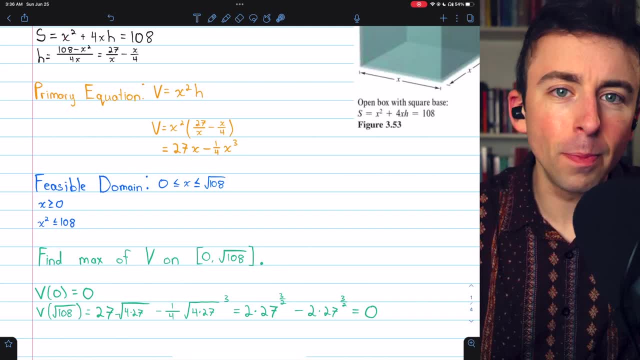 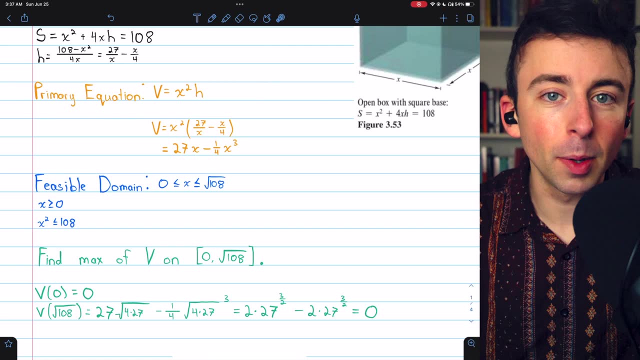 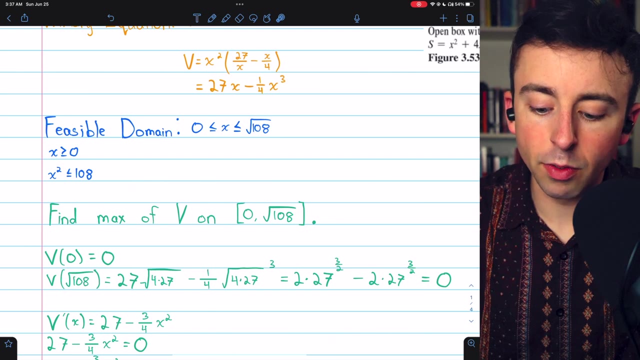 taken up by x squared, which forces h to be 0. If the height is 0, obviously our volume is 0. So these are not going to be our maximums. Let's move on to finding critical points by taking the derivative. Remember our volume equation is 27x minus one-fourth x cubed. That's what we're taking. 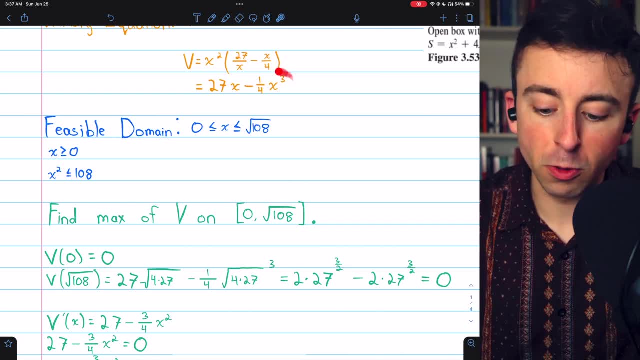 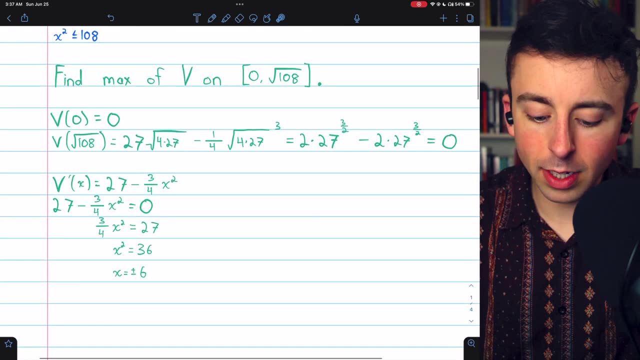 the derivative of to find our critical points. This is just going to require us to use the power rule. The derivative of 27x is 27,, and the derivative of negative one-fourth x cubed is negative three-fourths x squared. So that's v prime, the derivative of our function for volume. 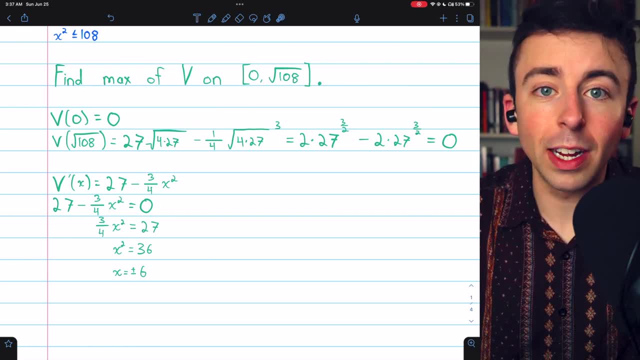 This is defined everywhere, So all we have to do to find critical points is set it equal to 0 and solve. Setting it equal to 0 and then adding three-fourths x squared to both sides, gets us here. Divide both sides by three-fourths and take the square root. x is equal to plus or minus 6,. 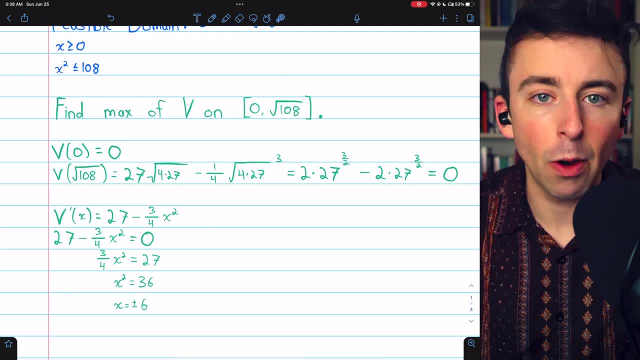 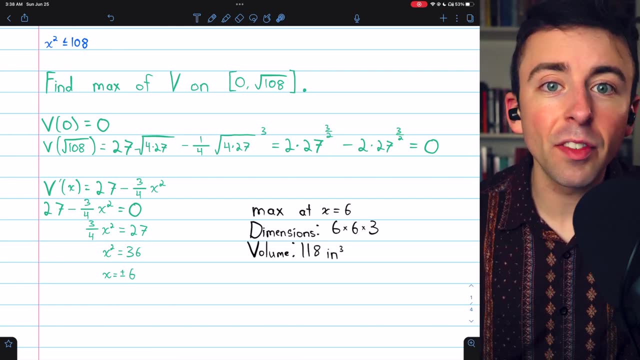 although of course it's only positive 6. that's in the allowable domain. And now we just have to make our conclusion. By the extreme value theorem, we know that our volume function has to have a maximum and a minimum on the surface area. So we're going to take the volume function and we're going to 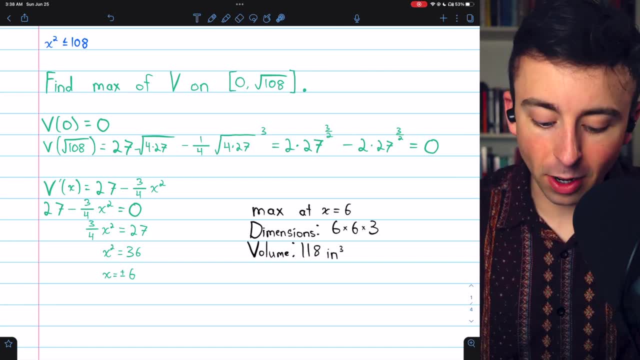 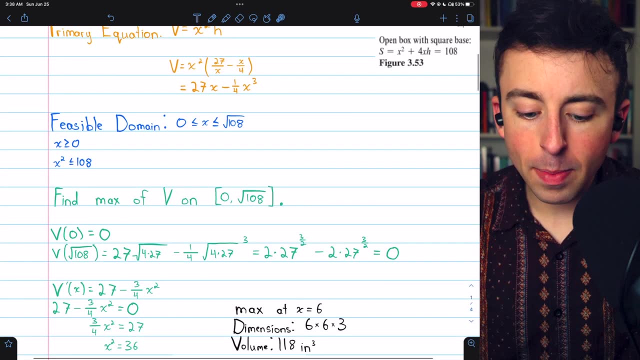 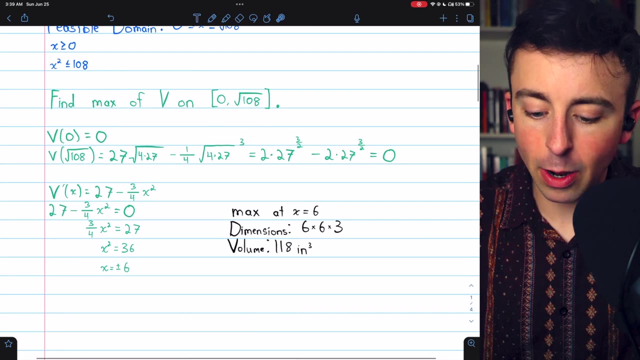 solve for the maximum. at the same time, The maximum obviously is not zero, so the maximum must occur at: x equals positive 6, and that tells us the dimensions of our box. Because, remember, we know that the height is equal to 27 over x minus x over 4.. And we just figured out that x has to. 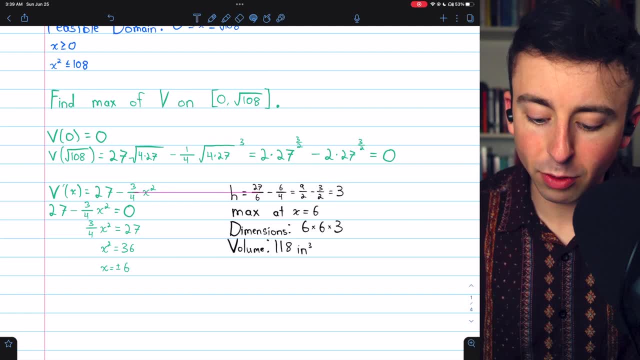 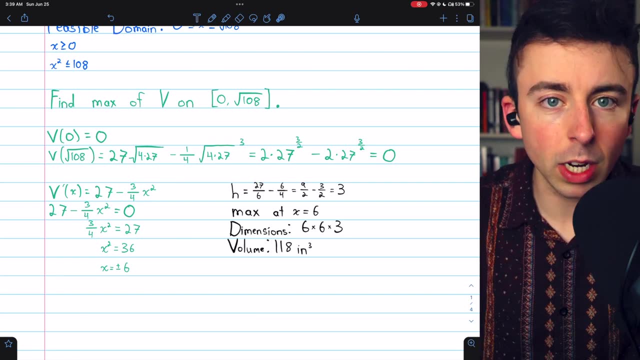 equal 6 in order to get that maximum volume. Thus we can solve for the height by plugging x equals 6 into that expression And we find that the height is forced to be 3.. So we're going to So the dimensions of the box. that will maximize the volume, given that the surface area has. 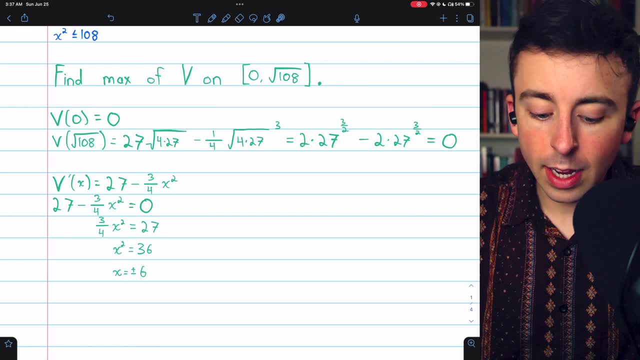 Okay, That's that, Thank you, Have a great day, Bye, Bye, Bye. Bye Bye for volume. This is defined everywhere, so all we have to do to find critical points is set it equal to zero and solve. Setting it equal to zero and then adding three-fourths x squared to both sides. 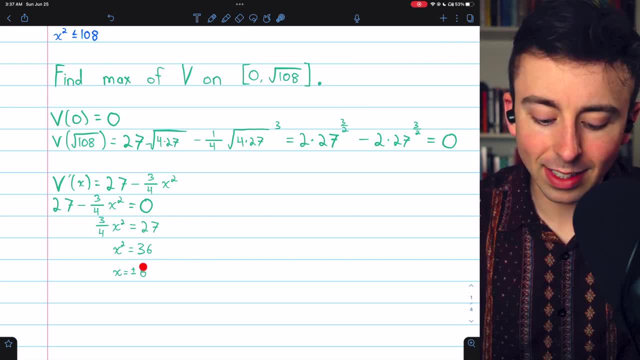 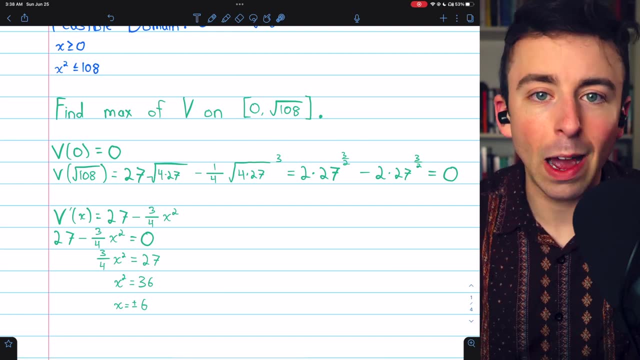 gets us here. Divide both sides by three-fourths and take the square root. x is equal to plus or minus six, although of course it's only positive six. that's in the allowable domain. And now we just have to make our conclusion. By the extreme value theorem we know that our volume function. 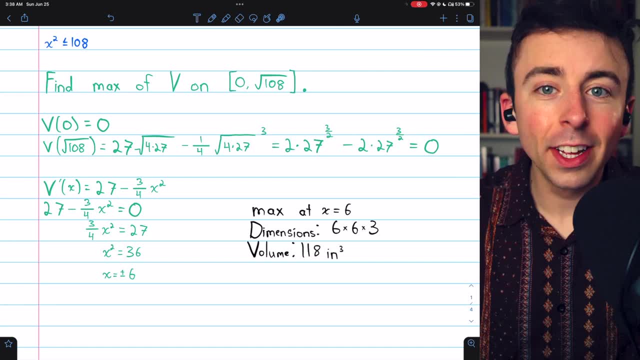 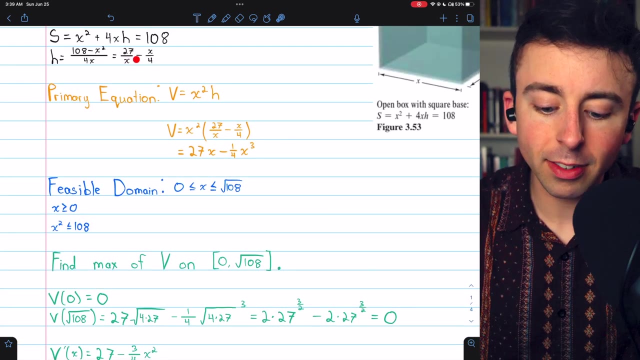 has to have a maximum and a minimum on this interval. The maximum obviously is not zero, so the maximum must occur at x equals positive six, And that tells us the dimensions of our box, because, remember, we know that the height is equal to 27 over x, minus x over four. 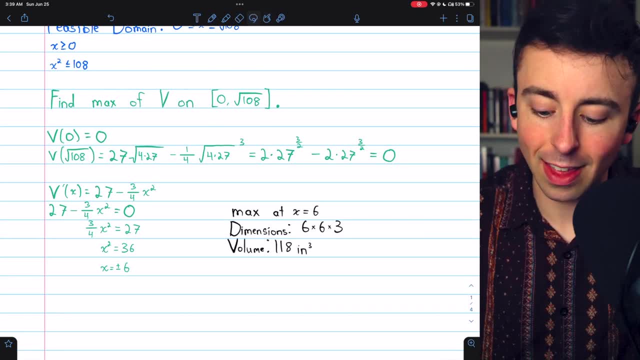 and we just figured out that x has to equal six in order to get that maximum volume. Thus we can solve for the height by plugging x equals six into that expression and we find the height is forced to be three, So the dimensions of the box that will maximize the volume, given that the 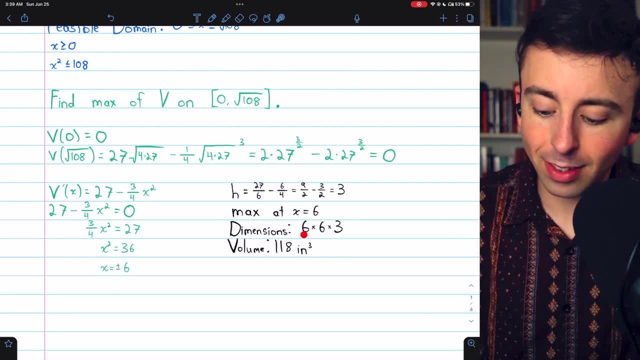 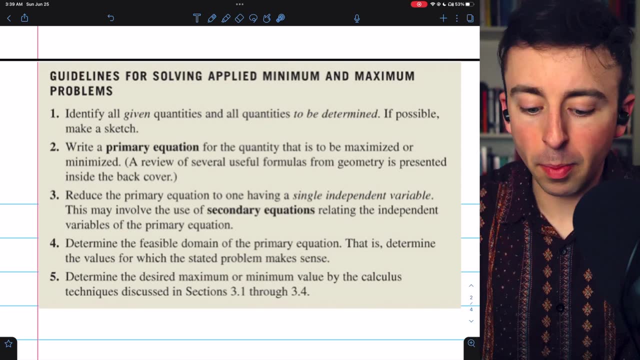 surface area has to be 108 inches. squared is going to be six by six by three, giving a volume of 118 inches cubed. That's how you solve an optimization problem. Here's a look at the guidelines from Larson's calculus before we move on to the second problem. The first thing we did, 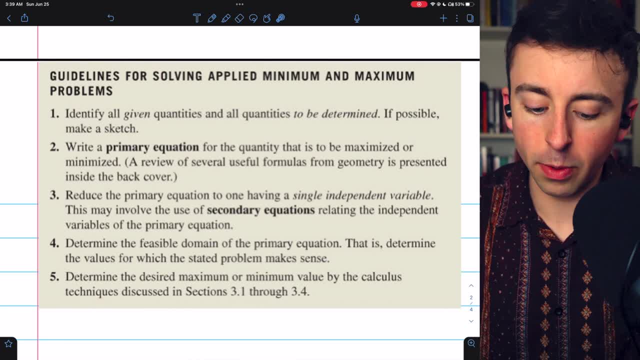 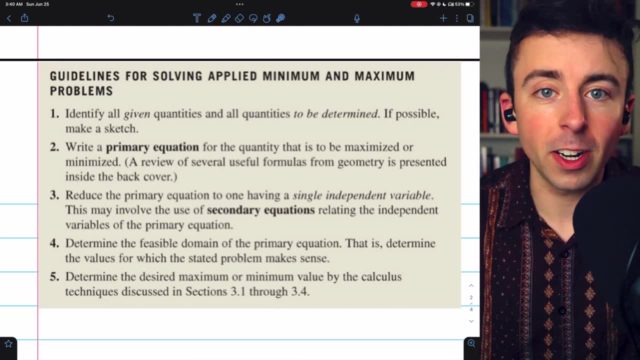 was to identify all given quantities, Quantities that we don't know, make a sketch, if possible. In the first example, we were given a picture, so we didn't need to make a sketch And, since we knew the surface area, we wrote an. 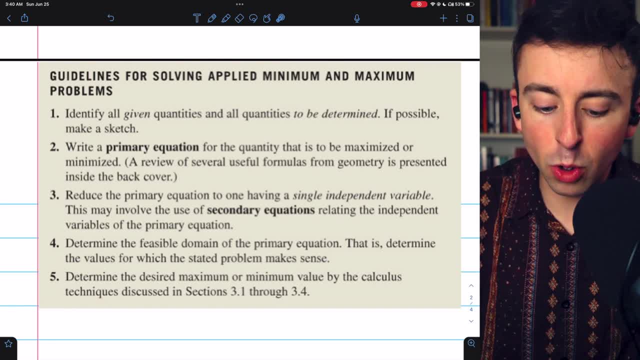 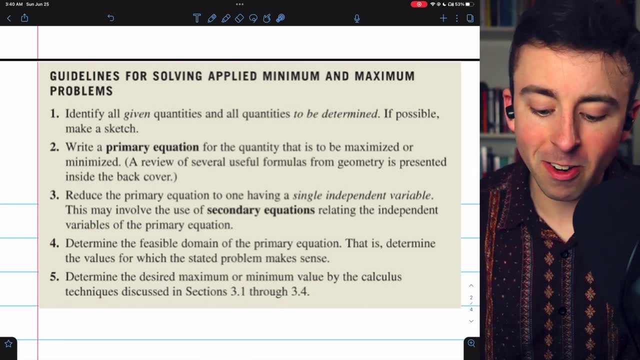 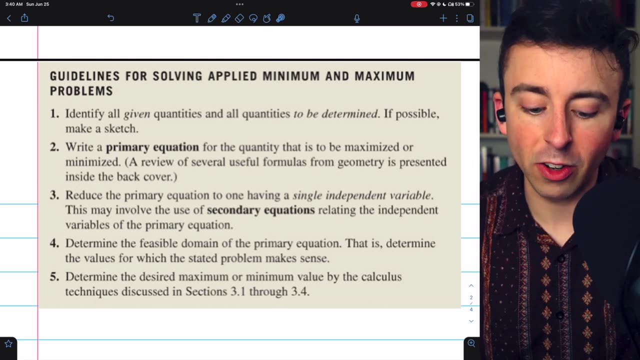 equation for that called a secondary equation. In step two we wrote a primary equation for the equation that is to be optimized, And in step three we reduced that primary equation to one having a single independent variable. To do that we made use of the secondary equations that we 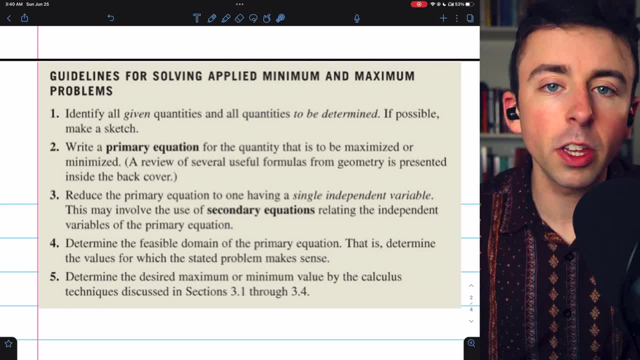 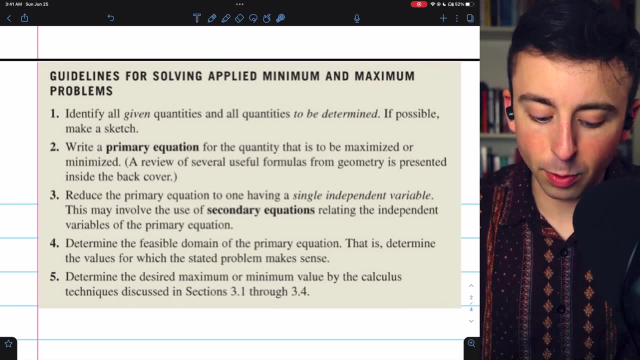 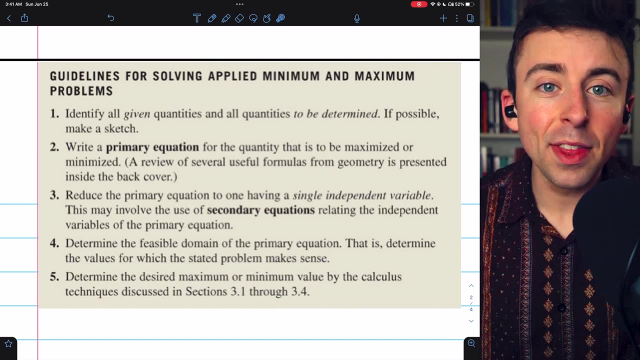 wrote in step one in order to rewrite the volume in terms of a single variable. Step four was to determine the feasible domain of the primary equation, And then step five was to just use calculus to find the maximum or the minimum. If the domain was a closed interval, like in our previous case, then we don't have to use the first. 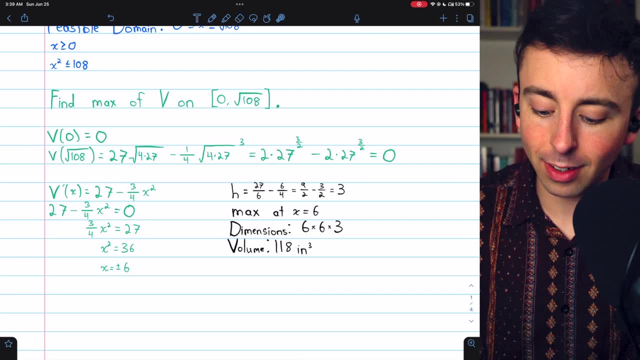 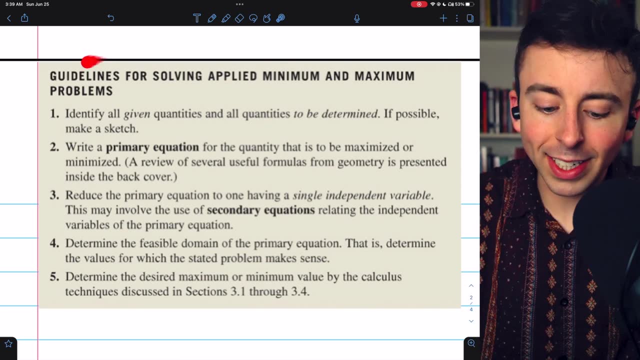 to be 108 inches, squared is going to be 6 by 6 by 3, giving a volume of 118 inches cubed. That's how you solve an optimization problem. Here's a look at the guidelines from Larsen's calculus before we move on to the second problem. 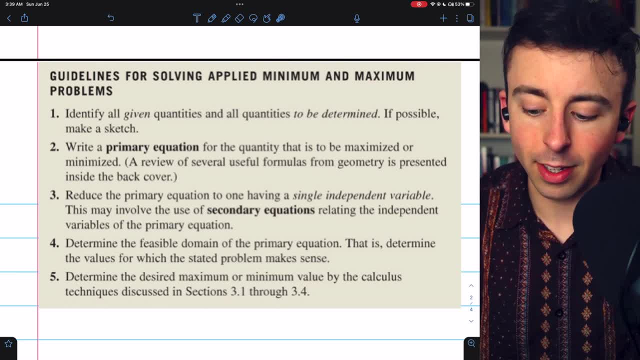 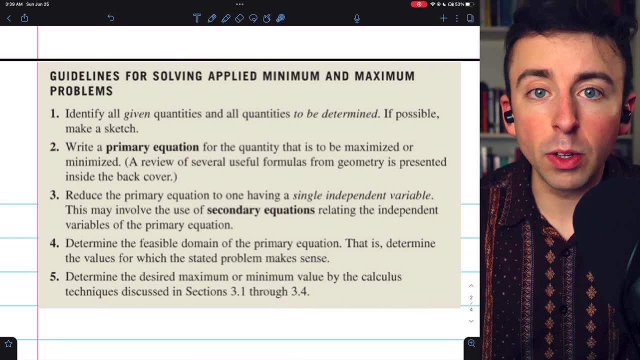 The first thing we did was to identify all given quantities and quantities that we don't know, make a sketch if possible. In the first example, we were given a picture, so we didn't need to make a sketch, And since we knew the surface area, we wrote an equation for that, called a secondary equation. 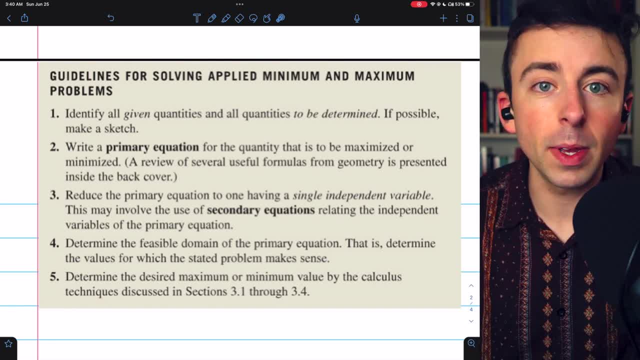 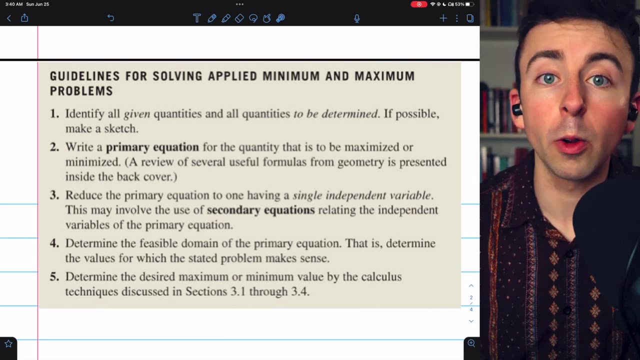 In step 2, we wrote a primary equation for the equation that is to be optimized, And in step 3 we reduced that primary equation to one having a single independent variable. To do that, we made use of the secondary equations that we wrote in step 1 in order to rewrite. 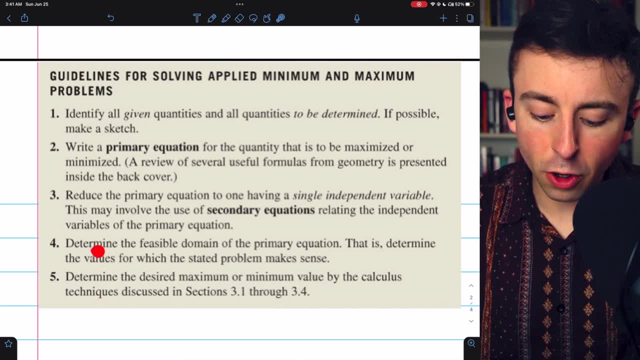 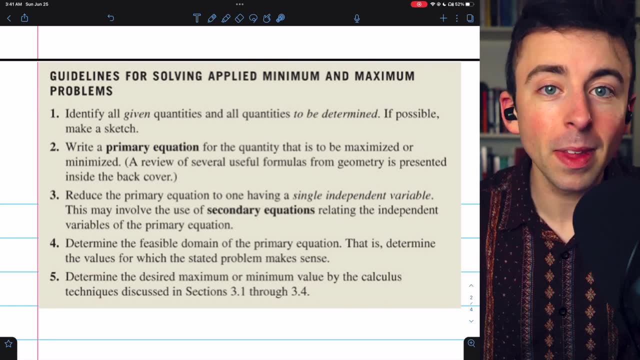 the volume in terms of a single variable. Step 4 was to determine the feasible domain of the primary equation, And then step 5 was to just use calculus to find the maximum or the minimum. If the domain was a closed interval, like in our previous case, then we don't have to. 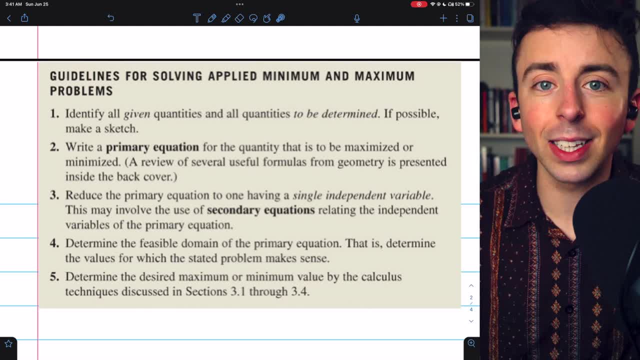 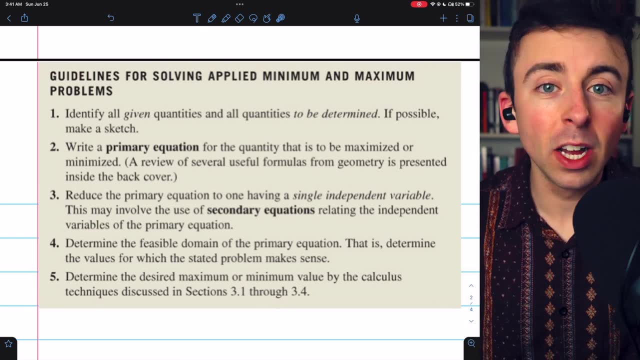 use the first derivative test or the second derivative test for classifying critical points, because we can just use the extreme value theorem and the candidate's test. In our last example. we're not going to have a closed interval, and so we will have to. 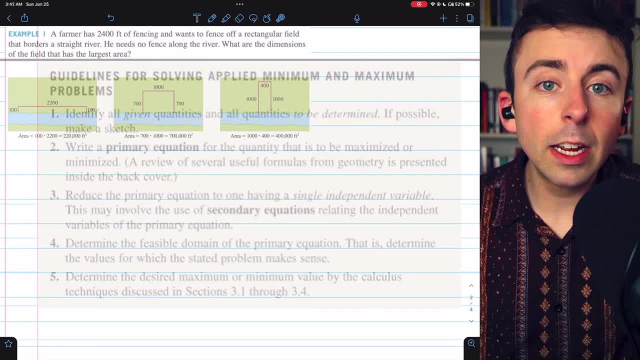 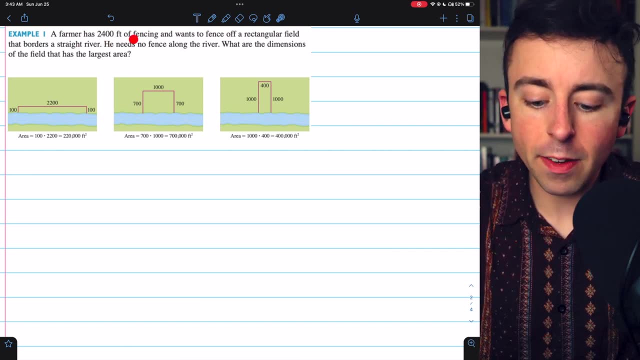 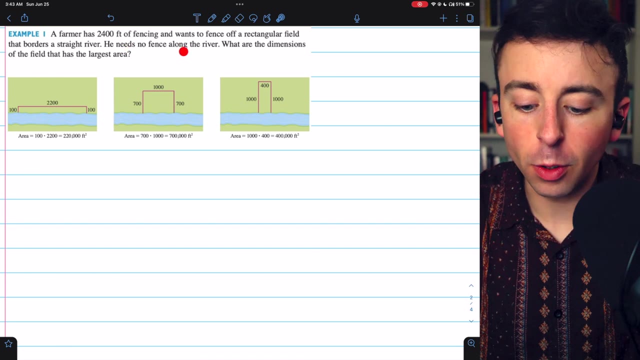 use either the first derivative test or second derivative test. Here is our second example. I think this is from Stewart's calculus. A farmer has 2,400 feet of fencing and wants to fence off a rectangular field that borders a straight river. He needs no fence along the river. 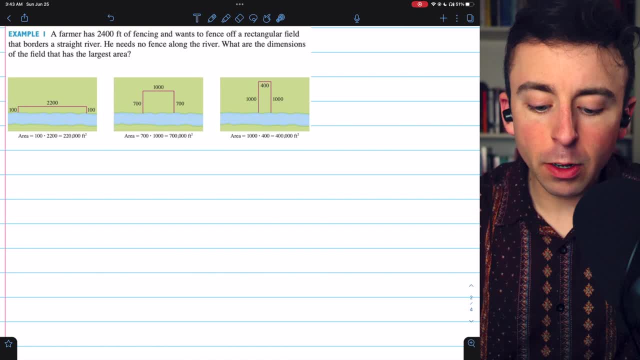 What are the dimensions of the field that has the largest area? Here's a few examples of possibilities. You can see that if we use a short and fat design, then we get a pretty small area, And if we get a long and skinny design, we also get a small area. 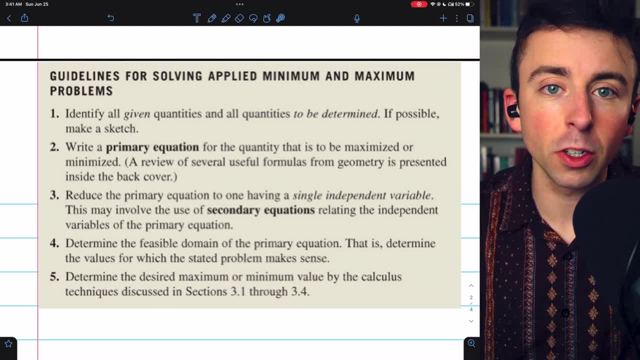 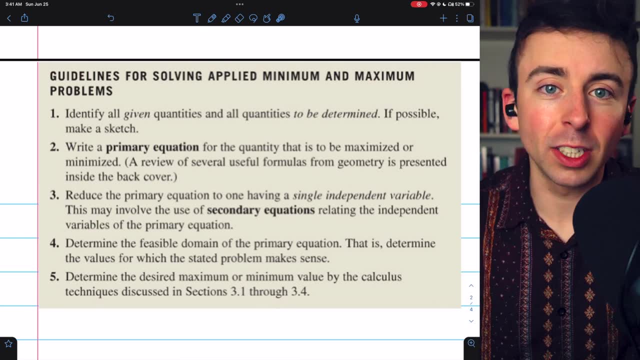 derivative test or the second derivative test for classifying critical points, because we can just use the extreme value theorem and the candidates test. In our last example, we're not going to have a closed interval, and so we will have to use either the 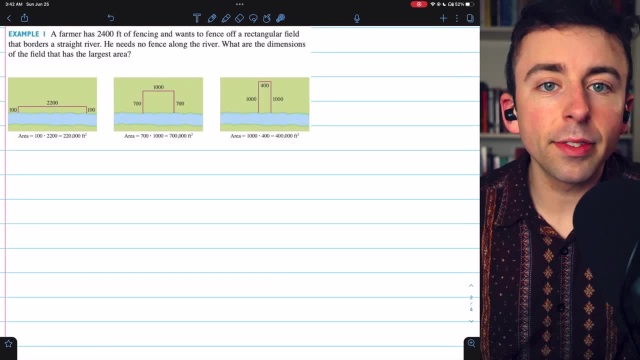 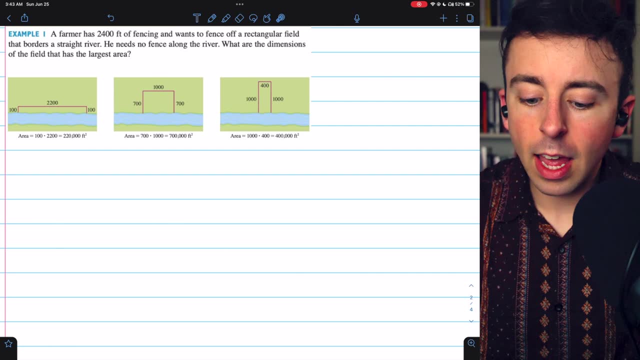 first derivative test or second derivative test. Here is our second example. I think this is from Stewart's calculus. A farmer has 2,400 feet of fencing and wants to fence off a rectangular field that borders a straight river. He needs no fence along the river. What are the dimensions of? 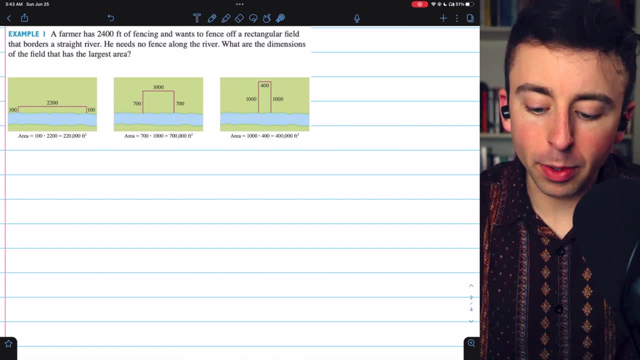 the field that has the largest area. Here's a few examples of possibilities. You can see that if we use a short and fat design, then we get a pretty small area, And if we get a long and skinny design, we also get a small area. If we go for a more balanced approach, though, the area is much 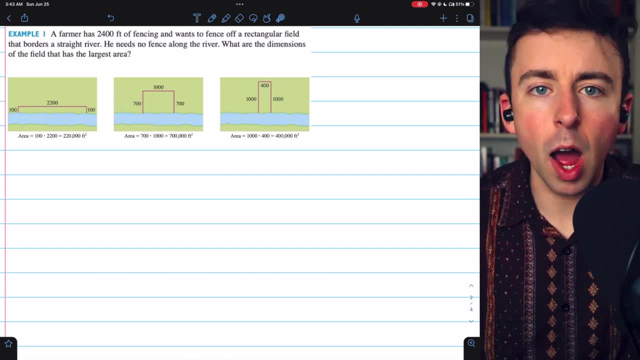 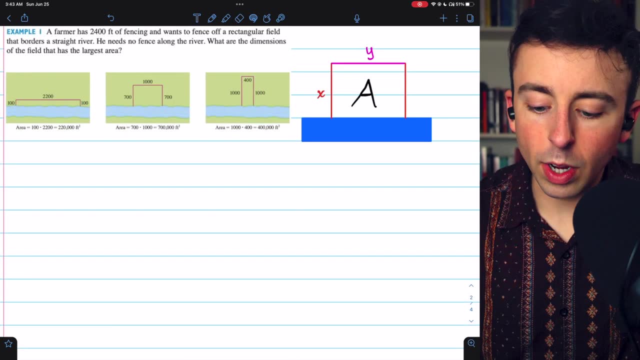 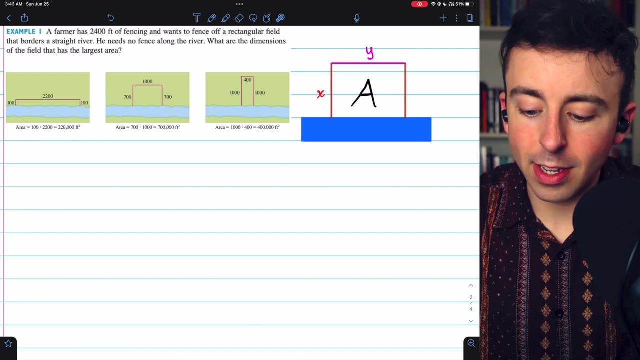 larger. So there's got to be some optimal point, some optimal dimensions for this fenced off area, giving us a maximum area, And that's what we're looking for. We'll begin with a sketch of the situation. We have this river and then we have our fenced off area. We'll say that the 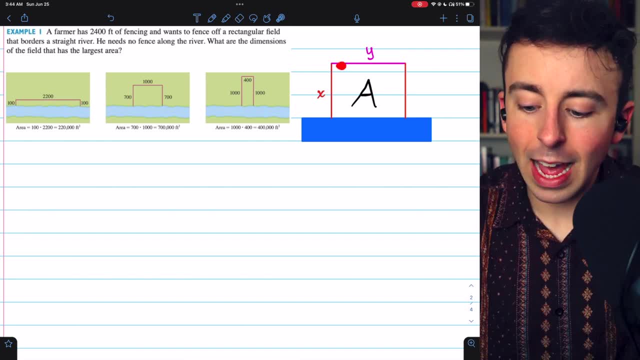 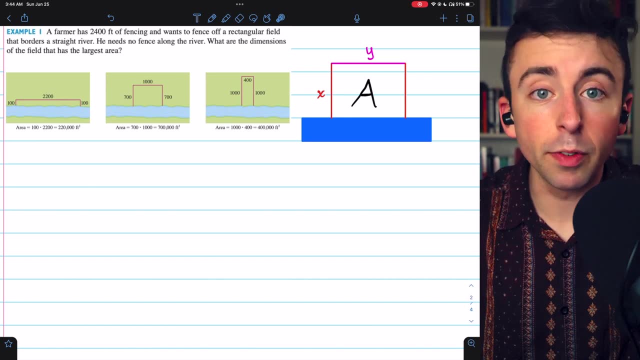 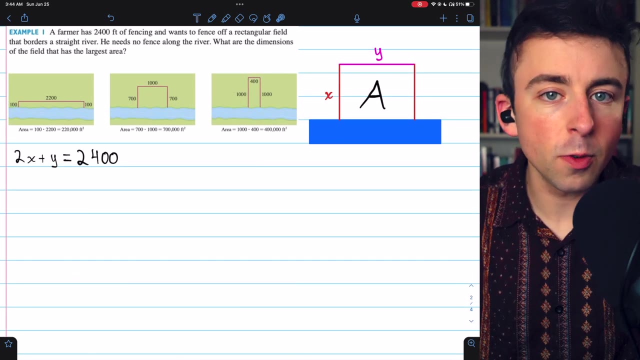 side of our rectangle opposite the river side, has a length of y, And then the other two sides that we need both have a length of x. We, of course, are trying to maximize the area of this rectangle. We do have some given information, which is that we have 2,400 feet of fencing, So x plus x plus y. 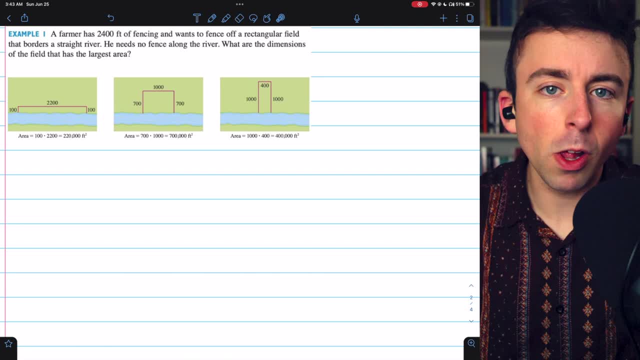 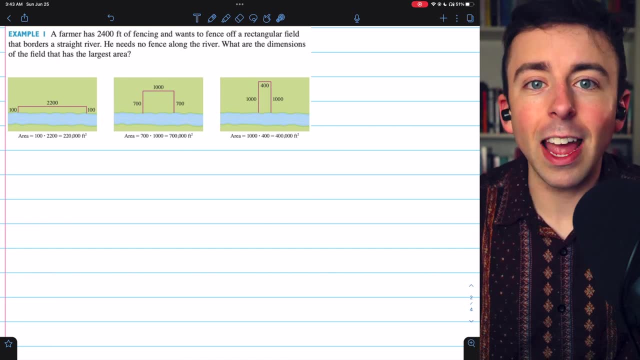 If we go for a more balanced approach, though, the area is much smaller. The area is much smaller, The area is much larger. So there's got to be some optimal point, some optimal dimensions for this fenced off area, giving us a maximum area. 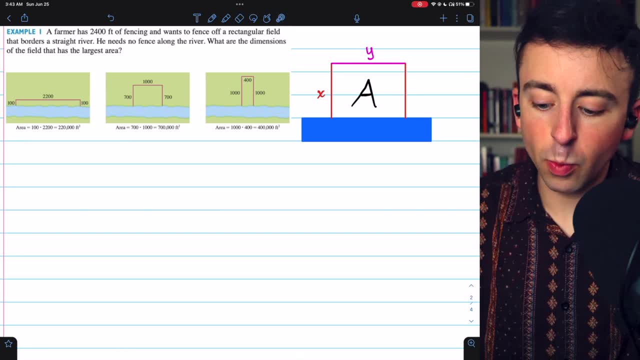 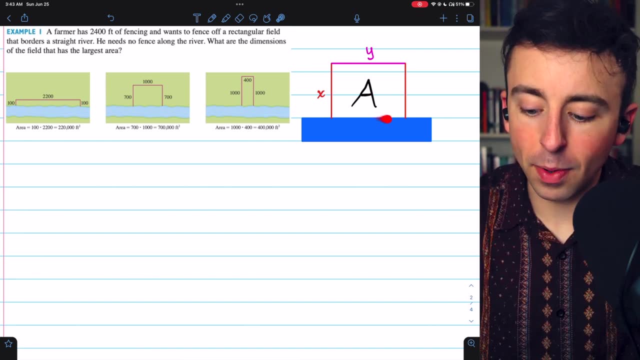 And that's what we're looking for. We'll begin with a sketch of the situation. We have this river, and then we have our fenced off area. We'll say that the side of our rectangle opposite the river side has a length of y, and then 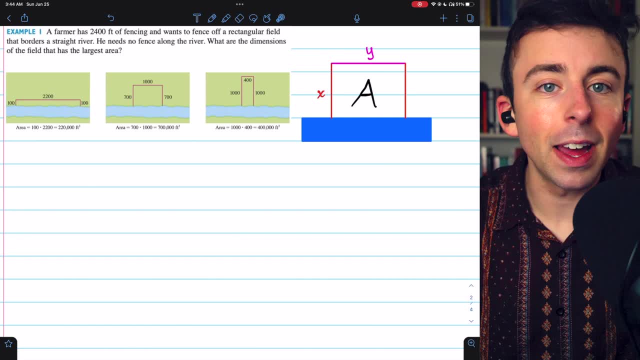 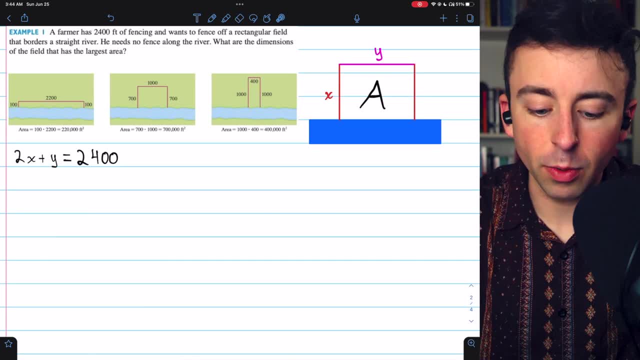 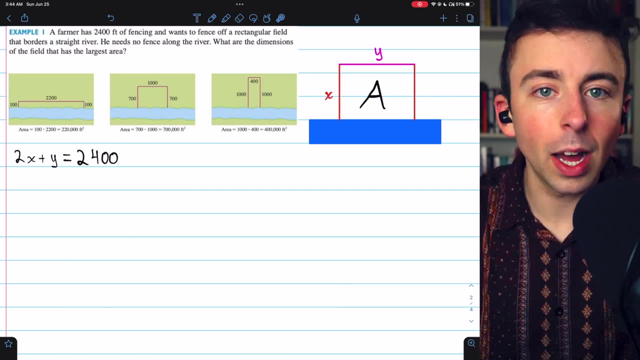 We're trying to maximize the length of y. We're trying to maximize the length of the area of this rectangle. We do have some given information, which is that we have 2,400 feet of fencing. So x plus x plus y or 2x plus y, will have to equal 2,400.. 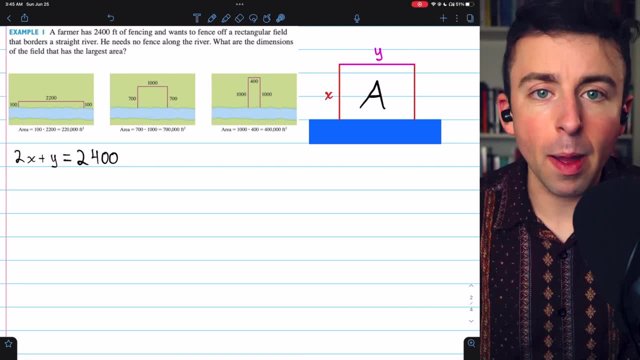 That's all the fencing we have. Now we can move on to the primary equation. Let's write an equation for the quantity that we're trying to optimize. We're trying to maximize area, so we'll write an equation for that. The area of this rectangle is, of course, just x times y. 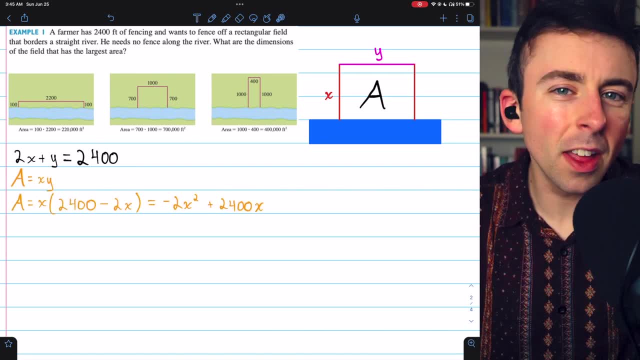 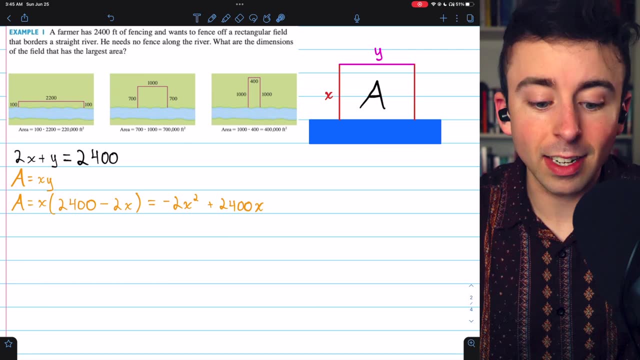 The area of this rectangle is, of course, just x times y. This is our primary equation: a equals xy. Again, though, we've got two variables here. We need an equation in terms of a single variable. We can fix that pretty easily. this is step three, by going back to our secondary equation. 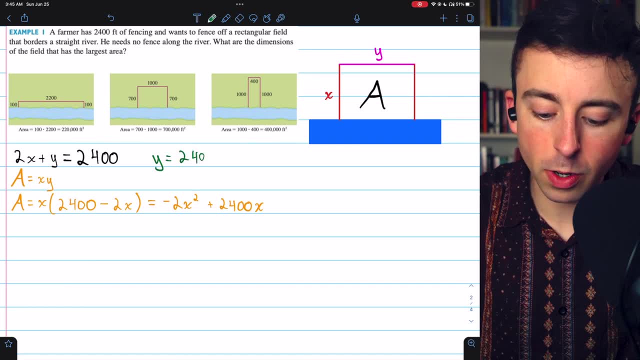 and solving for y, y is equal to 2,400 minus 2x, And then we can plug that in for y in our area equation to find that the area is equal to x times 2,400 minus 2x, which is the same as negative 2x squared plus 2x squared minus. 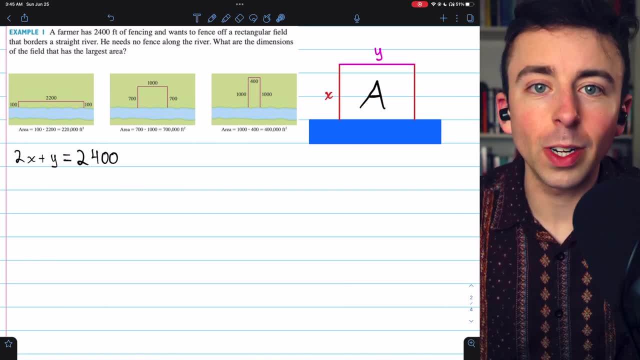 or 2x plus y, will have to equal 2,400.. That's all the fencing we have. Now we can move on to the primary equation. Let's write an equation for the quantity that we're trying to optimize, We're trying to maximize. 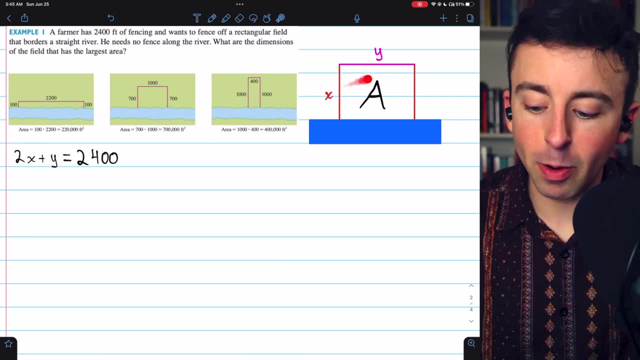 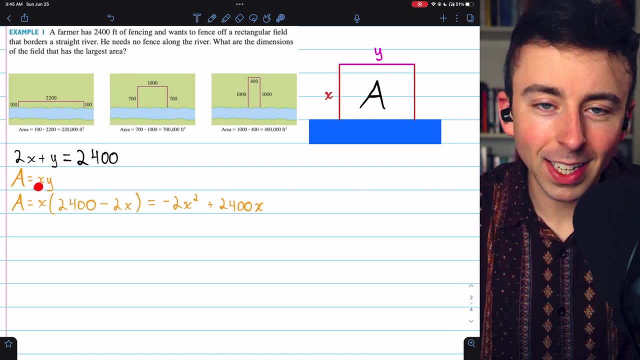 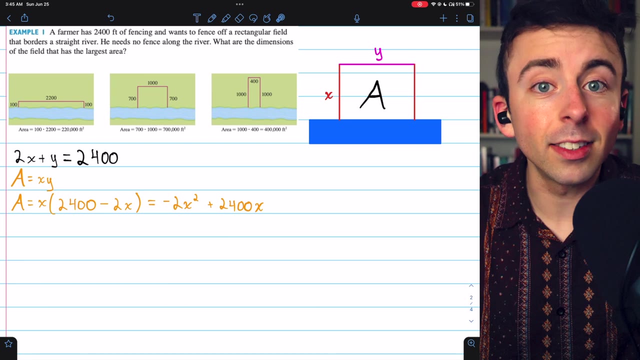 area, so we'll write an equation for that. The area of this rectangle is, of course, just x times y, So that's our primary equation: a equals xy. Again, though, we've got two variables here. We need an equation in terms of a single variable. We can fix that pretty easily. This is step three. 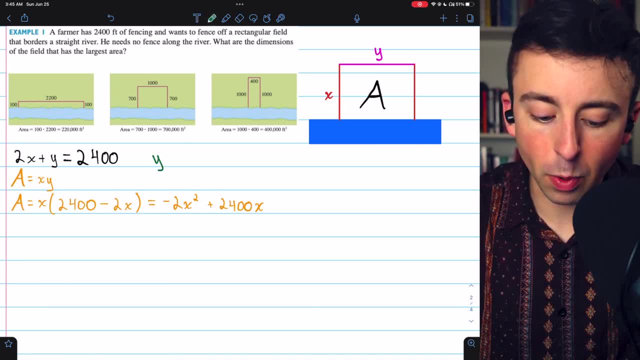 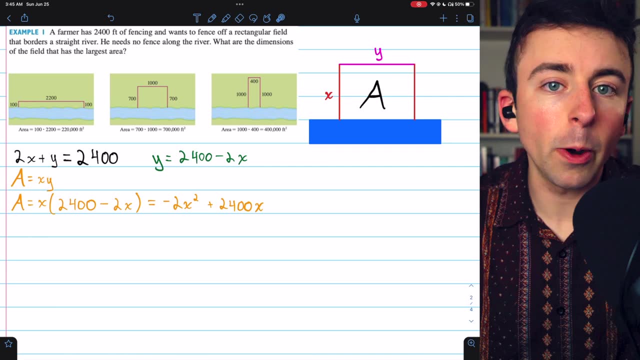 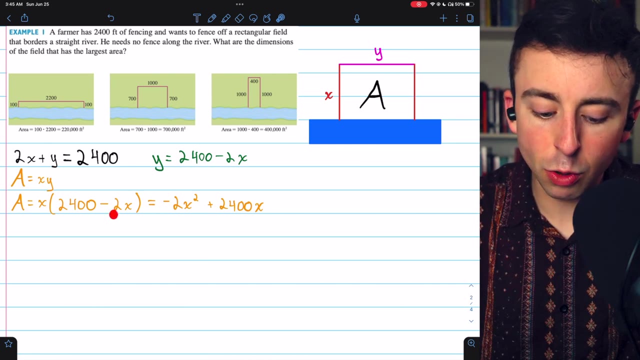 By going back to our secondary equation and solving for y, y is equal to 2,400 minus 2x, And then we can plug that in for y in our area equation to find that the area is equal to x times 2,400 minus 2x, which is the same as negative 2x squared plus 2,400 x. Now we have a primary. 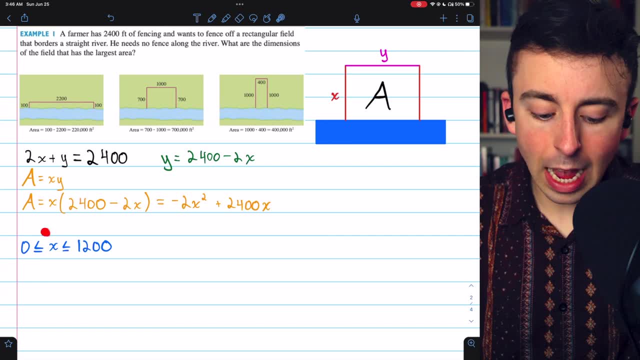 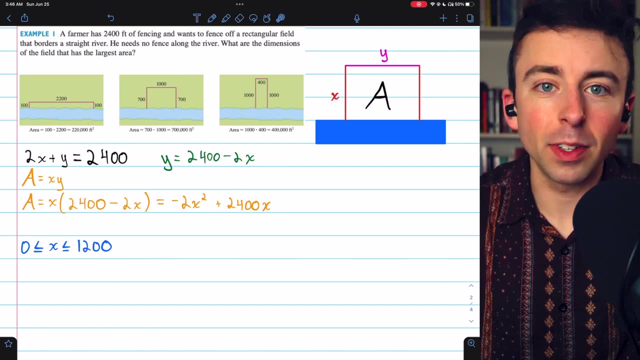 equation in terms of a single variable. The next step is to establish the feasible domain. In this case, x has to be between 0 and 1,200.. We obviously can't have a negative dimension on our rectangle And x has to be less than or equal to x. So we can plug that in for y in terms of a single variable. 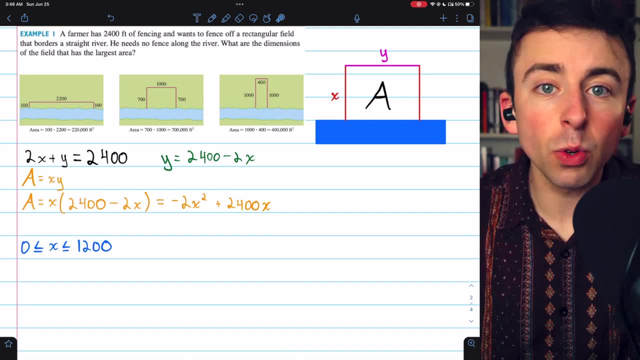 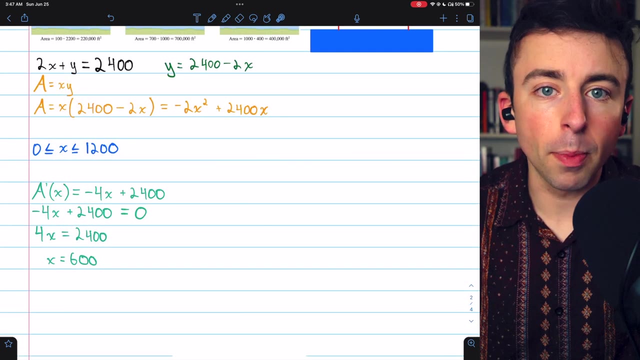 Again, this is a closed interval. Now we're on to the calculus part. We're trying to find the maximum value of this area function on the closed interval between 0 and 1,200.. It's easy to see that at the endpoints of this interval the area would be 0.. When x equals 1,200,. 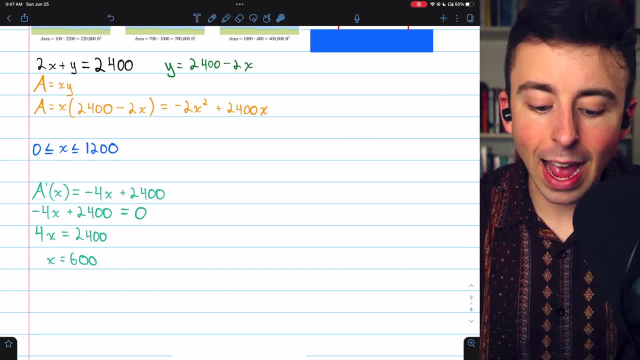 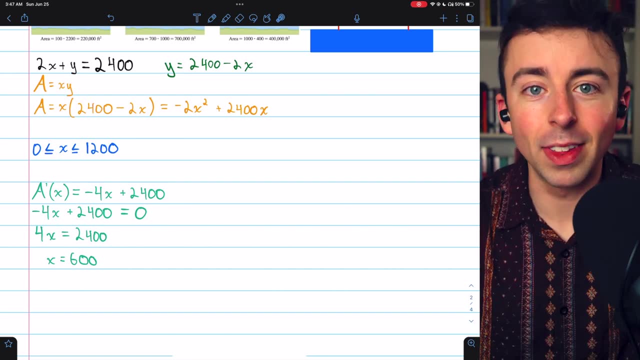 the area is obviously 0. And when x equals 1,200, well, the 2x takes up all of the fencing, And so y would be forced to be 0, thus again making the area 0. So whatever our maximum is, it's going. 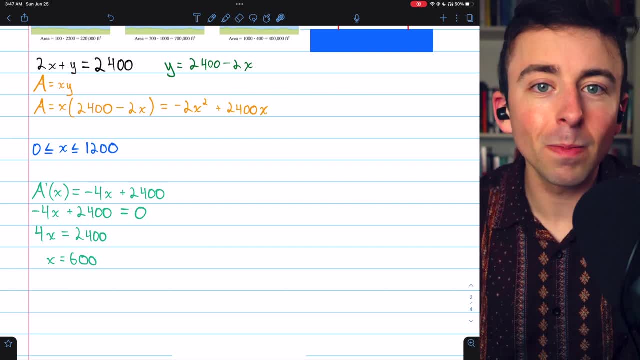 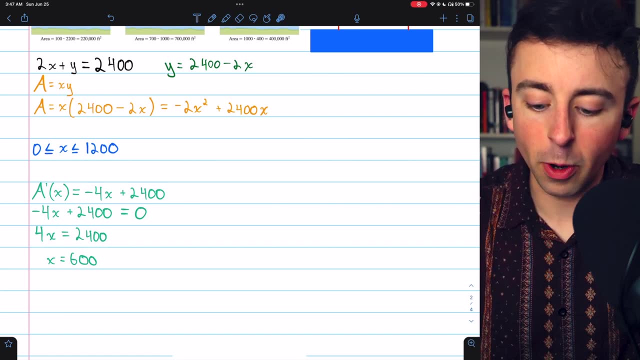 to be at a critical point. Let's take the derivative of the area function to find the critical point in the interval. We just apply the power rule to find a prime. The derivative of negative 2x squared is negative 4x and the derivative of 2,400x is just 2,400. Then 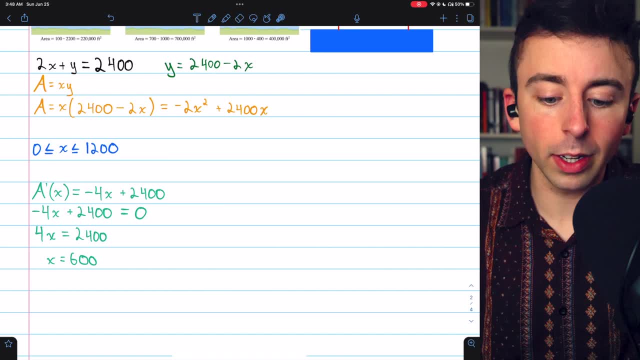 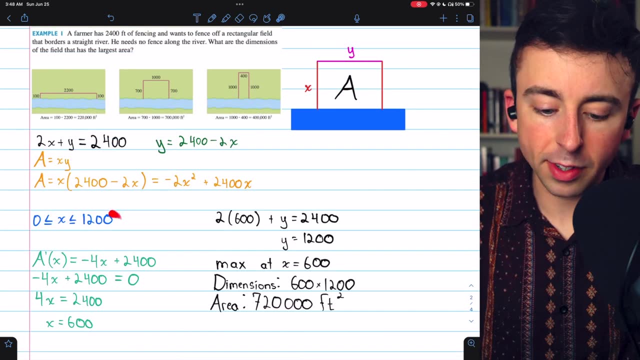 since this isn't undefined anywhere, to find critical points, we just set it equal to 0. And that gets us here. x equals 600.. And again we are on a closed interval. We're really using the extreme value theorem here. There has to be a max and a min on this closed interval. The 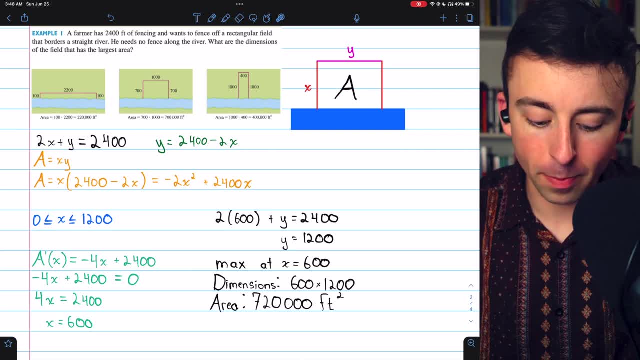 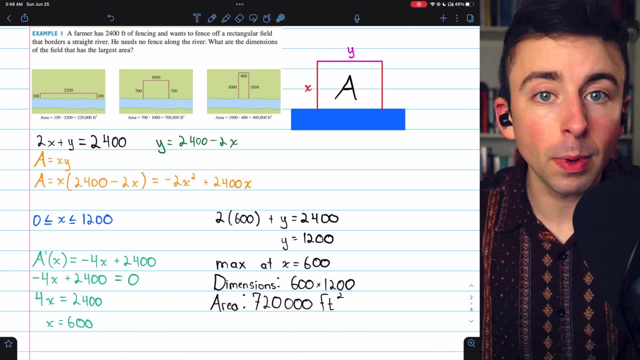 maximum obviously isn't 0, so it must occur at x equals 600.. If x equals 600, we know that y must equal 1,200, just by plugging 600 into this equation, That would give us that 1,200 plus y is 2,400, so y is 1,200.. Thus we have a maximum at x equals. 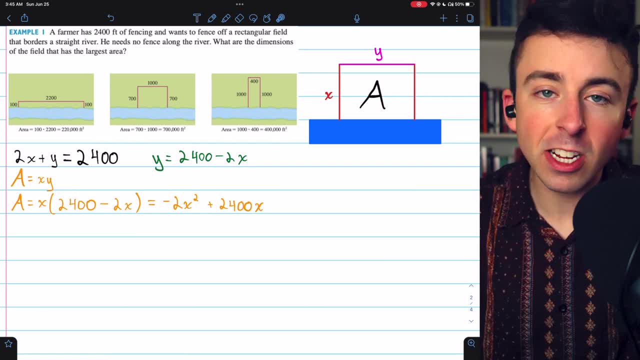 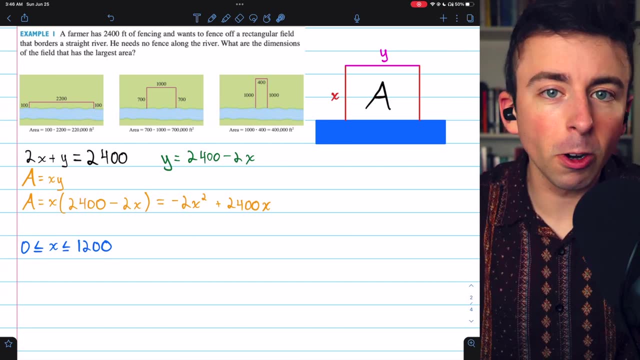 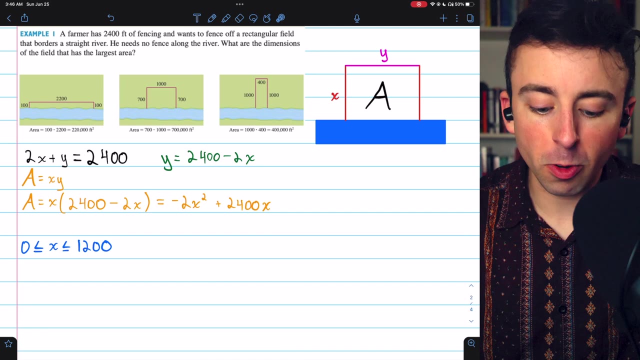 plus 2400x. Now we have a primary equation in terms of a single variable. The next step is to establish the feasible domain. In this case, x has to be between 0 and 1200.. We obviously can't have a negative dimension on our rectangle- and x has to be less than or equal to 1200, because the amount 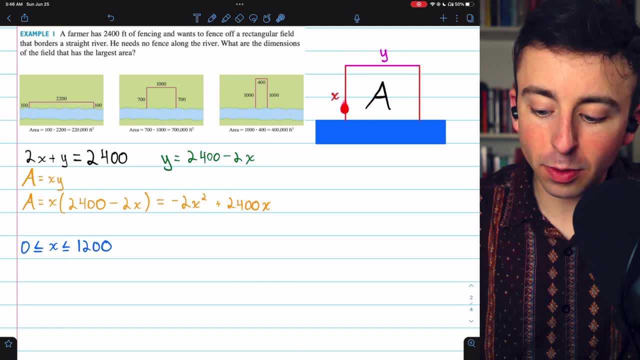 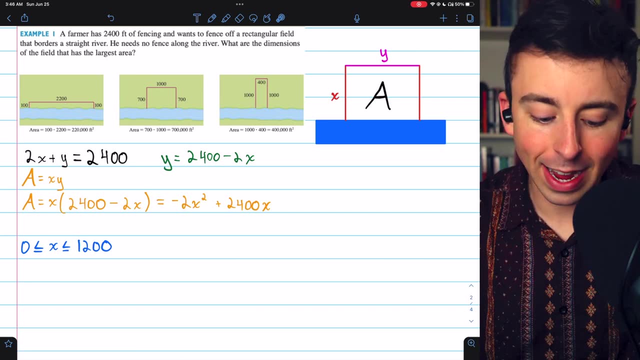 of fencing we have is 2400, and there's two copies of x in our design, So x can't exceed 1200.. We don't have that much fencing, So x is between 0 and 1200.. Again, this is a closed interval. 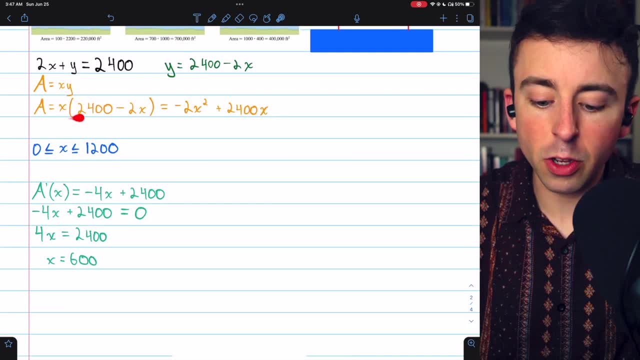 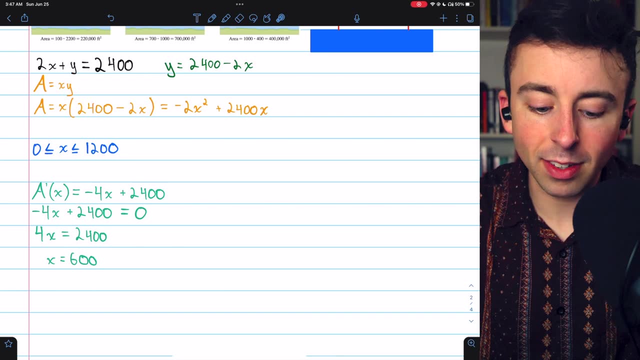 Now we're on to the calculus part. We're trying to find the maximum value of this area function on the closed interval between 0 and 1200.. It's easy to see that at the endpoints of this interval the area would be 0. When x equals 0,, the area is obviously 0. And when x equals 1200,. 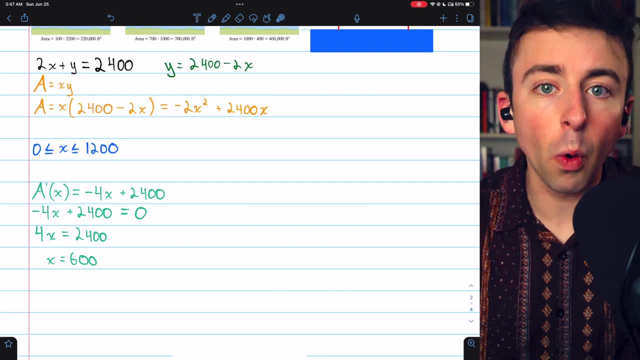 well, the 2x takes up all of the fencing, and so y would be forced to be 0, thus again making the area 0. So whatever our maximum is, it's going to be at a critical point. Let's take the derivative of the area function to find the critical point in the interval We just 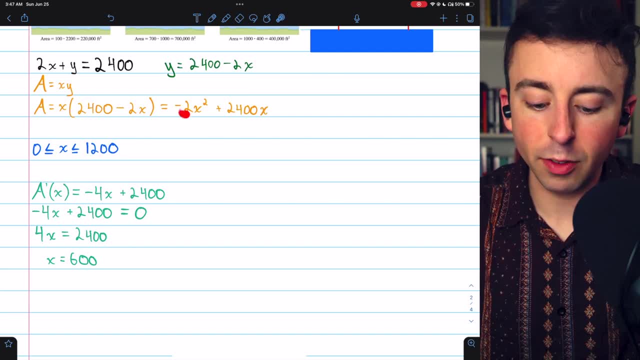 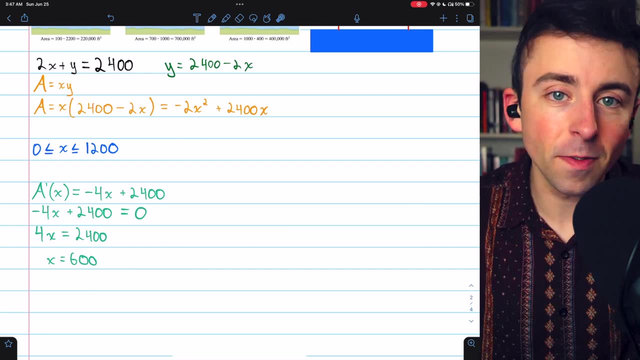 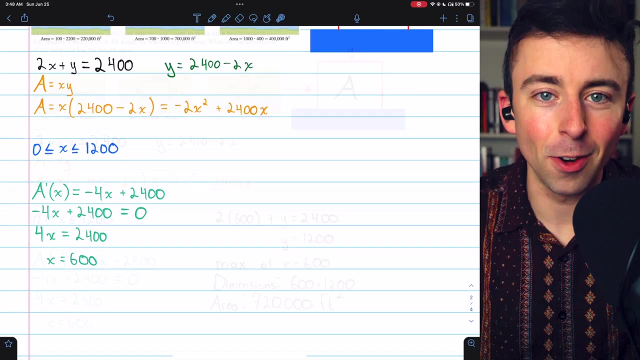 apply the power rule to find a prime. The derivative of negative 2x squared is negative 4x and the derivative of 2400x is just 2400.. Then, since this isn't undefined anywhere to find critical points, we just set it equal to 0, and that gets us here. x equals 600. 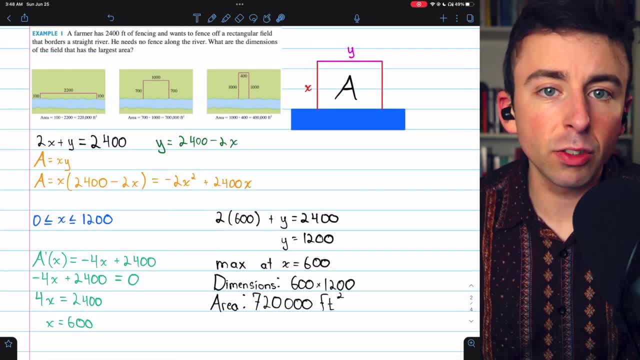 And again we are on a closed interval. We're really using the extreme value theorem here. There has to be a max and a min on this closed interval. The maximum obviously isn't 0, so it must occur at x equals 600.. If x, 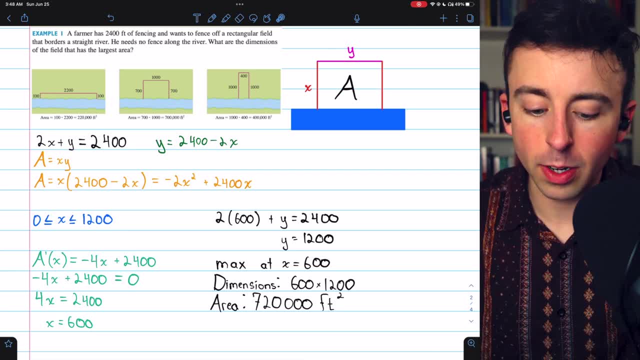 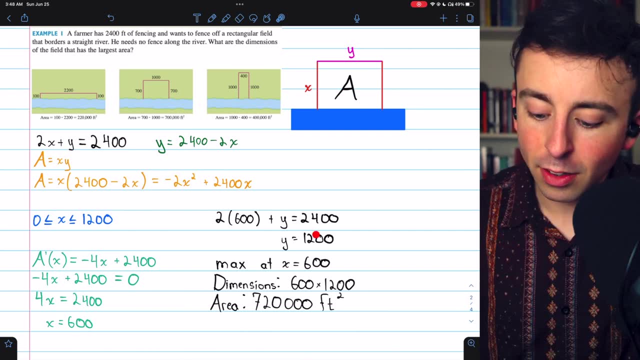 equals 600, we know that y must equal 1200,. just by plugging 600 into this equation, That would give us that 1200 plus y is 2400, so y is 1200.. Thus we have a maximum at x equals 600, the 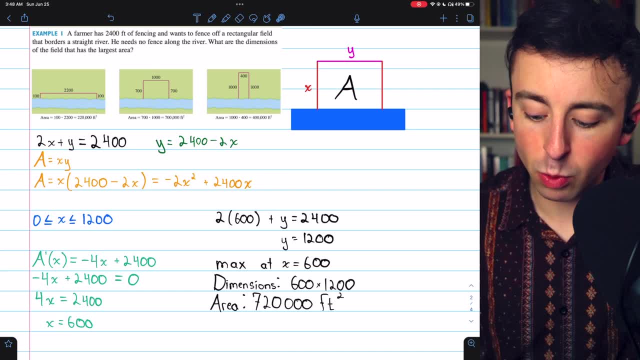 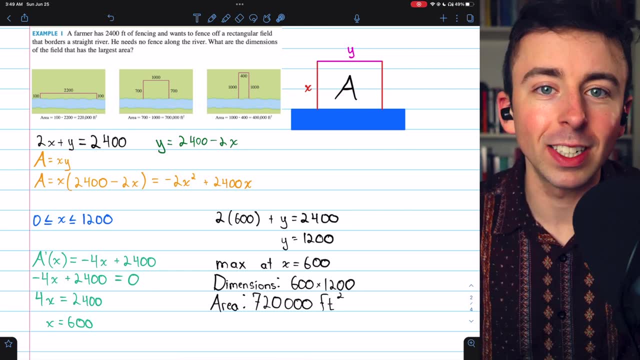 dimensions of the area function and we have a maximum at x equals 600,. the dimensions of the region that we need are 600 by 1200, and the area that we get is 720,000 square feet. That's the maximum area this region can have, given that we only have 2400 feet of fencing. 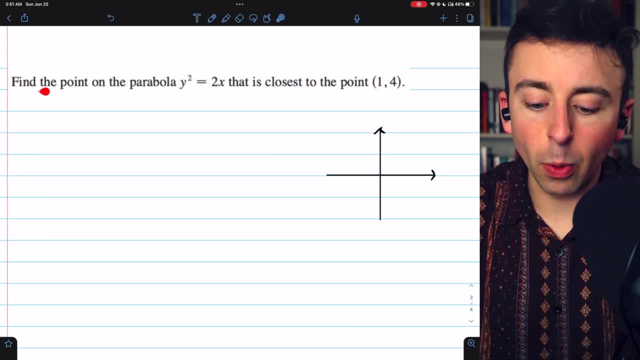 Now on to the final and most difficult problem. We want to find the point on the parabola y squared equals 2x, that's closest to the point 1, 4.. So we're trying to minimize distance closest right. We're minimizing distance. Let's begin with a sketch. Here's the xy plane. 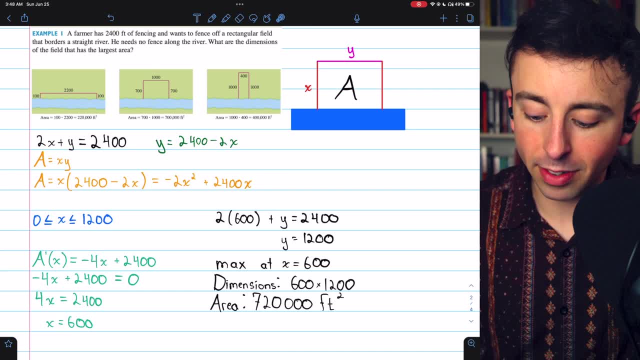 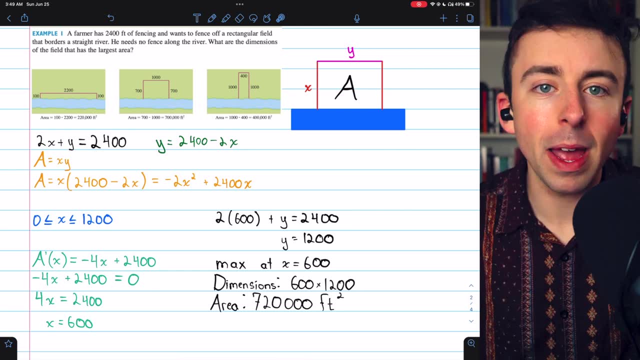 600.. The dimensions of the region that we need are 600 by 1,200, and the area that we get is 720,000 square feet. That's the maximum area this region can have, given that we only have 2,400. 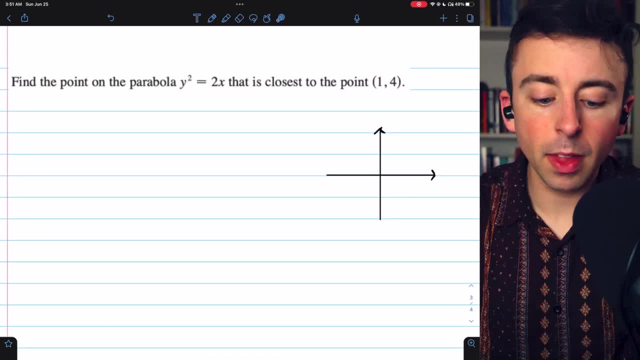 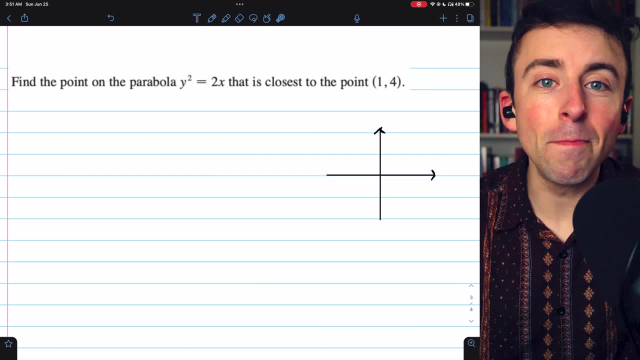 feet of fencing. Now on to the final and most difficult problem. We want to find the point on the parabola y squared equals 2x that's closest to the point on the parabola y squared equals 2x. So we're trying to minimize distance. Closest right We're minimizing distance. Let's begin with. 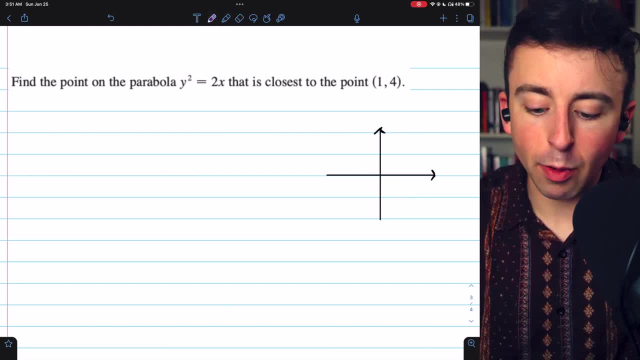 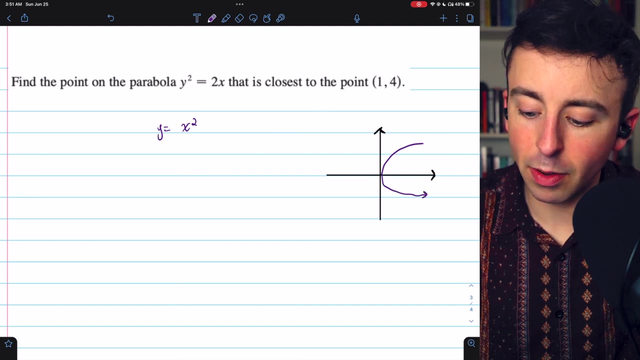 a sketch. Here's the xy plane and we want to graph: y squared equals 2x. y squared equals 2x looks a lot like y equals x squared, except instead of opening along the y-axis, it opens along the x-axis. The specifics of the sketch aren't too important, And let's say the point. 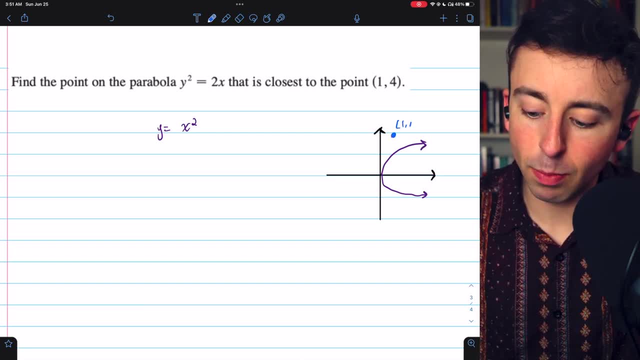 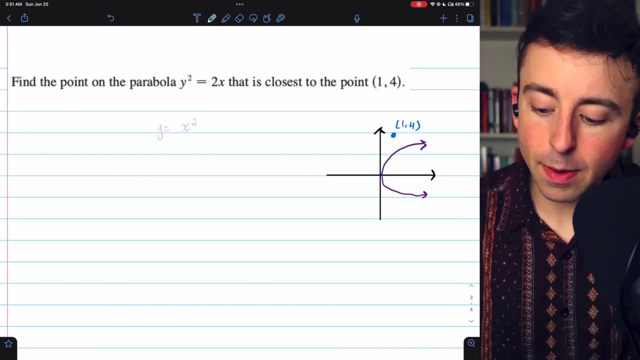 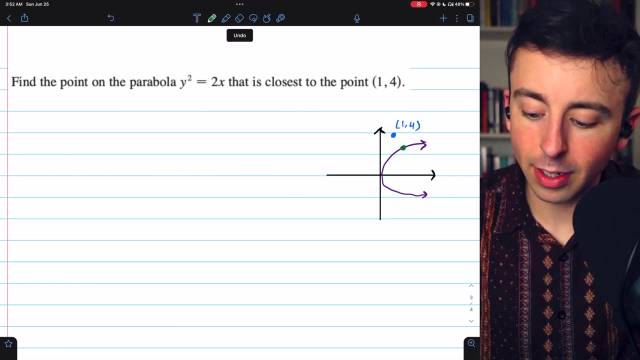 is right here and we're trying to minimize the distance between the parabola and this point. Or rather, we're trying to find the point on the parabola with minimum distance. Any point on this parabola has some distance from the point. we're trying to find which point is closest. 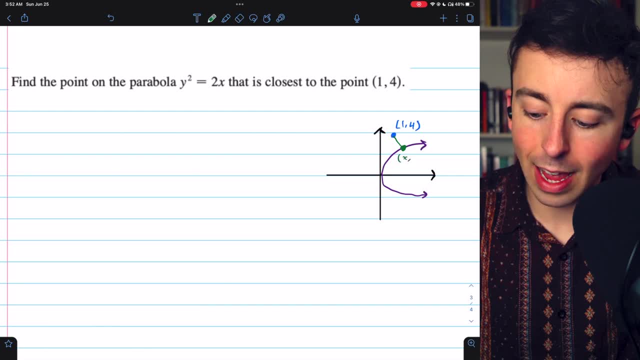 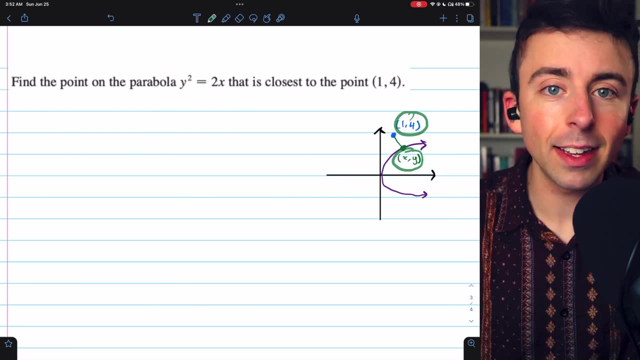 So let's just sketch a point on the parabola, say it has coordinates, The distance between a point on the parabola, and is what we're trying to minimize. We'd also want our secondary equation, if there was one. There is one, but it's already written for us. 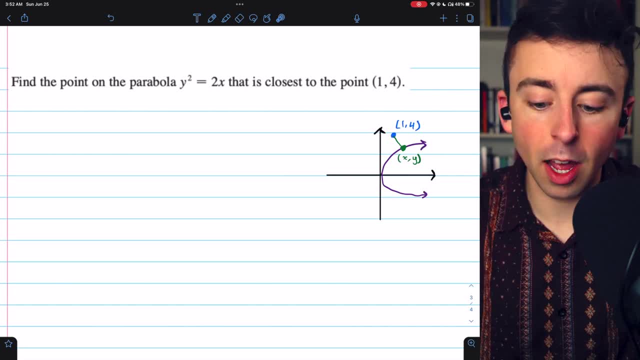 y squared equals 2x. That relates x and y and that's going to come in handy for writing our primary equation, which is the equation for distance. This is the distance between any point on this parabola and the point. It's the familiar distance formula. 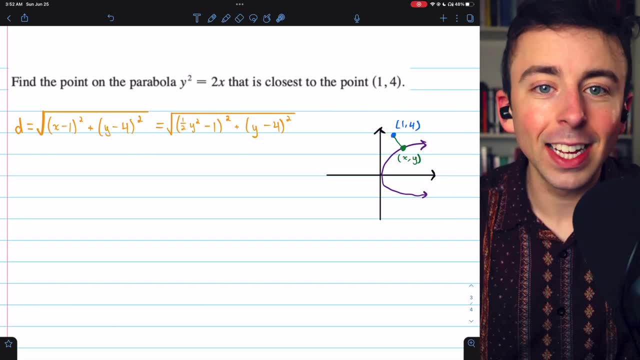 We have the square root of x minus 1 squared, that's the difference in the x coordinates squared. That's y minus 4 squared, the difference in the y coordinates squared. Again, this is just the distance between an arbitrary point on the parabola and the point. 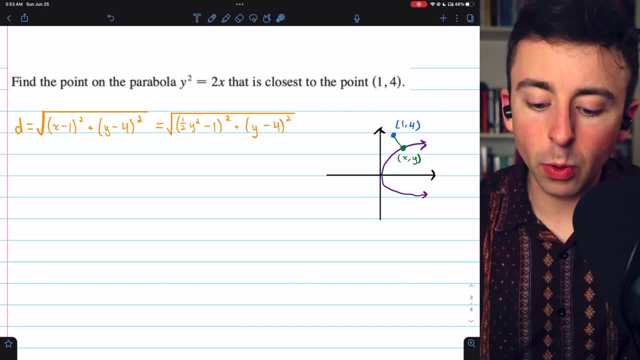 To put this equation in terms of a single variable. well, we know that y squared equals 2x, which means x equals 1 half y squared. So where we had x, we'll just put 1 half y squared, giving us this equation for distance in terms of a single variable. We could move. 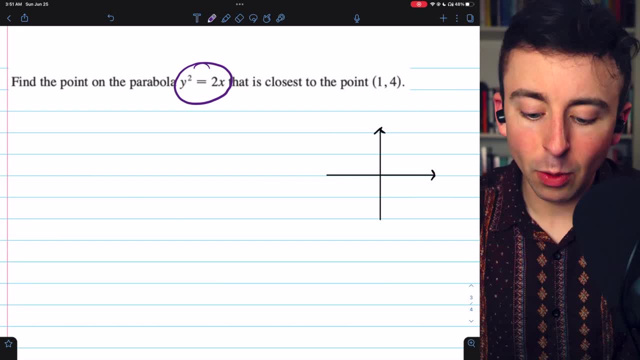 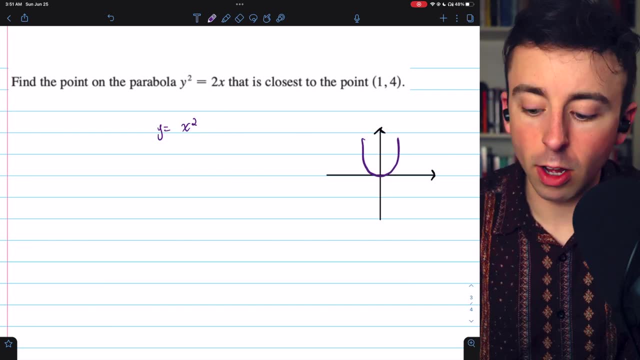 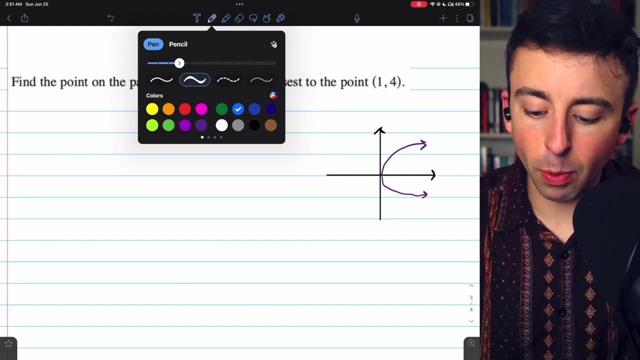 and we want to graph: y squared equals 2x. Y squared equals 2x looks a lot like y equals x squared, except instead of opening along the y-axis, it opens along the x-axis. The specifics of the sketch aren't too important And let's say the point 1,. 4 is maybe right here and we're 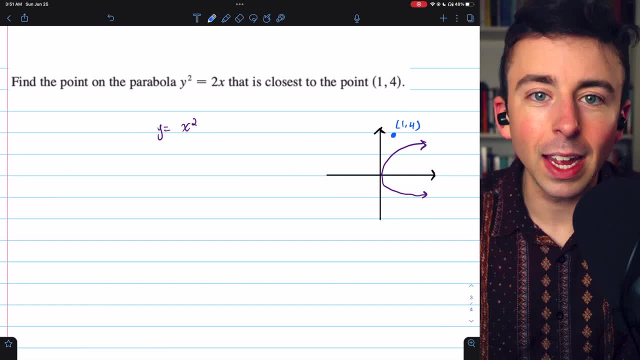 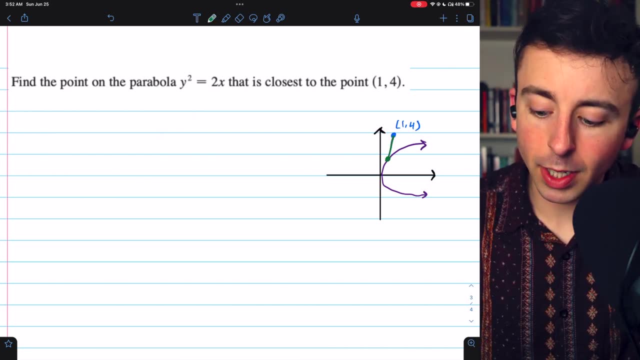 trying to minimize the distance between the parabola and this point, or rather, we're trying to find the point on the parabola with minimum distance. Any point on this parabola has some distance from the point 1, 4.. We're trying to find which. 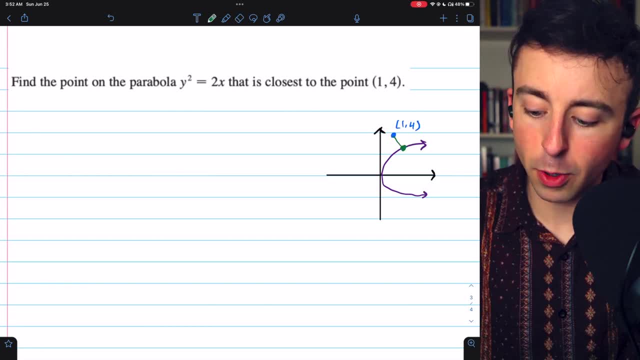 point is closest. So let's just sketch a point on the parabola. Say it has coordinates x- y. The distance between a point x, y on the parabola and 1, 4 is what we're trying to minimize. We'd 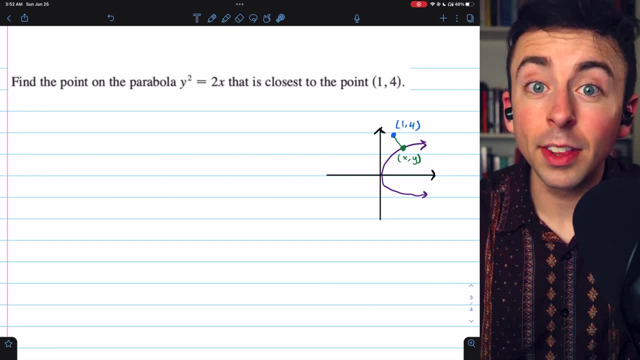 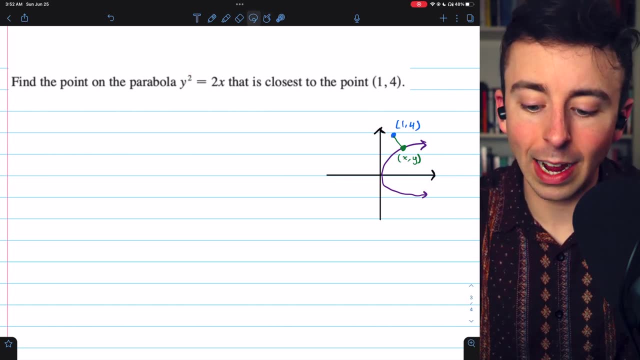 also want to write our secondary equation, if there was one. There is one, but it's already written for us. Y squared equals 2x. That relates x and y, and that's going to come in handy for our secondary equation, which is the equation for distance. This is the distance between: 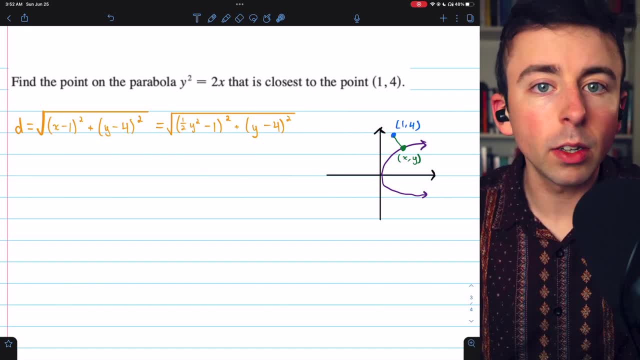 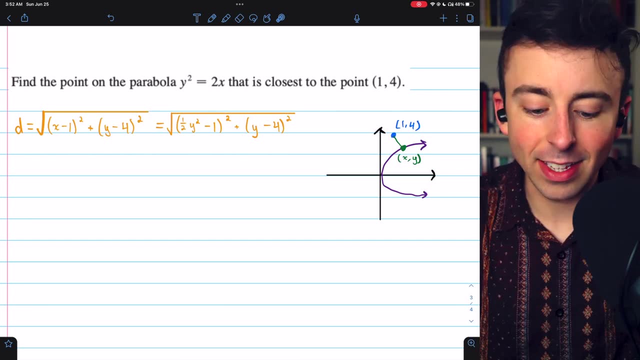 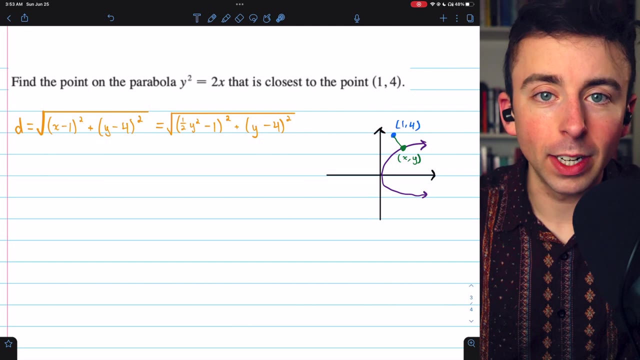 any point: x, y on this parabola and the point 1, 4.. It's the familiar distance formula. We have the square root of x minus 1 squared. That's the difference in the x-coordinates squared, plus y minus 4 squared, the difference in the y-coordinates squared Again. this: 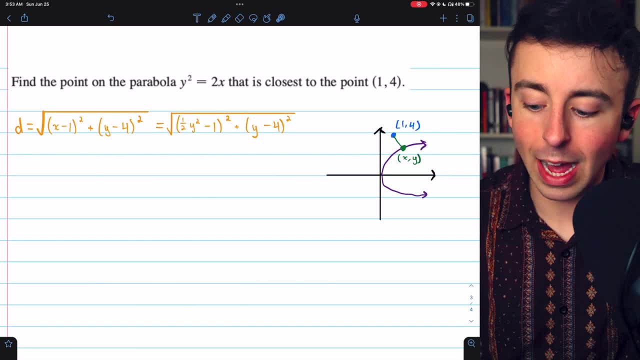 is just the distance between an arbitrary point x, y on the parabola and the point 1, 4.. To put this equation in terms of a single variable, well, we know that y squared equals 2x, which means x equals one-half y squared. So where we had x, we'll just put one-half. 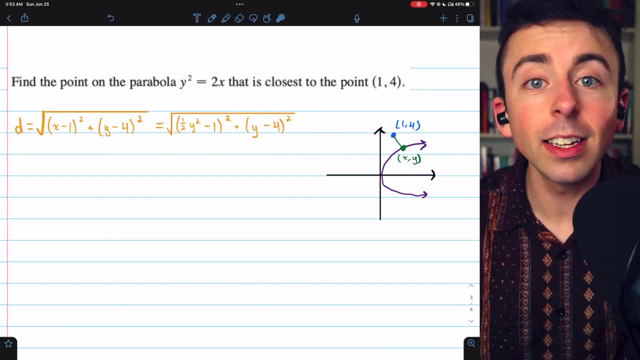 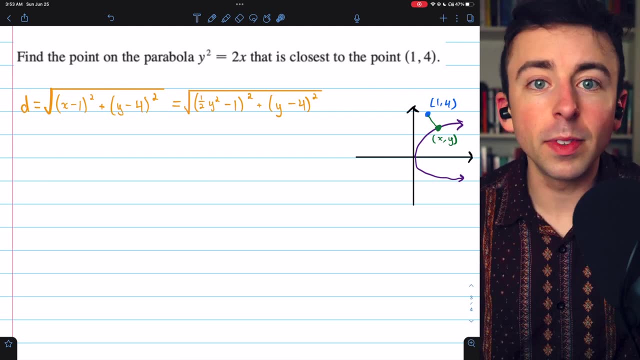 y squared, giving us this equation for distance in terms of a single variable. We could move forward using this square root function for our distance. However, the distance we know is going to be positive, right, The square root always gives a positive number And 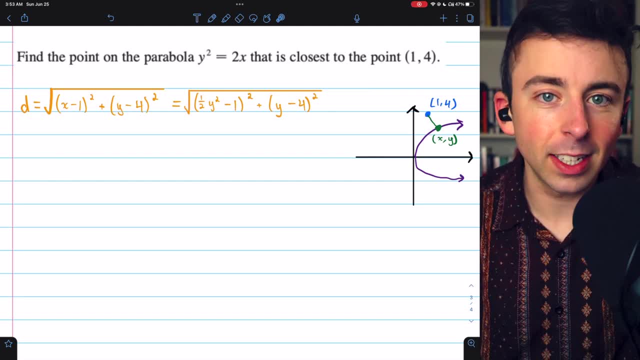 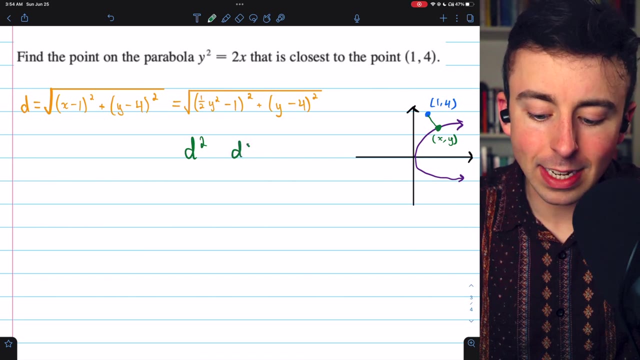 forward using this square root function for our distance. However, the distance we know is going to be positive, right? The square root always gives a positive number And x squared, or we could say d squared in this case, is increasing whenever d is greater. 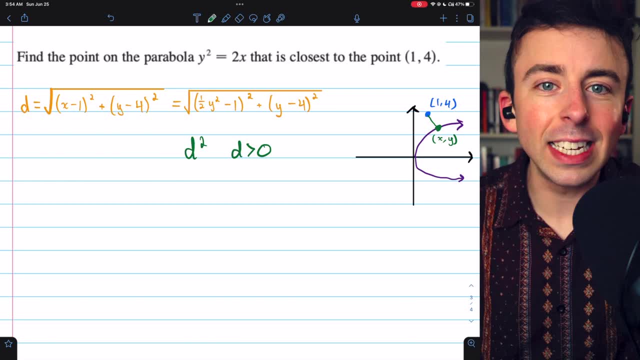 than 0,, which means wherever d squared is smallest is also where d is smallest. So the minimum of d, which is what we're looking for, will also be greater than 0.. So that's what we're looking for. We're looking for the minimum of d, which is what we're looking. 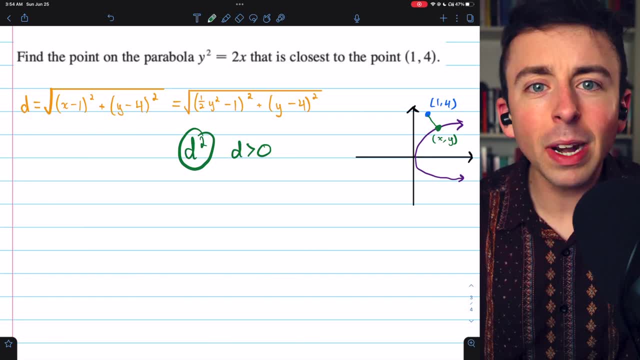 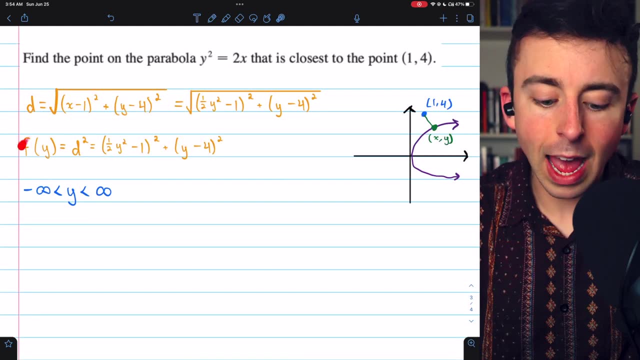 for We're looking for the minimum of d, which is what we're looking for. We're looking for the minimum of d squared. So it would actually be easier if we just worked with d squared. That way we don't have to deal with the messy square root. So we'll call our function f. 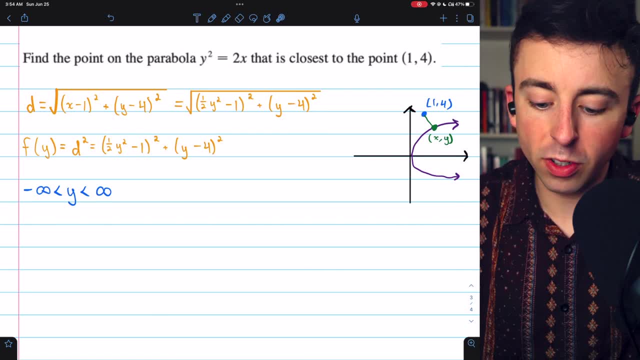 of y. What f of y is is d squared, which is just the distance function, but without that square root, because we squared it Again. the idea is that wherever d squared is minimum, that's also where d's minimum occurs. So this one will be easier for us to find, because 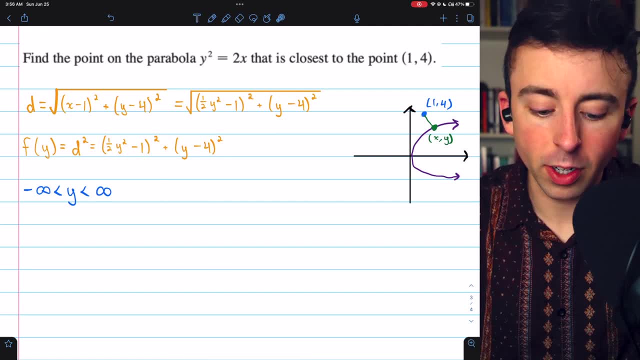 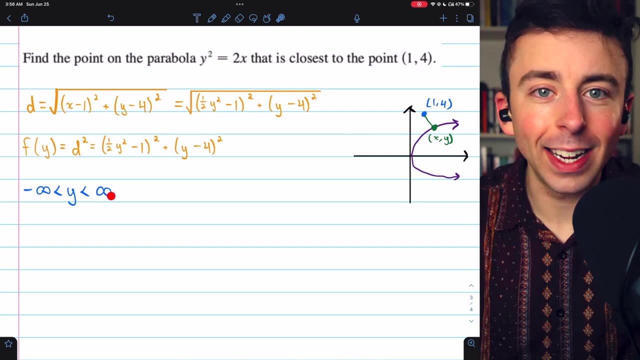 we don't have to deal with the square root. We also need to identify the domain of our function, the allowable values for y. In this case, y could be anything from negative infinity to positive infinity. This is a geometric situation, so there's no real world restrictions. 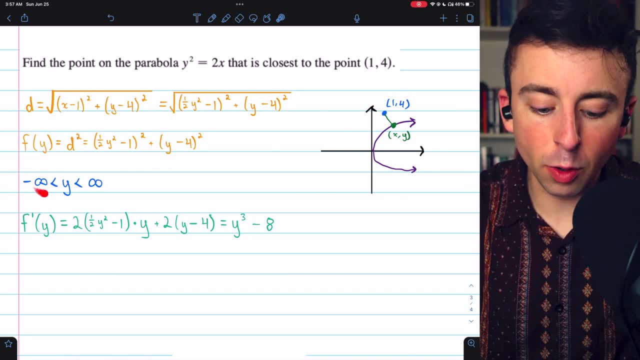 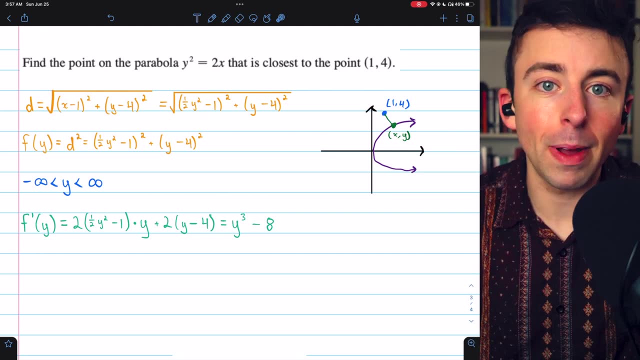 Y could be anything. Since we're not focused on a closed interval, we will have to use the first derivative test or second derivative test to classify our critical points as minimums or maximums. We, of course, are looking for a minimum, But let's get to it, We'll take. 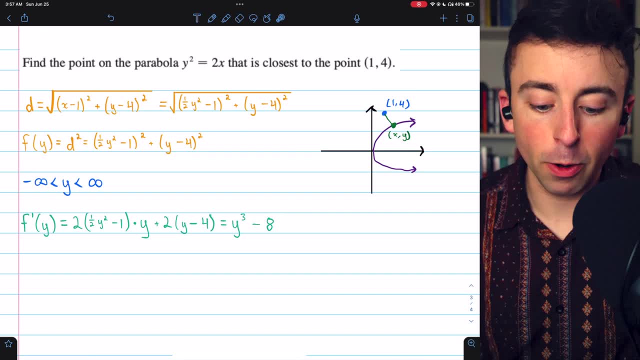 the derivative of f, of y, and then we can work out the random variable. So then we can find our critical points. To take the derivative of this, we're going to have to use the chain rule, and that gets us here. The derivative of a thing squared is just two times that thing. but then we 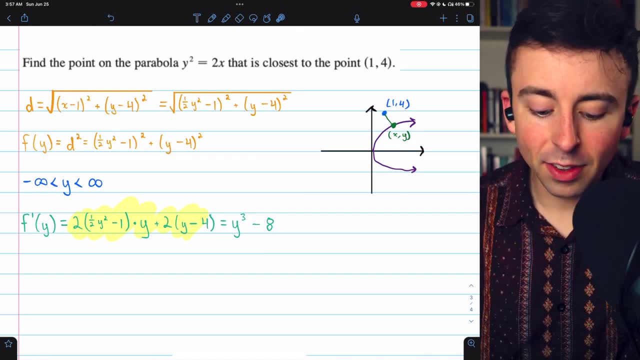 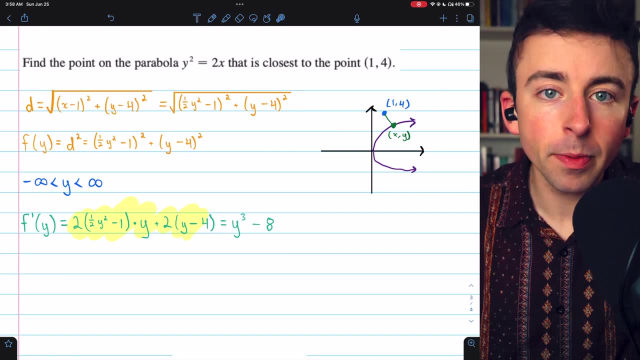 need to multiply by the derivative of the inside function. The derivative of one half y squared is just y. Then the derivative of y minus four squared is similar. The derivative of a thing squared is two times the thing. Multiply by the derivative of the inside function. In this case, 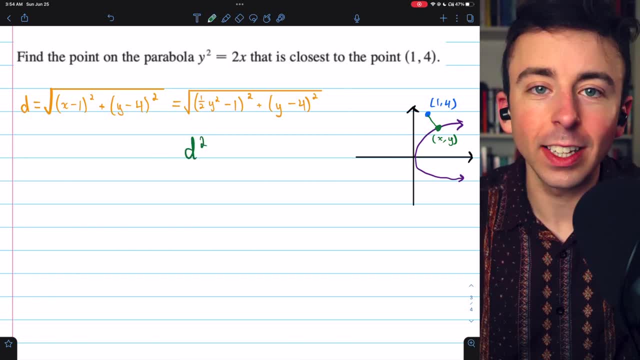 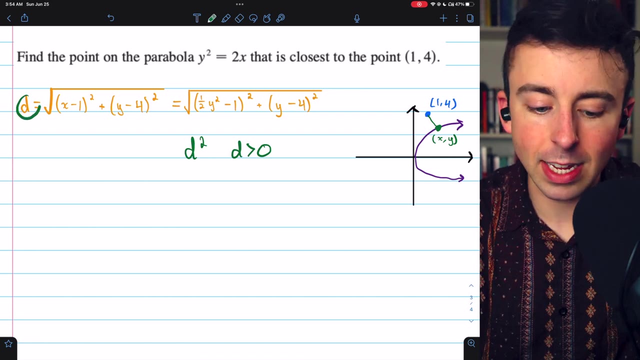 x squared, or we could say d squared in this case is increasing whenever d is greater than zero, which means wherever d squared is smallest is also where d is smallest. So the minimum of d, which is what we're looking for, will also be the minimum of d squared. 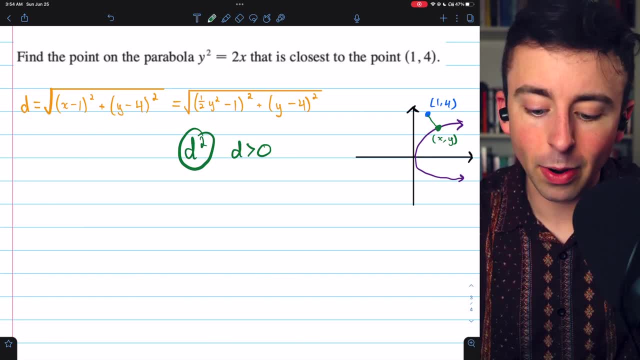 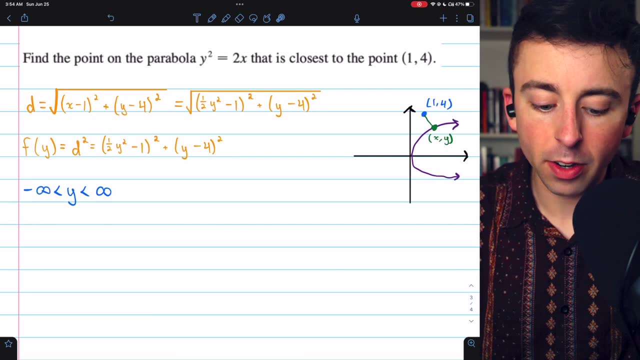 So it'd actually be easier if we just worked with d squared. That way we don't have to deal with the messy square root. So we'll call our function f of y. What f of y is is d squared, which is just the distance function, but without that square. 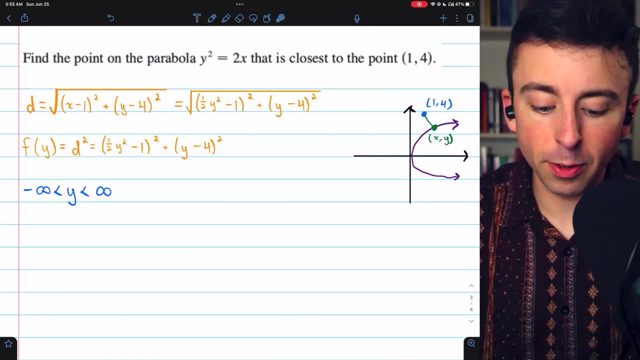 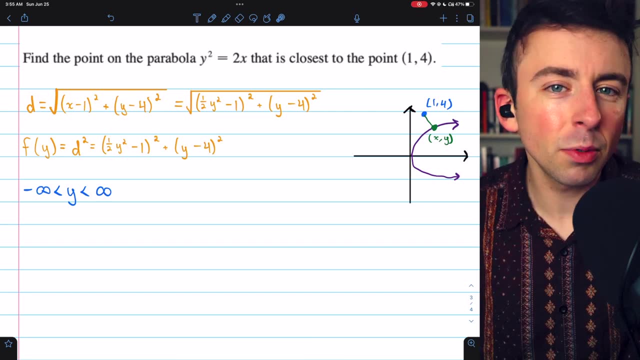 root because we squared it Again. the idea is that wherever d squared is minimum, that's also where d's minimum occurs, So this one will be easier for us to find because we don't have to deal with the square root. We also need to identify the domain of our function, the allowable values for y In this. 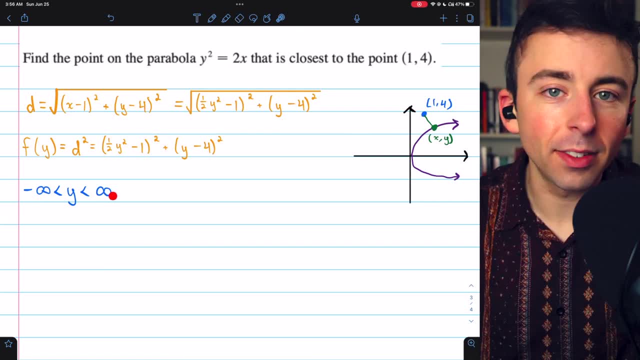 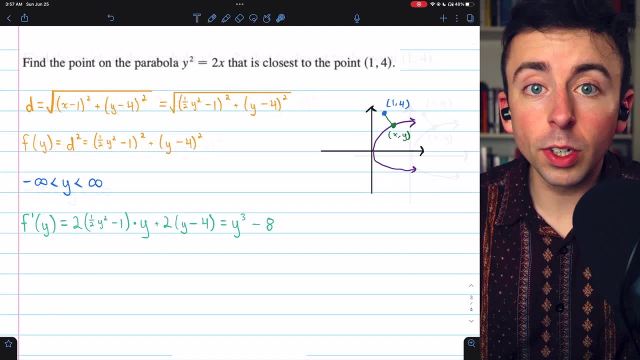 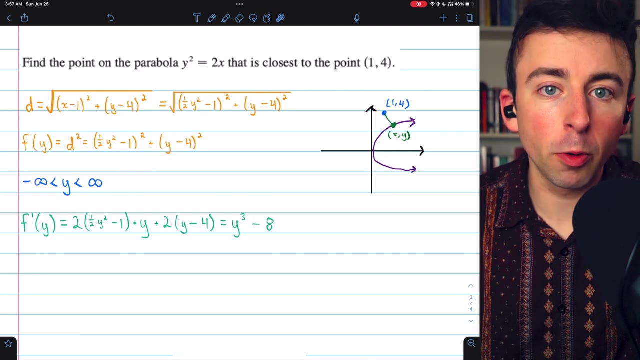 case, y could be anything from negative infinity to positive infinity. This is a geometric situation. There's no real-world restrictions. Y could be anything. Since we're not focused on a closed interval, we will have to use the first derivative test or second derivative test to classify our critical points as minimums or maximums. We 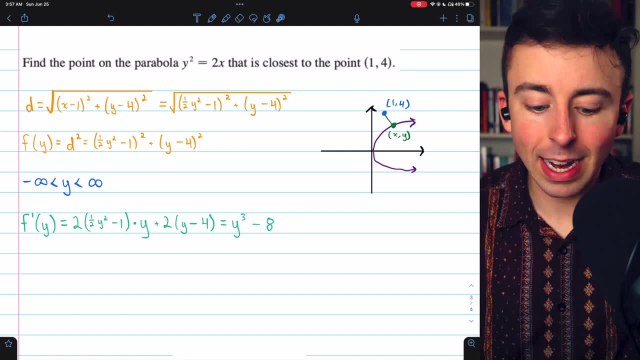 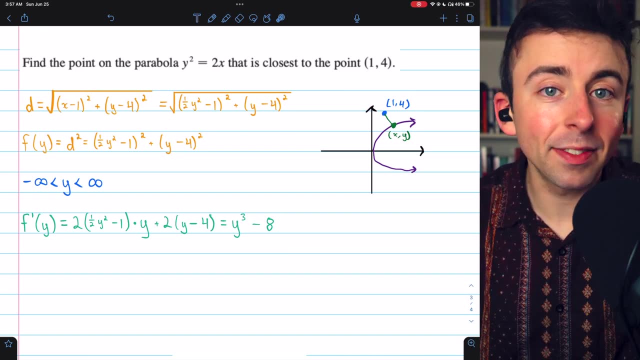 of course, are looking for a minimum, But let's get to it. We'll take the derivative of f, of y, and then we can find our critical points. To take the derivative of this, we're gonna have to use the chain rule, And that gets us here. The derivative of a thing squared. 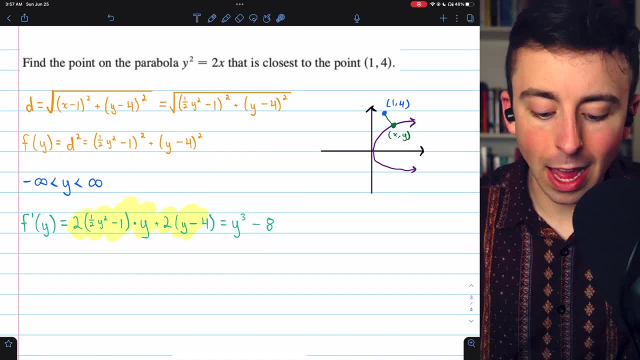 is just two times that thing. but then we need to multiply by the derivative of the inside function. The derivative of one-half y squared is just y. Then the derivative of y minus four squared is similar. The derivative of a thing squared is two times the thing. 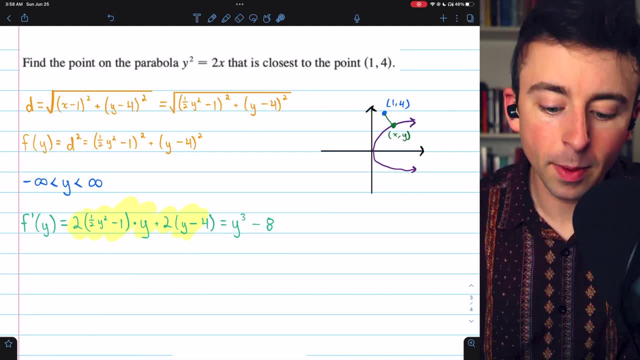 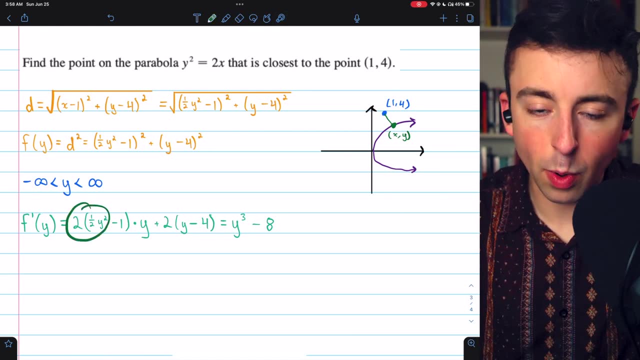 multiplied by the derivative of the inside function. in this case that's just one. Now if we simplify this, we end up getting y cubed minus eight. That's because two times a half y squared is y squared multiplied by one-third. So this part j squared is divided from y. 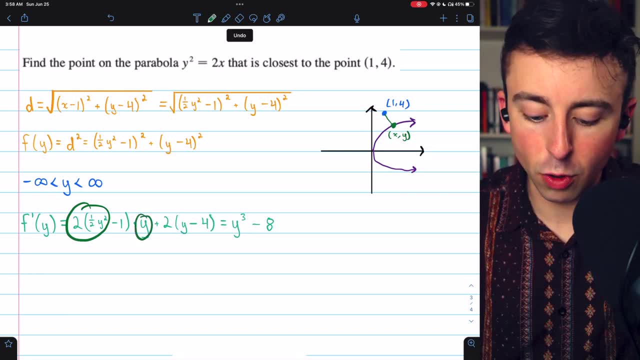 which is equal to plus j. so well, fo, or perhaps eight, reported. a real point here is that all It is a squared. So here, to be completely straight, we might have to take f of z squared. y gives us y cubed, But then 2 times negative, 1 times y is negative, 2y, which cancels out with. 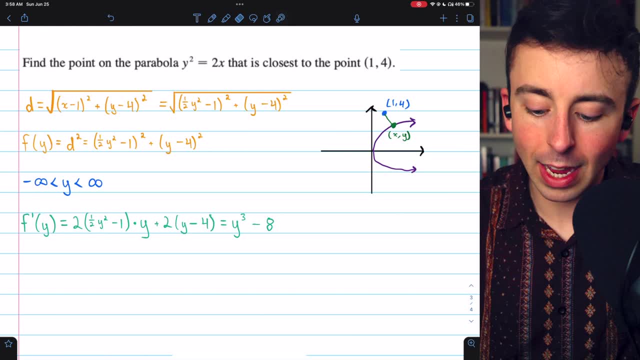 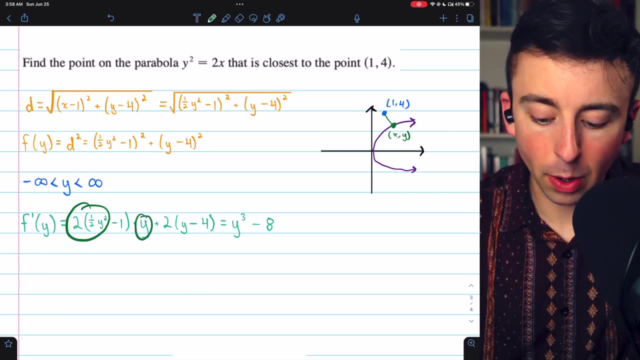 that's just one. Now, if we simplify this, we end up getting y cubed minus eight. That's because two times a half y squared is y squared Multiplied by y gives us y cubed, But then two times negative. one times y is negative, two y, which cancels out with that plus two y, But then also we have two. 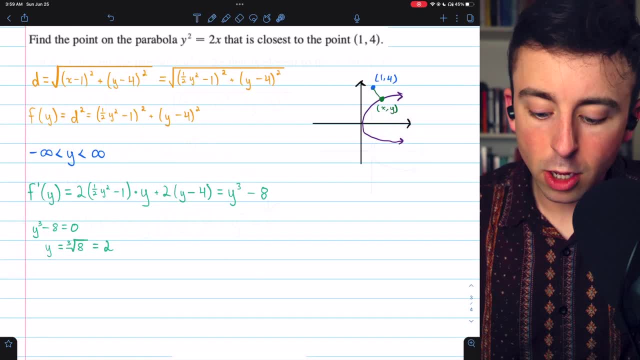 times negative four, and that's where we get the minus eight. Y cubed minus eight is defined everywhere, so the only critical points will be where this equals zero. Setting it equal to zero, we find that y equals positive two. Now, this could be a minimum. 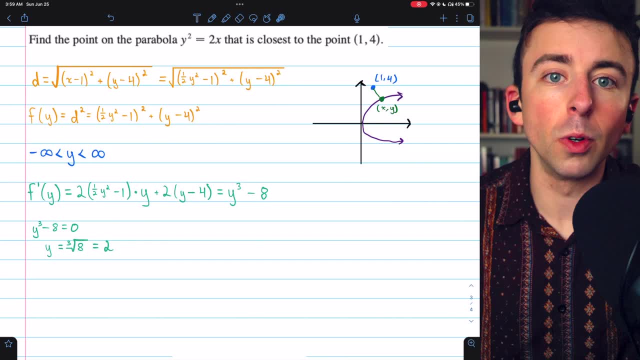 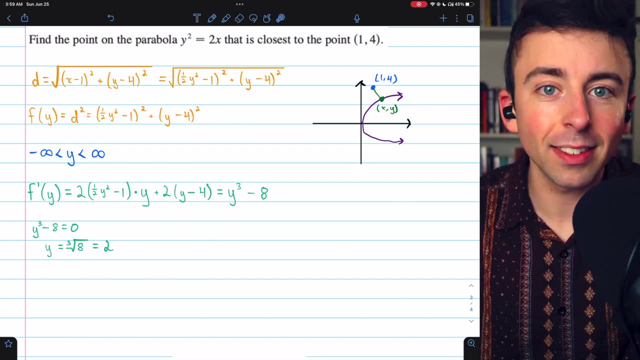 or a maximum. We don't have the extreme value theorem to apply here. We don't have a list of candidates, So we do need to classify this using the first or second derivative test. You could also just use some geometric intuition and say: hey, this parabola goes on forever. Obviously there's 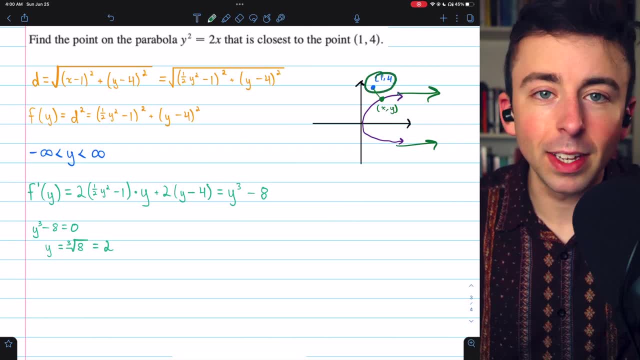 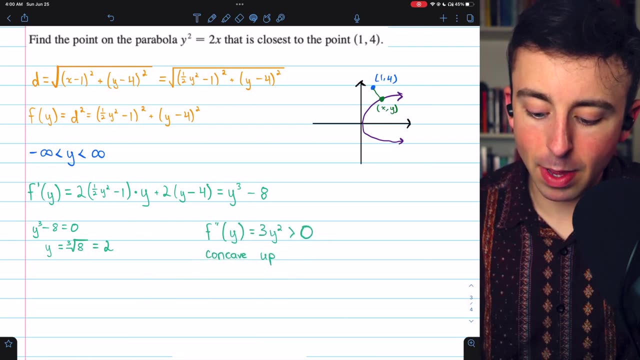 not going to be a point on it with a maximum distance from this fixed point, But let's just use calculus. The geometric intuition assures us that y equals two is a minimum and the calculus confirms it If we take the second derivative to assess the concavity. the second derivative is three. 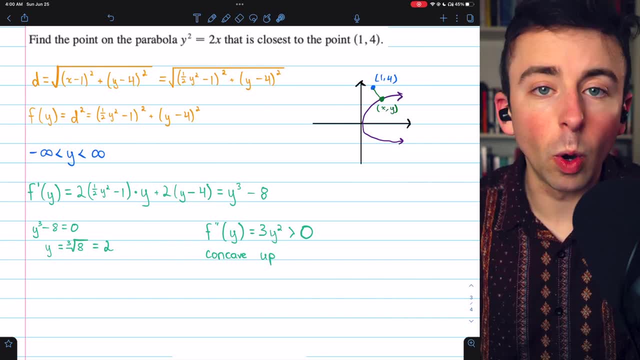 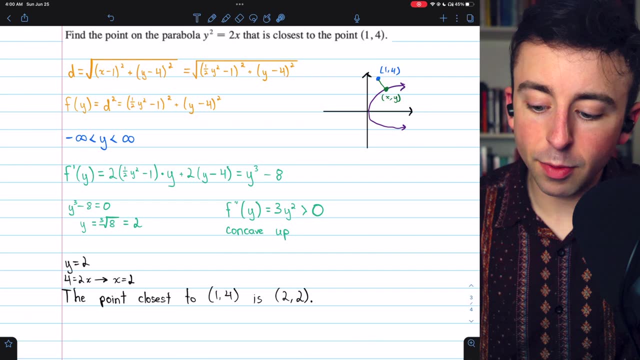 y squared, which is going to be positive, at y equals two. Thus the function is concave up, and so, indeed, we've found us a minimum. So the distance between the parabola and the point one, four is minimized when y equals two. What's the x coordinate there? 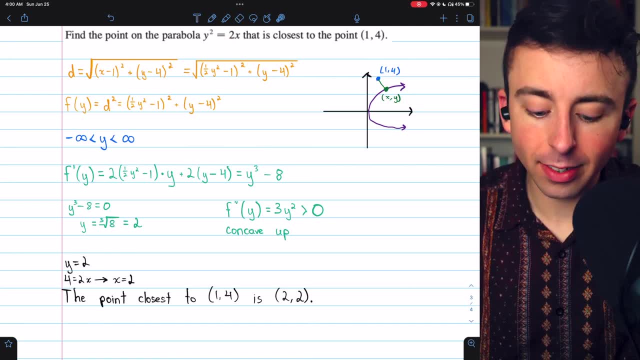 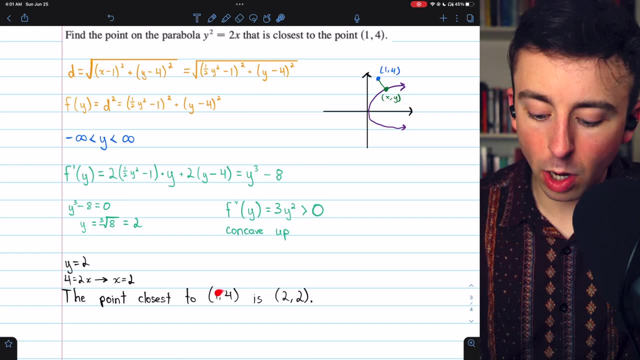 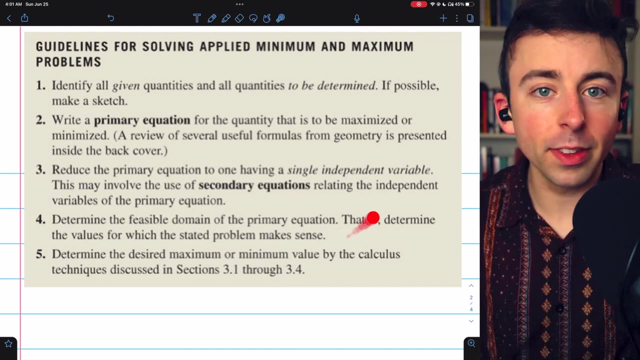 Well, since y, squared, equals two x, when y equals two, x is forced to be two. So the point on the parabola closest to one, four is the point two, two. And that's how you use calculus to solve optimization problems. Again, here are the steps. The first step is to identify the given quantities. 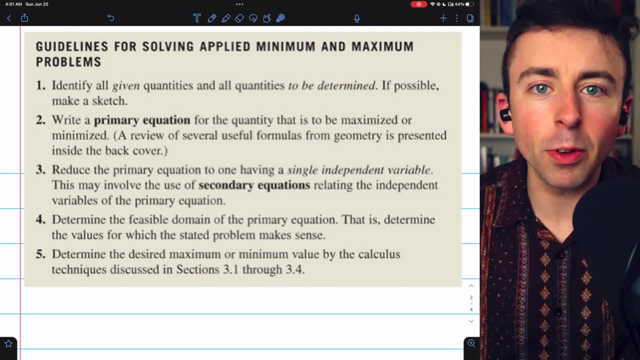 and the quantities you want to find out. Make a sketch, if you can, and write those secondary equations. Step two is to write a primary equation for the quantity you're trying to optimize. Step three is to write a primary equation for the quantity you're trying to 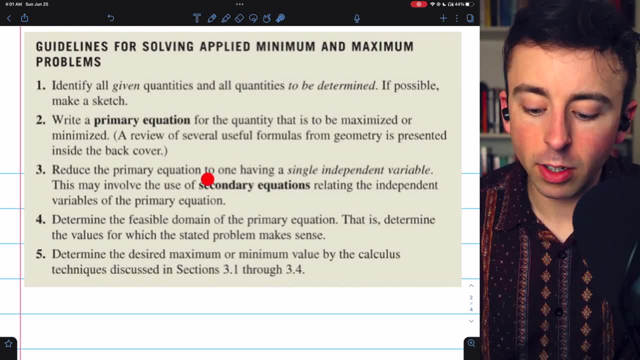 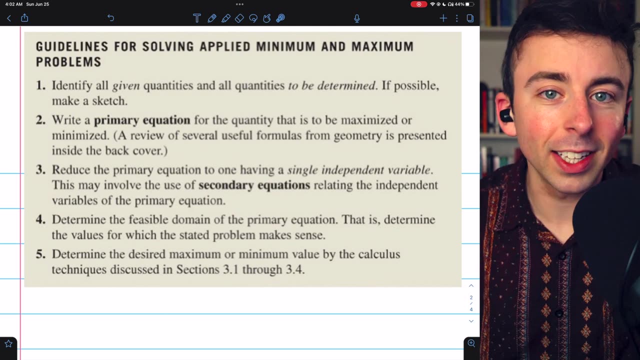 optimize. Step three is to reduce that primary equation to one having a single independent variable. Usually we have to do this using the secondary equations. Step four is to determine the feasible domain of our primary equation, And then step five is to just use calculus in order. 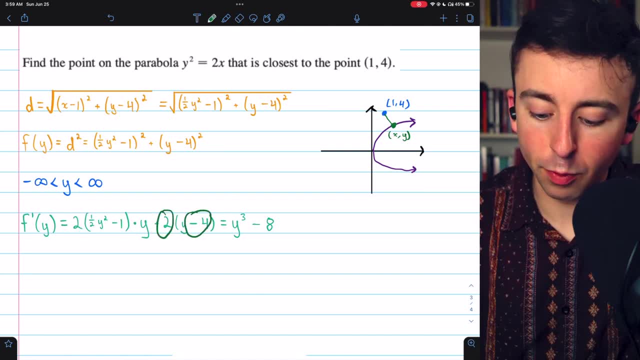 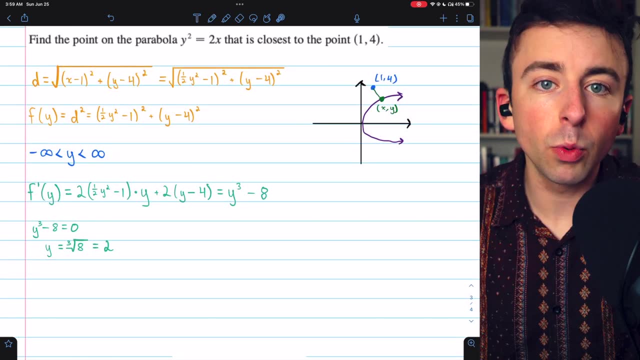 that plus 2y, But then also we have 2 times negative 4, and that's where we get the minus 8.. y cubed minus 8 is defined everywhere, so the only critical points will be where this equals 0.. 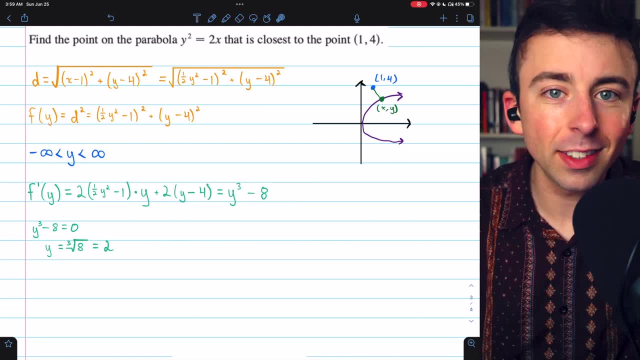 Setting it equal to 0,, we find that y equals positive 2.. Now this could be a minimum or a maximum. We don't have the extreme value theorem to apply here. We don't have a list of candidates, so we do need to classify this using the first or second derivative test. You could also just 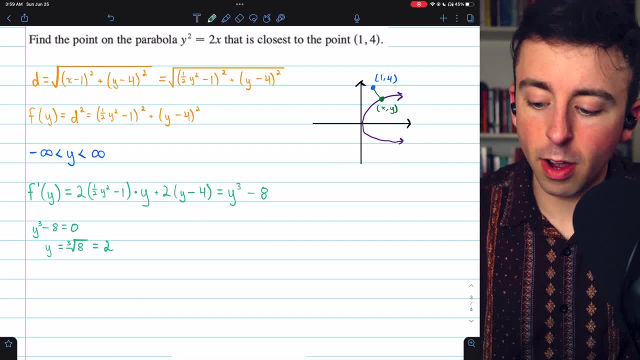 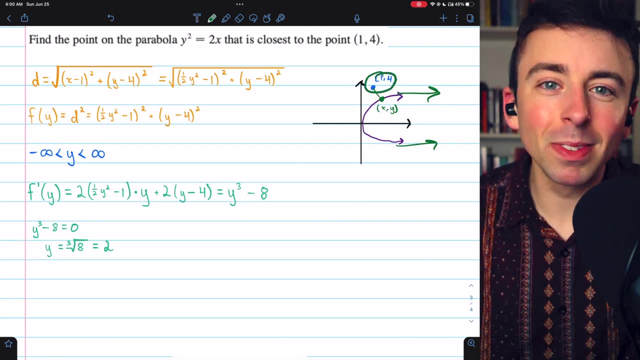 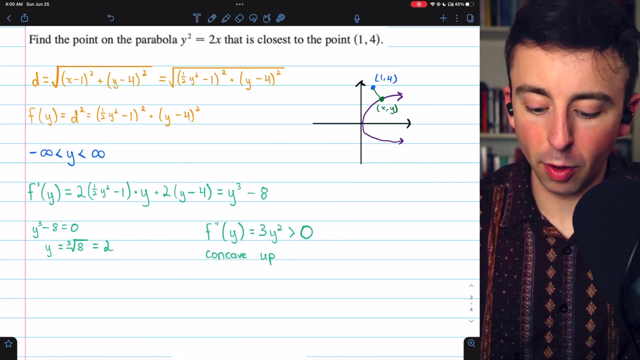 use some geometric intuition and say, hey, this parabola goes on forever. Obviously there's not going to be a point on it with a maximum distance from this fixed point, but let's just use calculus. The geometric intuition assures us that y equals 2 is a minimum, and the calculus confirms it. 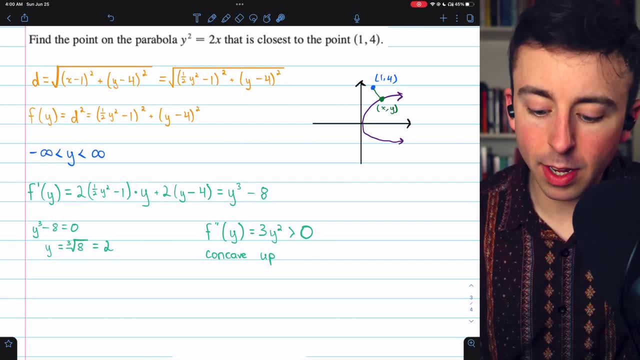 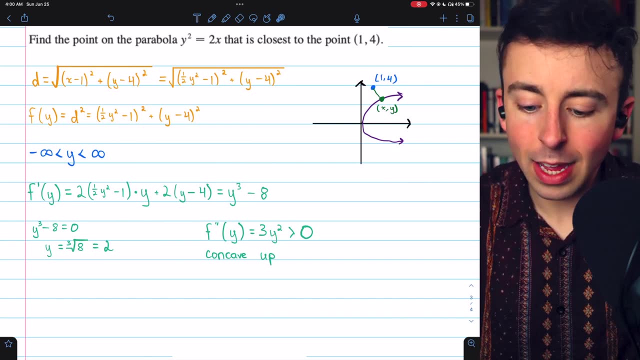 If we take the second derivative test, we find that y equals 2.. The second derivative to assess the concavity, the second derivative, is 3y squared, which is going to be positive at y equals 2.. Thus the function is concave up, and so, indeed, we've found: 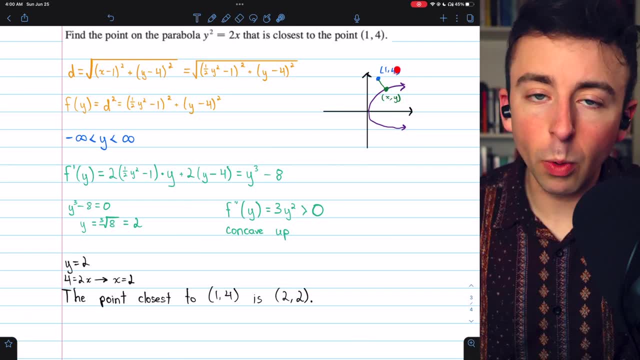 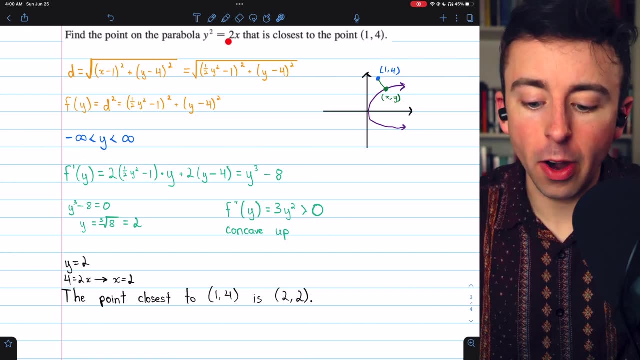 us a minimum, So the distance between the parabola and the point 1, 4 is minimized when y equals 2.. What's the x-coordinate there, though? Well, since y squared equals 2x, when y equals 2,. 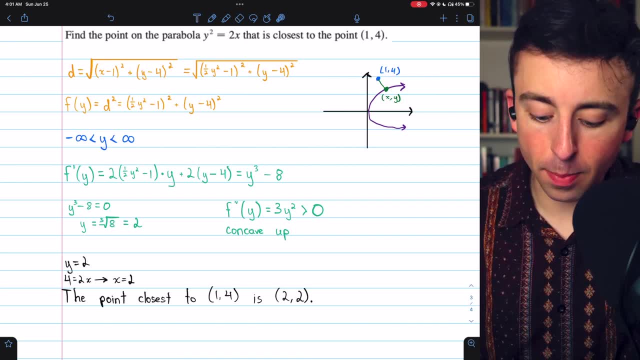 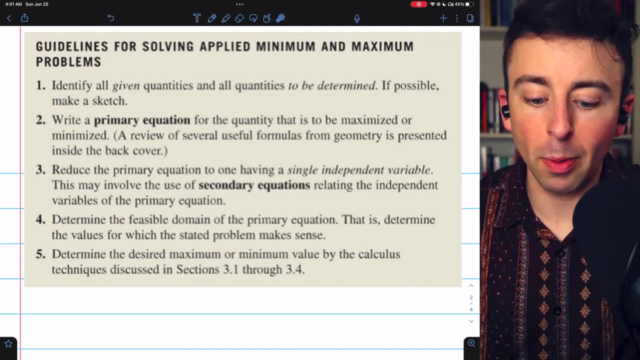 x is forced to be 2.. So the point on the parabola closest to 1, 4 is the point 2, 2.. And that's how you use calculus to solve optimization problems. Again, here are the steps. The first step is to identify the given. 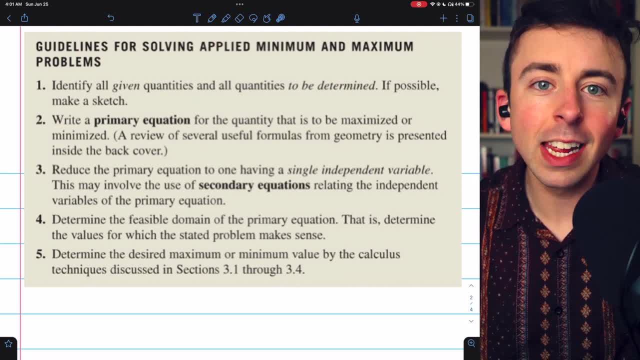 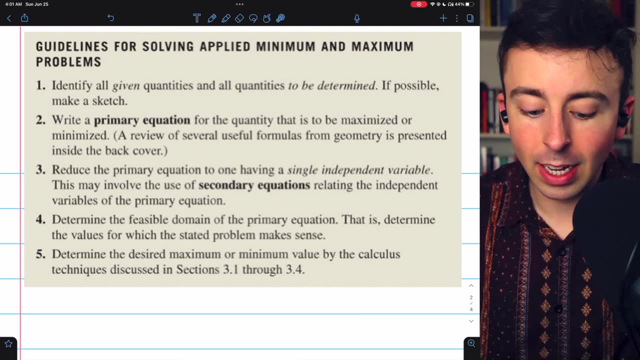 quantities and the quantities you want to find out. Make a sketch, if you can, and write those secondary equations. Step two is to write a primary equation for the quantity you're trying to optimize. Step three is to reduce that primary equation to one having a single independent. 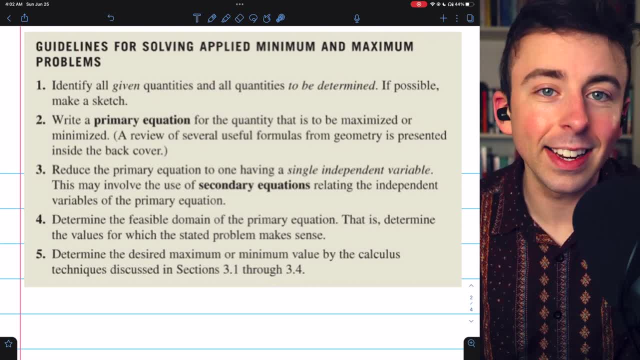 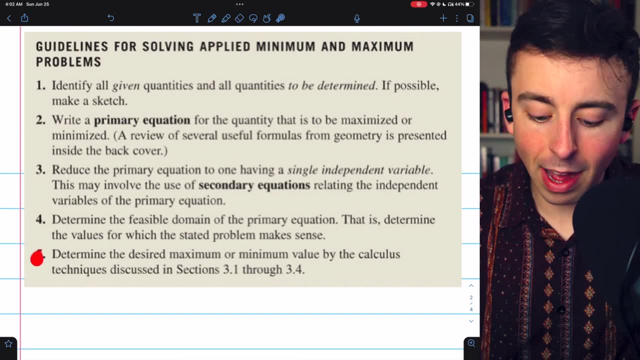 variable. Usually, we have to do that by writing a primary equation for the quantity. you're trying to do this using the secondary equations. Step four is to determine the feasible domain of our primary equation, And then step five is to just use calculus in order to find the max or the.